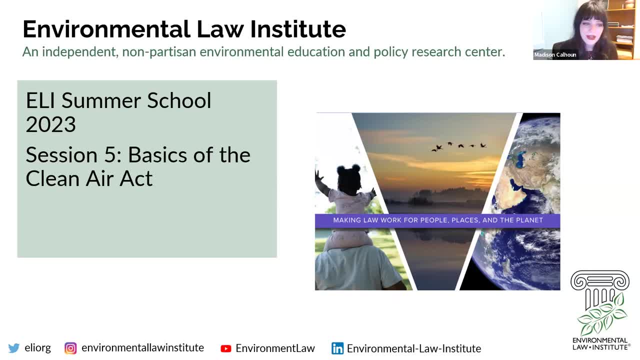 It's an introductory course into the basics and foundational elements of environmental law. So, no matter your background, you're welcome to attend all of our sessions. We will have a session of summer school every week throughout the remainder of July from 12 pm to 2 pm Eastern same times. 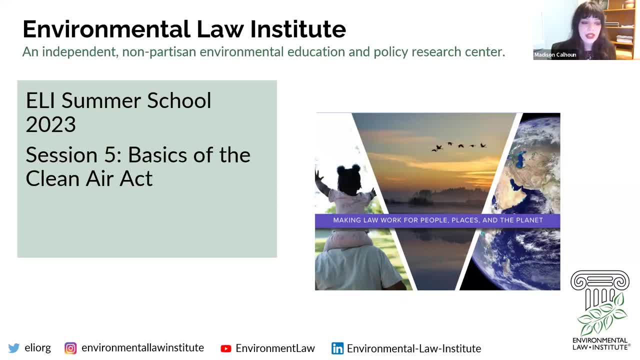 We're here right now. We will have one more session of summer school this year that will be hosted at our Washington DC office, at ELI- That's the Hazardous Waste in Sight session at the very end of July. The other sessions will only be offered via webinar. 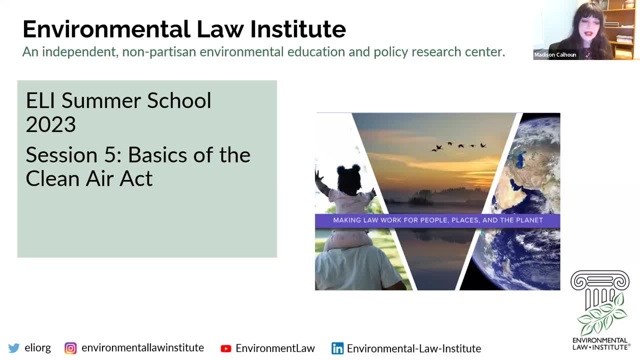 All sessions will be recorded and posted to ELI's website within a few business days of each event. If you've missed any previous sessions that took place throughout June, we encourage you to check them out now via our website. You can find each individual session on our website at ELIorg. 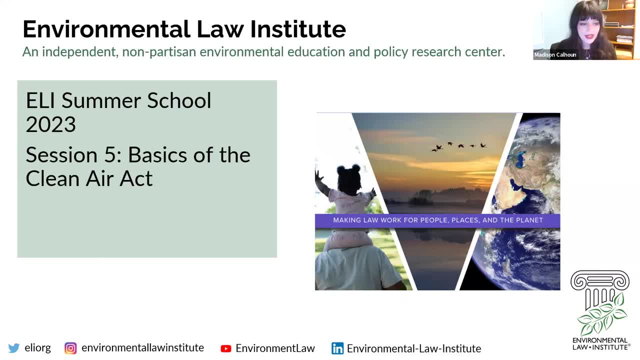 Please reach out to me or events at ELIorg with any questions. Now we'll go ahead and kick things off for today's session. Today's session, like I said, is an introduction into the basics of the Clean Air Act. In a moment I'll hand things over to our wonderful moderator. She will give some opening remarks and then our two panelists will each present. 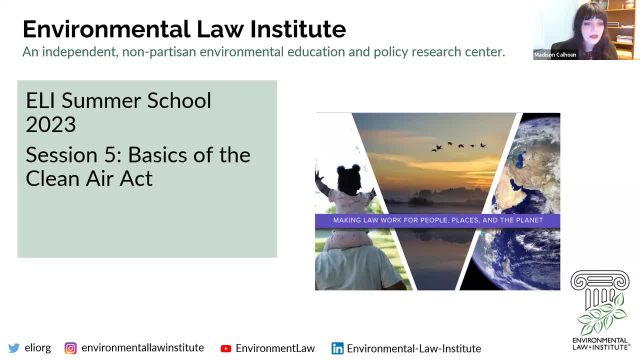 After the presentations, we'll have time for a roundtable discussion, followed by time to answer audience questions. Please feel free to submit your questions as soon as you think of them using Zoom's Q&A function. There's no need to wait until the end of the program. You can submit your questions as you think of them. 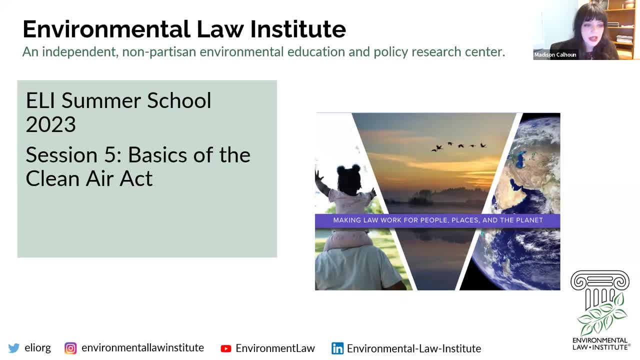 The chat function is also open. We encourage you to use the chat function to answer questions, Chat to converse with one another or to post your observations throughout the program. However, please remember to put your questions in the Q&A box, not in the chat. 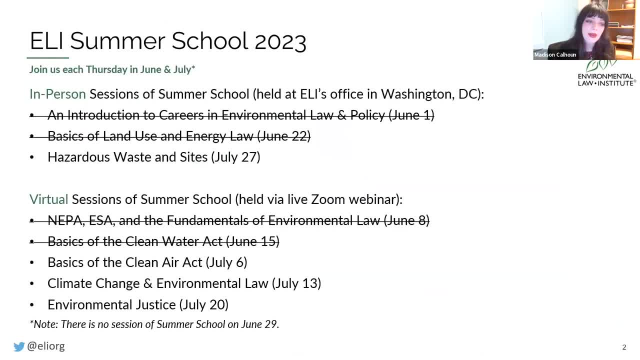 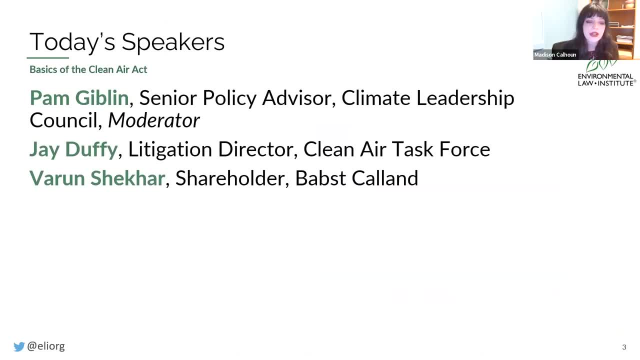 With that let's begin. I'm now going to introduce our moderator, Pam Giblin. Pam is a senior policy advisor at the Climate Leadership Council. She was previously a partner for 24 years at Baker Brotz, where she led the firm's environmental practice group. 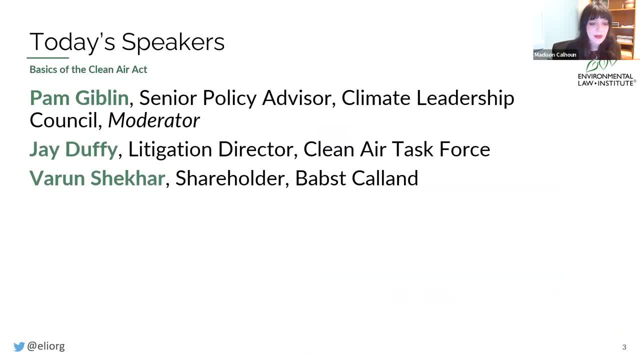 She's practiced environmental law since 1970 and has extensive experience in advising clients on a broad array of environmental issues. Pam was president of the American College of Environmental Lawyers from 2014 through 2015.. She previously served as a member of the Environmental Protection Agency's Clean Air Act Advisory Committee. 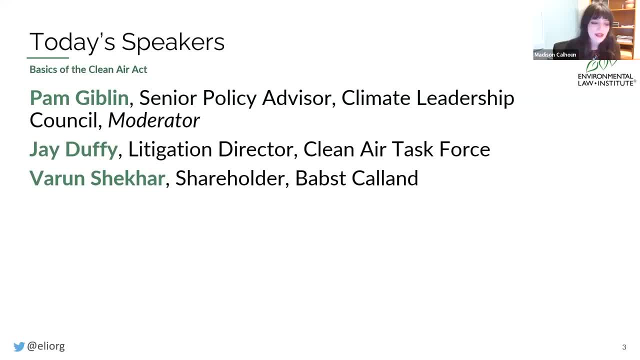 Pam has received her BA with honors from the University of Texas and her JD from the University of Texas School of Law. Pam, I'll go ahead and hand things over to you. Thank you so much, everyone. Well, I really appreciate the privilege of participating in this program, and our vision of what we want to accomplish today is to give you a. 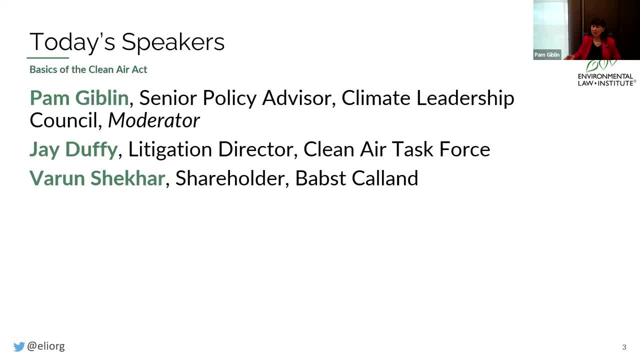 foundational grounding about the Clean Air Act, how it all hangs together, to help you understand how to solve problems under the Clean Air Act. So I always like to go back to the basics. I always told people when I was managing the environmental department at Baker Brotz: start with the statute, then move to the regulations and then finally to the policy documents. 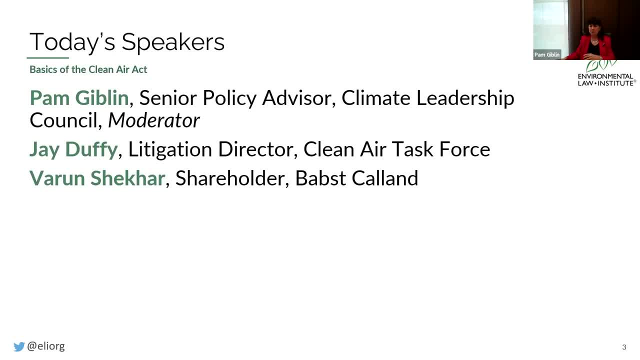 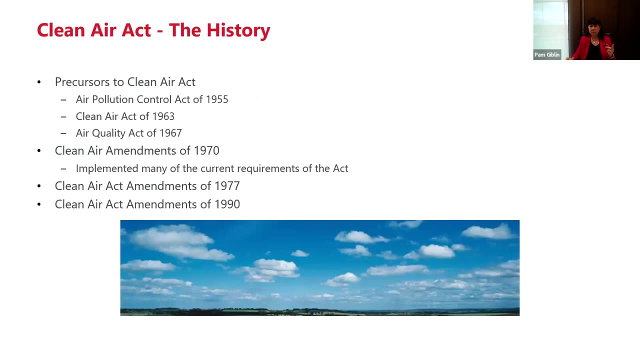 Because we had people who sometimes wanted to immediately go to the sort of the geekier documents and the statute always takes us back. If you could post the first slide, I did a very quick summary of the history of the Clean Air Act and this is important because 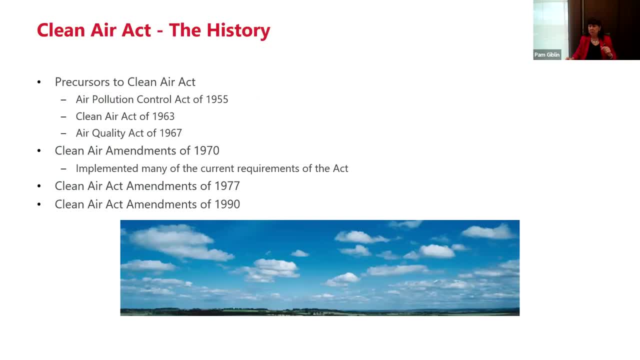 the Clean Air Act basically started in 1970. That was the iteration that created EPA and implemented many of the current requirements of the Act. Fascinatingly, that 1970 Act was 38 pages. It's almost like the US constitution when you read it. It's very elegantly worded and gives very basic direction to EPA. 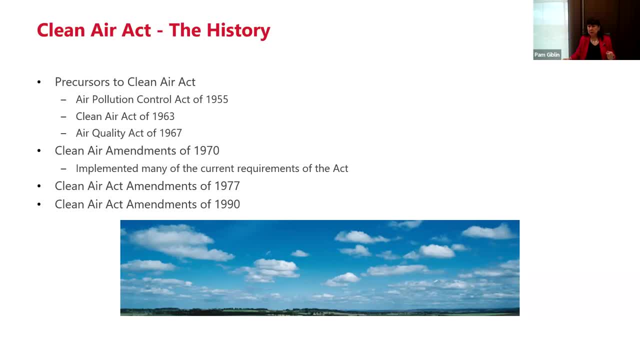 Among the things that it mandated that EPA do, which is sort of the anchor of the Clean Air Act, was to establish National Ambient Air Quality Standards, And later Maroon is going to talk in greater detail about that, But again, it was a. 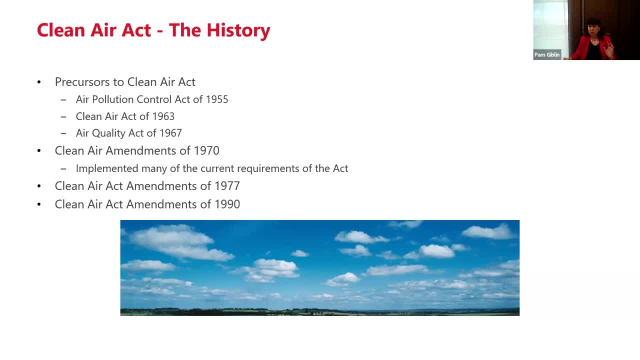 It was an exquisitely elegant statute short and created the true north of the Clean Air Act, which was that certain health-based standards had to be attained, those national ambient air quality standards. And one interesting thing about the national ambient air quality standards is that since 1970, there have only been six pollutants designated as NAXAs national ambient air quality standards, which is fascinating. 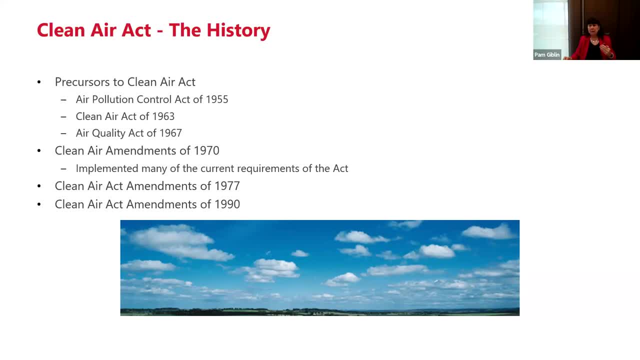 There has been discussion that if greenhouse gases are to be regulated under the Clean Air Act in more force, that perhaps there should be a NAX, a national ambient air quality standard for CO2 or any of the other greenhouse gases. But so far we've had six. six since 1970, and six continue. 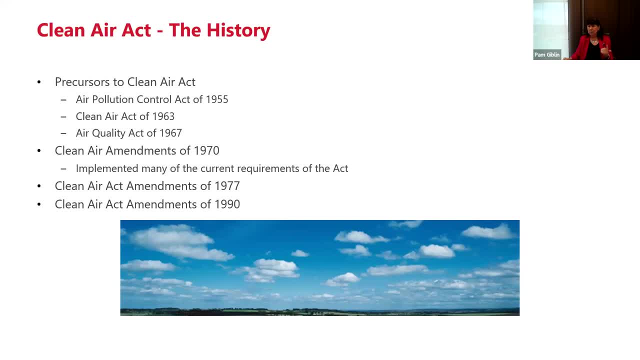 And one of them is kind of a sort of an anomaly: It's carbon monoxide, not carbon dioxide, which of course carbon monoxide is an exquisitely. It's not really sort of generally considered as an air pollutant, but it's been there since the beginning. 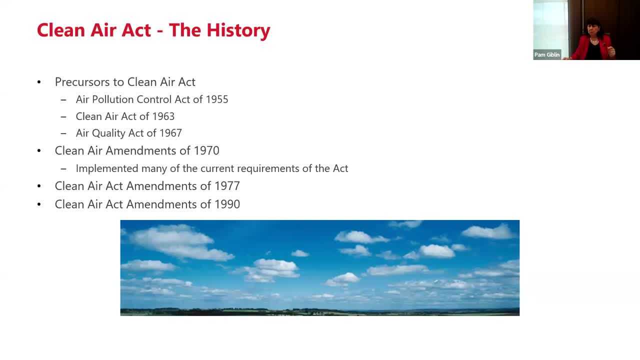 No NAXAs have been deleted. They're supposed to be revised periodically and sometimes they are. But the lead NAX, for example, was not touched for gosh like 20 years. But it's very important to remember that that's sort of the cornerstone of what was mandated in the original 1970 Clean Air Act. 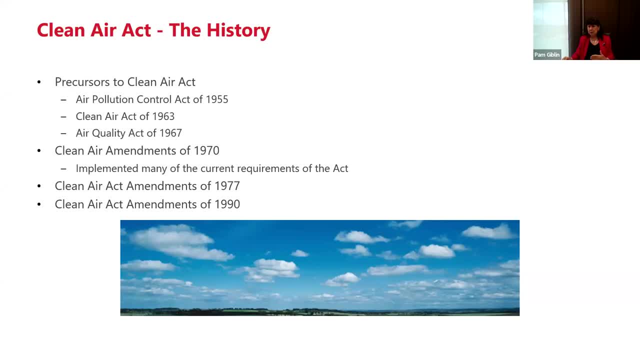 I had the privilege of working with Leon Billings, who was the author of the Clean Air Act of 1970, and he also authored the Clean Water Act. He was the chief staffer for the Senate Environment and Public Works Committee and Senator Muskie, from Maine, was the main- you know- senator in charge of that committee. 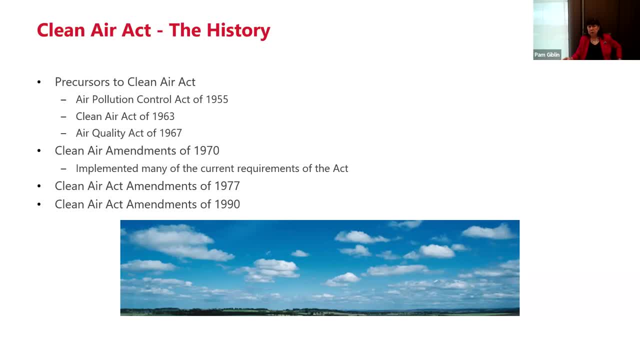 And Leon was masterful. I want to give a plug to an interview, An interview that Scott Fulton, former president of ELI, did with Leon Billings before Leon passed away, where Leon goes through the history of the Clean Air Act from the inside and you know what it took to get it enacted and what were the fundamentals that he was trying to work on. 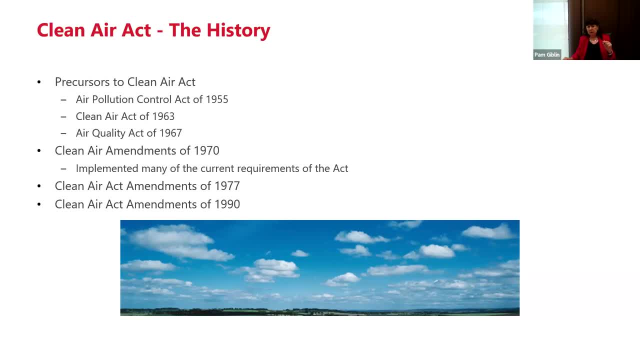 But he was marvelous- The Clean Air Act amendments of 1977, which I actually worked on because the original 1970 Act did not have preconceptions And so it set these standards and then EPA had to go enforce them after the fact that you could build something without pre-construction review. 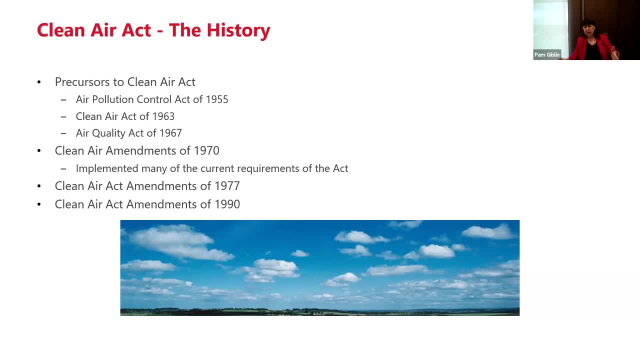 Well, just as a side point, Texas, for example, had a Clean Air Act since 1965, five years before the 70th Amendment, And in 71, Texas added a pre-construction permit requirement to their Clean Air Act, first state in the country to do this. 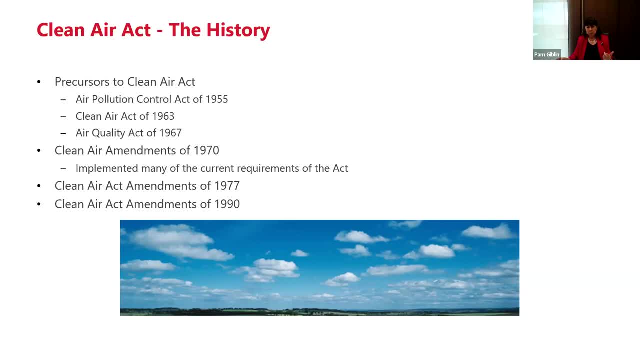 And so one day I get a call from Leon Billings who had heard about the fact that we had put this into the Texas statute and said: I want to do that to the federal statute. So I started working with him. The amendments were supposed to pass in 75, but that took another two years. 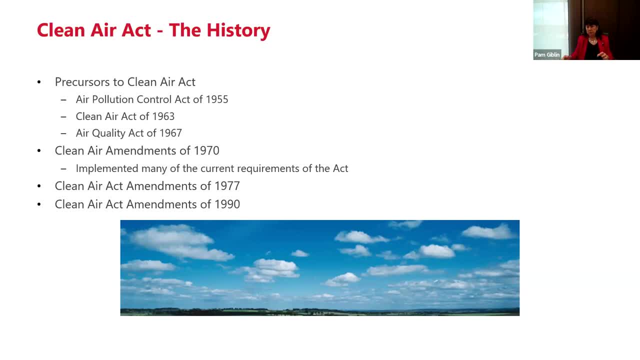 So the Clean Air Act amendments of 1977 introduced for the first time the notion of pre-construction permit, that before you could break ground on a facility you had to get approval, Approval, You had to demonstrate that you were going to meet all of the standards, not just the National Land and Air Quality standards but whatever other standards had been enacted in the meantime. 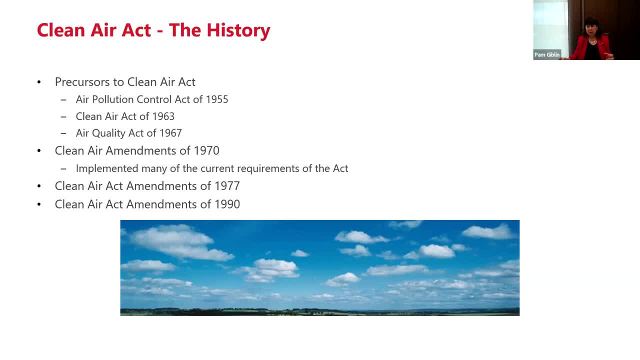 One again these little anecdotes that Leon Billings would share. Texas's permit provisions did not have any minimum below which you did not have to get authorized in advance. He thought that was a little harsh, that it was going to be difficult to sell that to Congress. 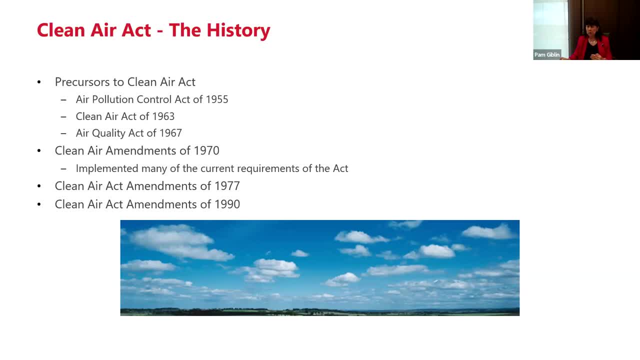 He said there has to be some threshold. He said there has to be some threshold below which you're not a major source. you don't have to get pre-construction permit approval. So he was trying to figure out where that threshold should be. 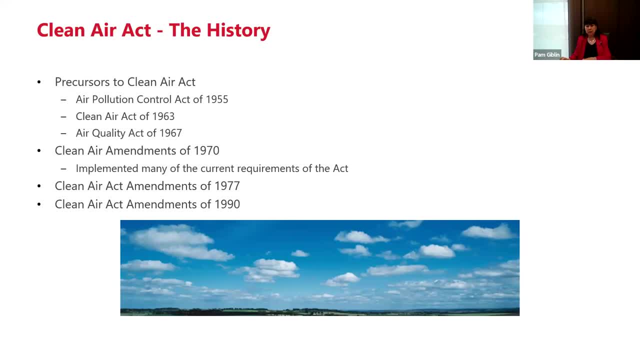 Well, Senator Muskie was, as I mentioned, from Maine. So, Leon, I was in his office and he picks up the phone and calls Myron Knudson, who some of you may have heard of. He's legendary with MEPA. 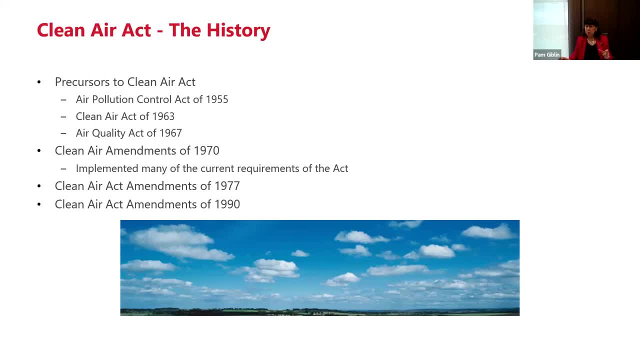 He's just recently retired, But he was head of Region 1, which included Maine. So Leon says: okay, Myron, What does the largest source emit in Maine, The largest source of air contaminants? And Myron said, gosh, maybe 50 tons. 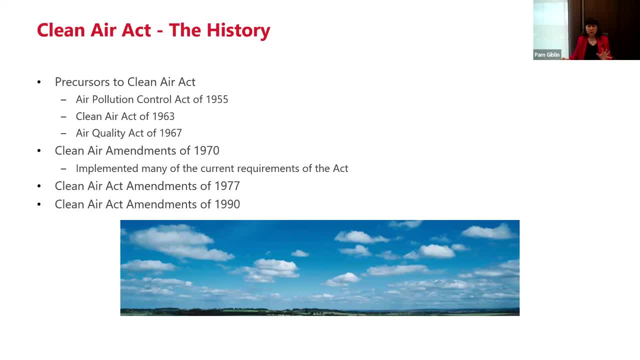 So Leon said: well, let's double it. So the 100-ton threshold that was put into the 77 amendments as the major source cutoff came from that. So it was fascinating to see how the sausage was being made. And then finally the Clean Air Act amendments of 1990.. 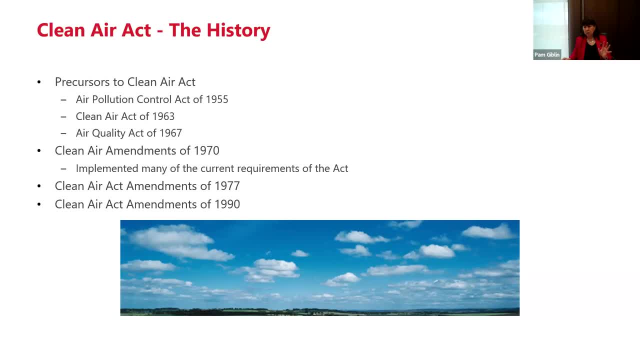 And it's significant that a statute that is as powerful as the Clean Air Act has only been amended, you know, twice since 1970. And the Clean Air Act amendments of 1990, and Jay is going to touch on a lot of what was added by that series of amendments. 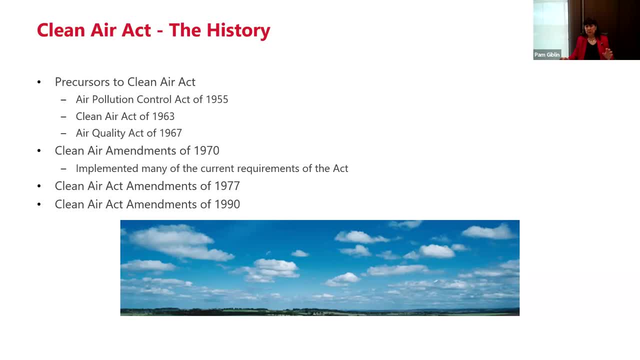 It's like it's about 900 pages of amendments, So 38-page initial statute, and it just grew and grew and grew. And the most significant, The most significant thing in the Clean Air Act amendments of 1990 was the addition of what are called Title V permits, which it sets up a process for consolidation of all the requirements that apply to a facility so that they could be codified in one place, in that one Title V permit enforceable by EPA. 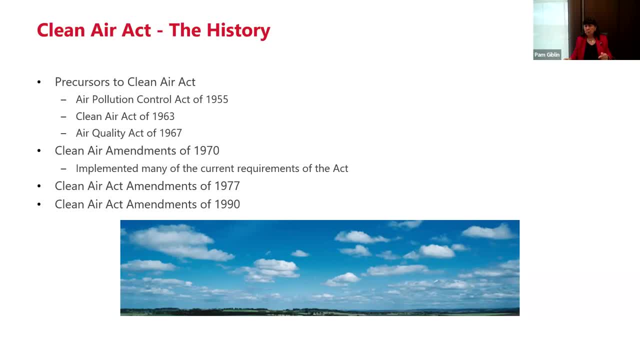 Because over time, the various requirements that a facility had to meet, as you might expect, grew in terms of Number and complexity and there was a lot of push to have that all codified in one, So that was a hallmark. Next slide, please. 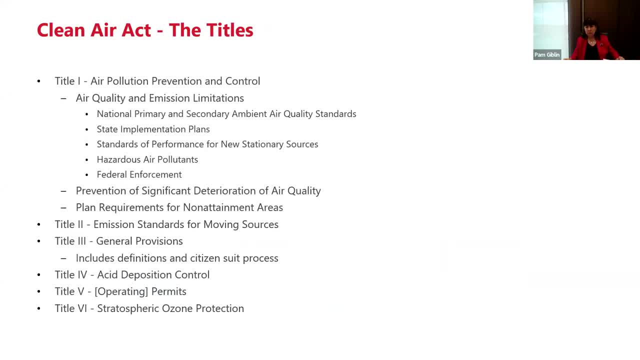 And I'll go real quickly through this, because our two wonderful panelists are going to cover this stuff in a lot more detail. This just shows the various titles- Excuse me- of the Clean Air Act And, as I mentioned, Title I, in my opinion, is one of the cornerstones. 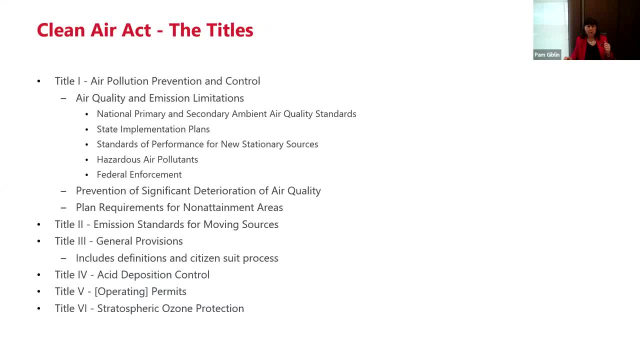 It's the true north: the establishment of the national uh primary and secondary ambient air quality, and then the, the uh psd, the prevention of significant deterioration of air quality, and all of that which came later as the pre-construction permit requirements. and then you've got other titles: uh and again uh. barun is going to talk about the mobile source piece of it. 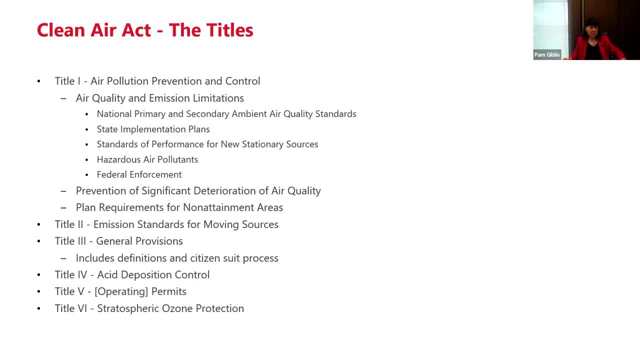 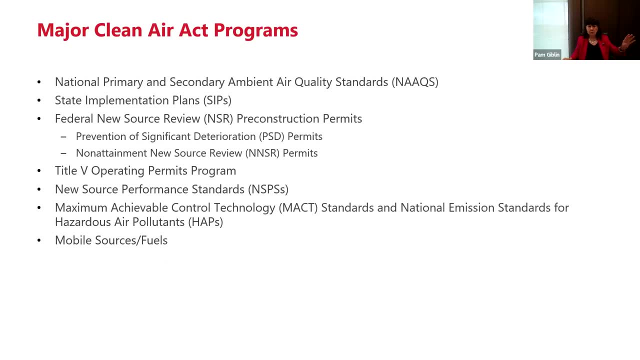 which is very significant. and then last slide, please. this again just summarizes the various programs. so, under those titles, this: these are, these are the, the programs that epa has established and is implementing with the states. and one significant point about the national primary and secondary ambient air. 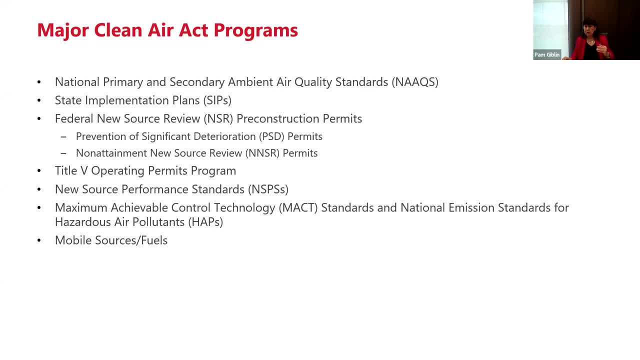 quality standards. while epa sets them and revises them from time to time, it's the state's states that have to develop what are called state implementation plans demonstrate how they are going to attain and maintain those standards within all of the states, So there's a significant role that 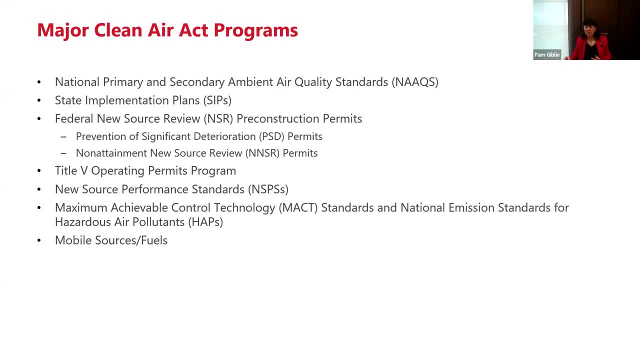 was set out in the 70 amendments. for states, EPA supervises those would use the state implementation plans, but the states have the primary responsibility to choose the mix of controls and reductions that would attain and maintain those standards. Okay, now let me. 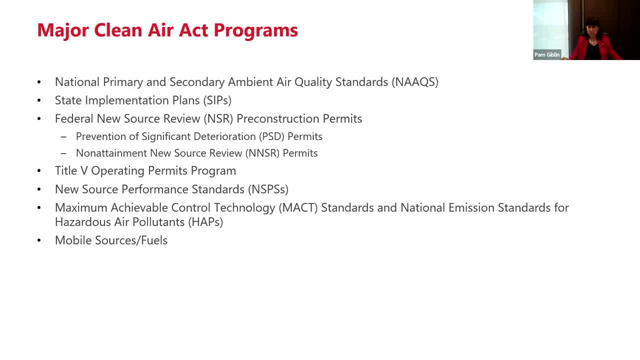 introduce our wonderful panel because I think we're very fortunate to have people that work in this every day. So Varun Shekhar is a partner at Babs Callen and he has a very broad portfolio. He works in the environmental and transportation safety group at the firm and he also works in 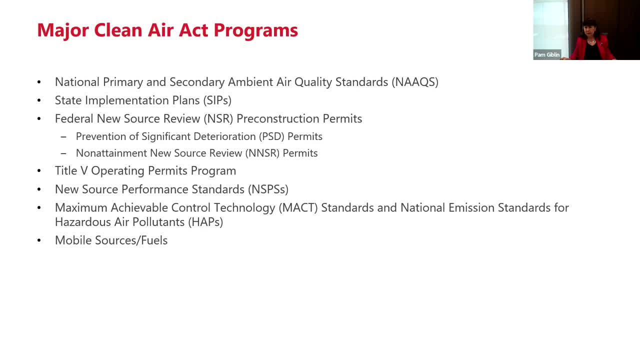 the intellectual property practice. So he has a technical background. He got a degree, an MS, in biomedical engineering, So he has the technical and the legal. He received his law degree from the University of Wisconsin Law School cum laude And, as I mentioned, he works a lot in pretty much all aspects of the Clean Air Act. 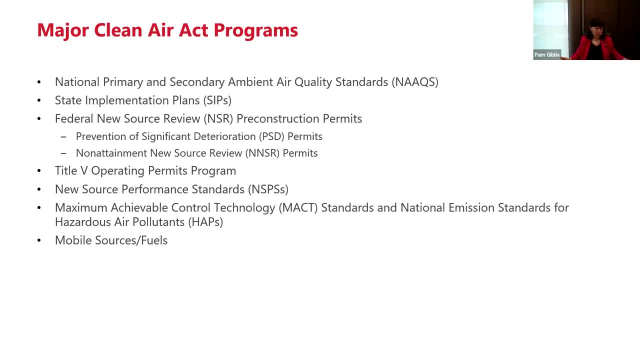 And then we're also very fortunate to have Jay Duffy, who is with the Clean Air Task Force, And Jay, his work right now is focused on greenhouse gas pollution at power plants. So one of the- again I'm so biased in favor of the Clean Air Act in terms of what an elastic statute it is, The ability to regulate. 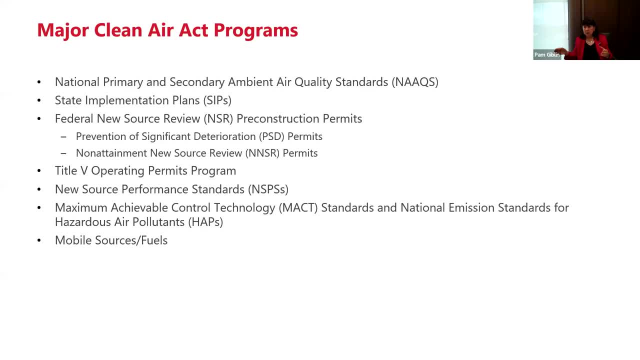 greenhouse gas emissions without a specific federal statute dealing with. that. I knew was going to come through the Clean Air Act, because the Clean Air Act has all that flexibility, And so Jay is going to fill us in on that. He has a JD from Villanova Law School, where he was associate editor of the Environmental Law Journal. 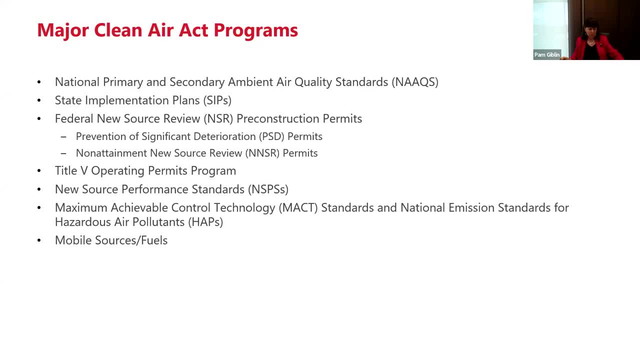 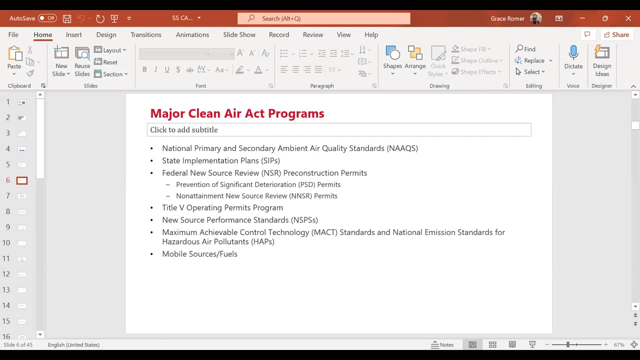 And again, he has a lot of real world expertise that he's going to share with us. So, with no further ado, take it away. You're muted. I think, Varun. You're muted, I think, Varun. For some reason my mute button went away. I don't know what happened to it. But thanks, Pam, for that great introduction. 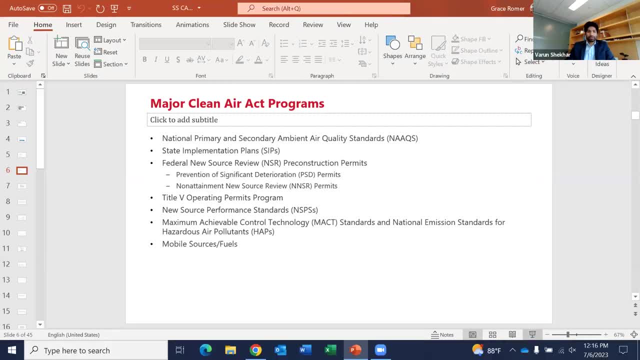 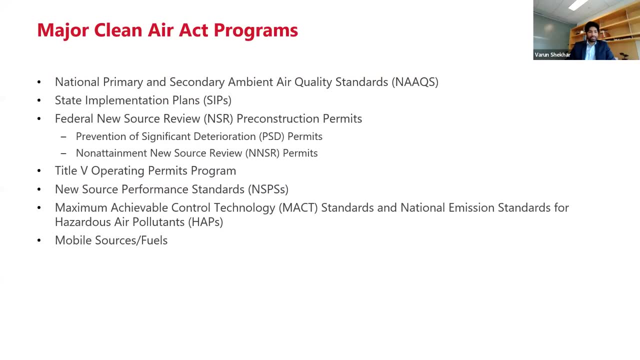 I just want to make sure, There we go. Madison, can you hear me? Yes, we can hear you now. You're good, Great Thanks. Thanks. I'm not sure what happened, But again thanks, Pam, for that great introduction. 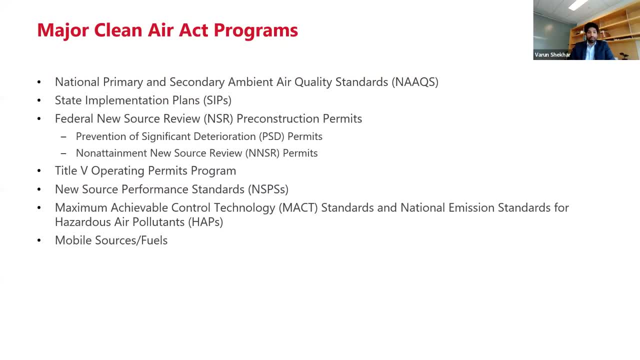 Again. my name is Varun Chikar. I'm going to be providing an overview of some of the major provisions of the Clean Air Act. Particularly, I'm going to focus on stationary source sources and mobile sources and what regulations pertain to them. 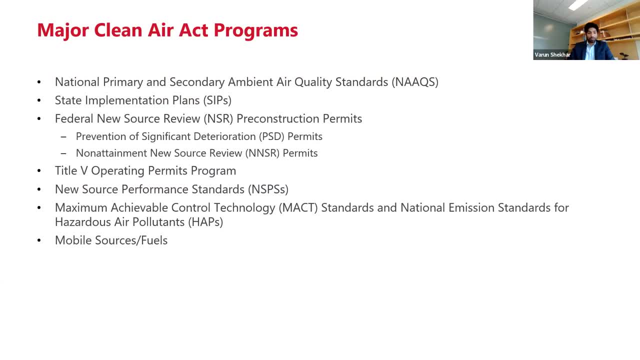 So we're focusing mainly on Title one and Title two. Also, there's some you know: Title five, for example, which also has a lot of you know. So there's some you know, Title five, for example, which also has a lot of you know. 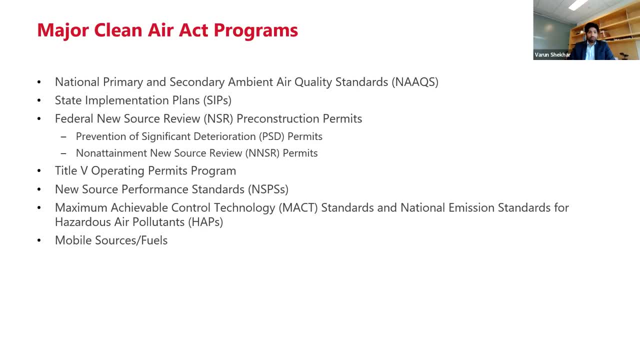 and some kind of impacts on stationary resources as well. And so, to start, I wanted to go over some aspects of the Scope of the Clean Air Act, And I want to invite all of you to just try this on yourtels, our, its site, your website, or just talk about your own policy goals. 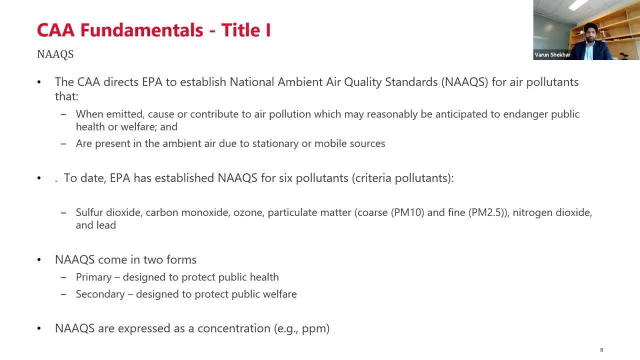 We don't just want to go to the top of our� keepbao, We also want to go to the region level Again, that is, ourAreas for this year- ulate reality. So you're going to kind of show how you can influence thisseen tid �ter. 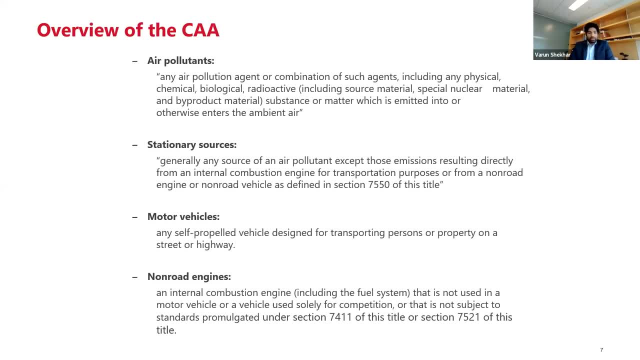 I wanted to go over some aspects of the scope of the Clean Air Act. habenidestKAbe don't it wanted to start with some kind of preliminary scoping concepts with respect to the Clean Air Act. And before I get into that, I just want to kind of underscore what Pam was saying about. 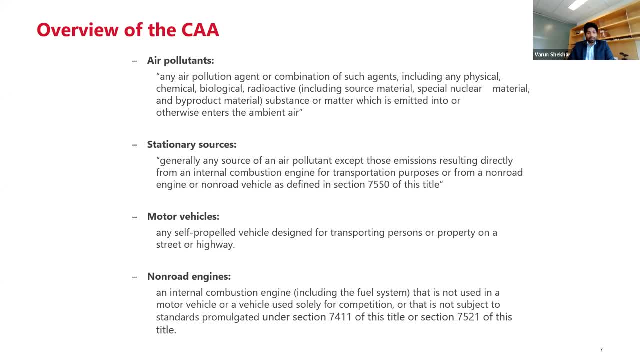 the kind of the comprehensiveness of the Clean Air Act And in my opinion it's one of the most complicated statutes out there in kind of the environmental arena. But that said, it's also arguably one of the most important, probably the preeminent environmental sort of issue that we're 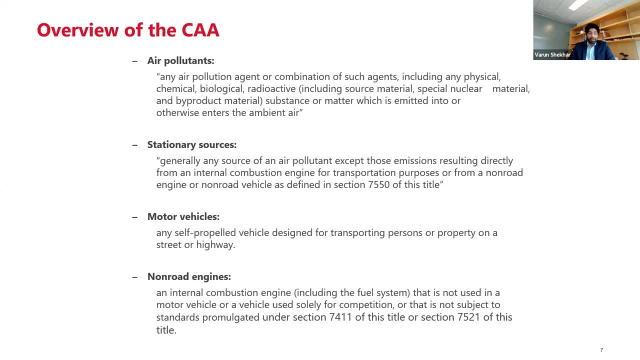 facing these days is climate change And, as Pam mentioned, it's one of the main tools, at least on the domestic front, to attempt to regulate in that area. And so you know it's a very complicated statute And there are practitioners, including Pam, who have dealt with this for decades. 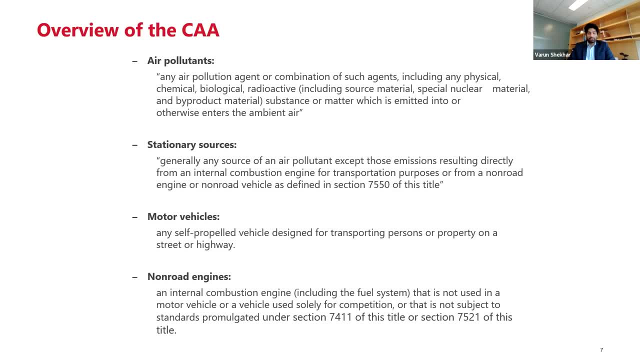 And you know, even that being so, you kind of learn something new every day about the Clean Air Act, And it's just, it can be very dense at times, but it's important to kind of understand some of its nuances And I think that I'm not going to purport to be able to, you know, cover all of it in 30. 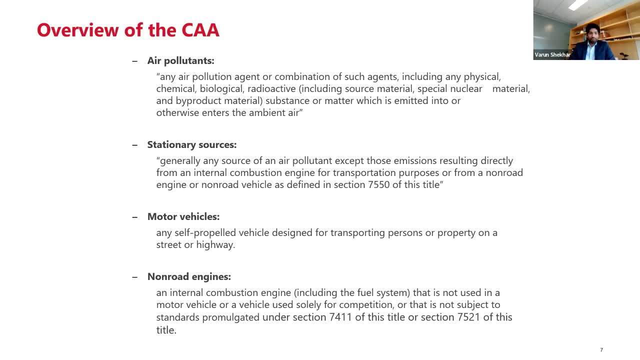 minutes. So I'm just going to touch on some of the high points. But I wanted to start with what exactly is covered in the Clean Air Act And then how does the Clean Air Act work And how does the Clean Air Act go about in regulating those aspects? So when we're starting to talk about the scope, you have to start with air pollutants, which is kind of the basic unit of what's regulated under the Clean Air Act, And I put the definition here from the statute And whenever I read it it's kind of I find it to be comically broad. 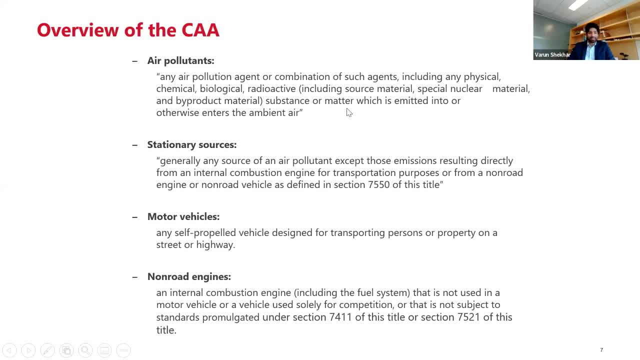 Any physical, chemical, biological, radioactive substance or matter which is emitted into or otherwise enters the atmosphere, ambient air Congress, for all intents and purposes, could have just basically replaced the first four lines of that or three lines of that with anything It is so broad It certainly. 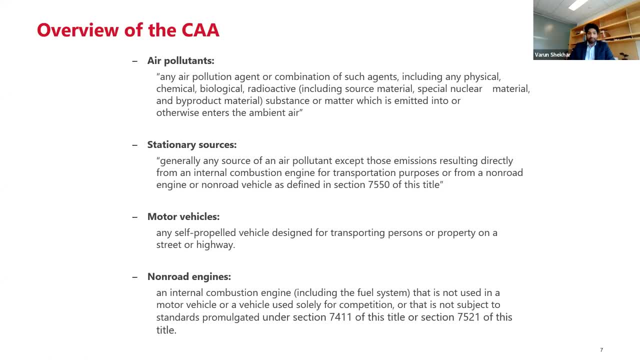 encompasses things like greenhouse gases, carbon dioxide, among other things. Now, when we're talking about some of the programs that Pam summarized, there's going to be some sort of a showing of health impacts or environmental impacts that will kind of narrow down what. 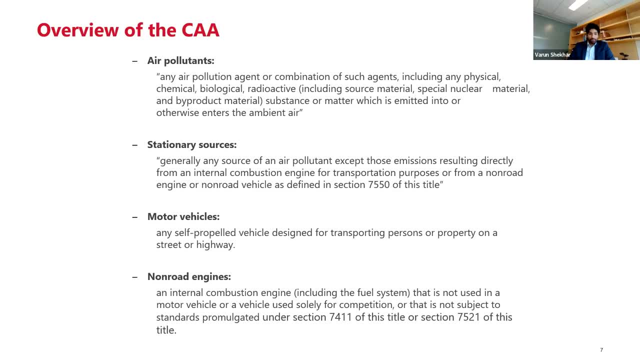 exactly the scope of air pollutants is, But it is a very broad definition. One limitation on it is in the last part of it, which is the emitted into or otherwise enters the ambient air. That's an important limitation. to kind of make it clear that when we're talking about the Clean 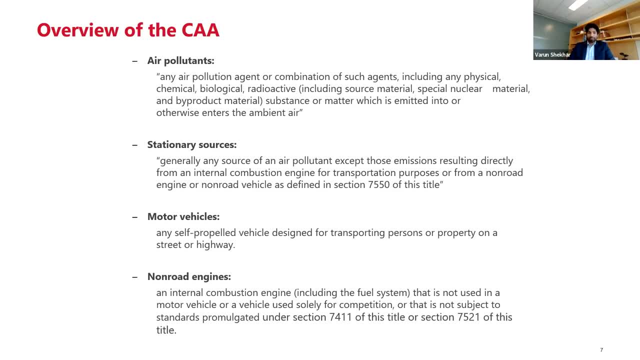 Air Act. we're not talking about indoor air quality. That is something that is more, for example, with respect to OSHA. There may be some other standards as well, But the Clean Air Act is focused on the environment. It's focused on the environment. It's focused on the environment. 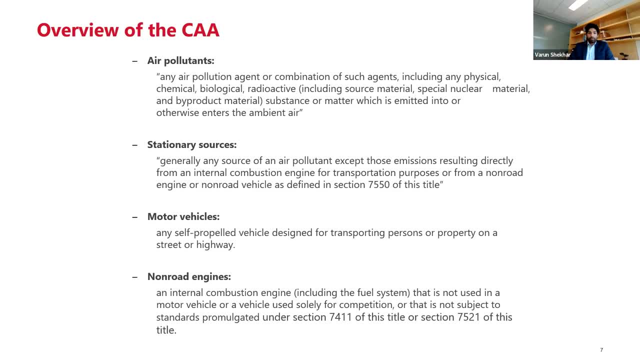 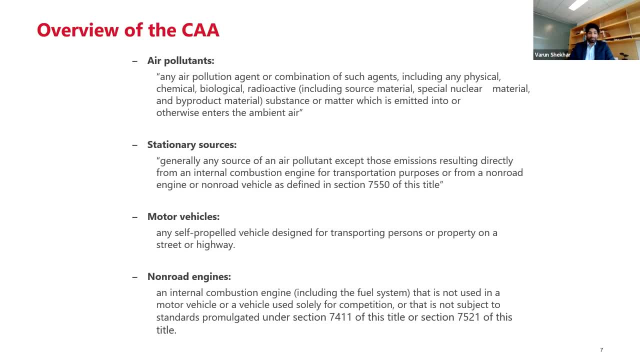 That. I have the definition there again. It's basically defined as anything which is not mobile sources, internal combustion engines for transportation purposes. So think of things like factories. It can even be things like a pilot coal that sits on a facility ground. You know, fugitive emissions that come from that, Those can. 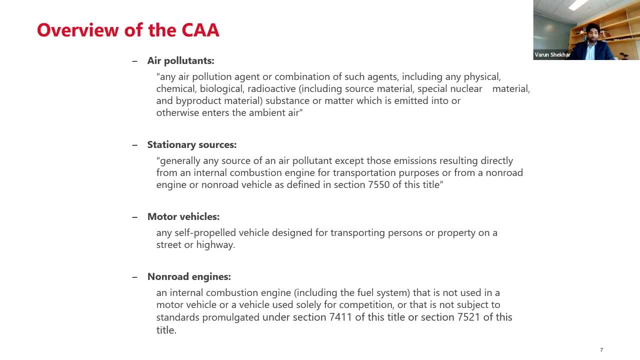 be stationary sources, Mobile sources- we're talking about things like motor vehicles, which is kind of self-explanatory, And then also a category called non-road engines. Think of things like cranes, tractors, things that don't travel on public roads. but 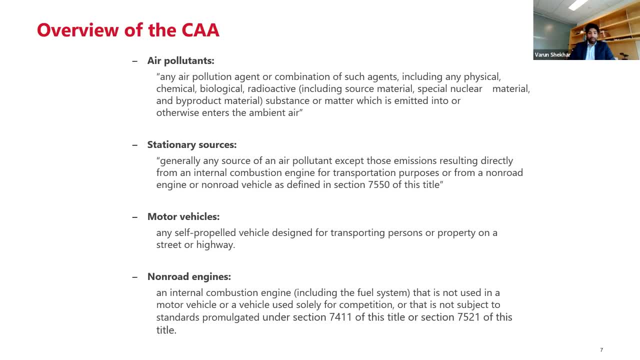 they're kind of mobile And they have engines that emit into the atmosphere. So those are the basics, And then there's also a category called non-road engines. which is a category called non-road engines, Kind of an overview of the units that are regulated under the portions of the Clean Air Act that I was. 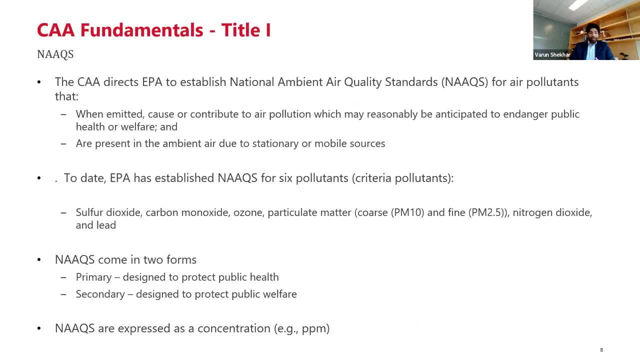 talking about. So we've identified air pollutants, We've defined the scope of them. How does the Clean Air Act actually regulate that? Well, there's a couple ways they do it. As Pam alluded to, we have the National Ambient Air Quality Standards, or, as air practitioners call them, the NACs. 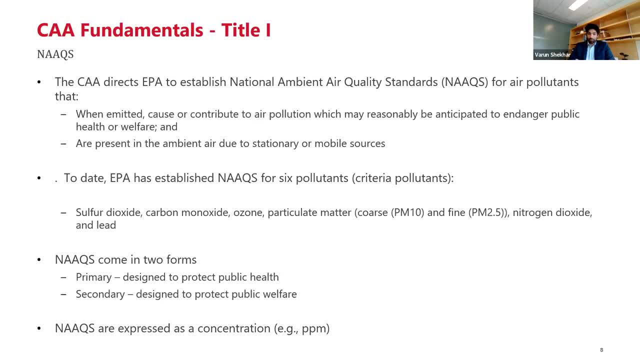 And the Clean Air Act requires EPA to establish the NACs for certain air pollutants, namely those which, when they're emitted, cause or contribute to air pollution which may reasonably be anticipated to endanger public health and welfare, and which are also present. 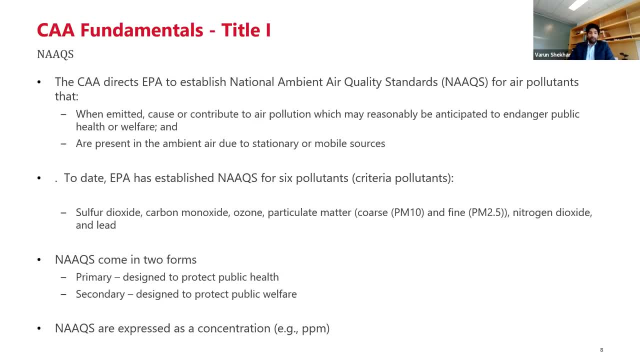 in the ambient air due to stationary or mobile sources. As Pam mentioned, there's been NACs established for six pollutants, basically from the 1970 Clean Air Act. These are called criteria pollutants And the six are listed here: sulfur dioxide, carbon monoxide, ozone, particulate matter. 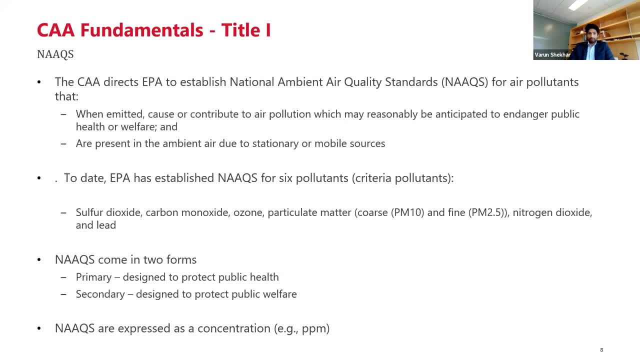 and this includes both coarse and fine species, as well as nitrogen dioxide and lead. An important add-on to that is, you know, although these are the six criteria pollutants, it also includes the precursors to those pollutants as well. So, for example, if we're talking about ozone ground, 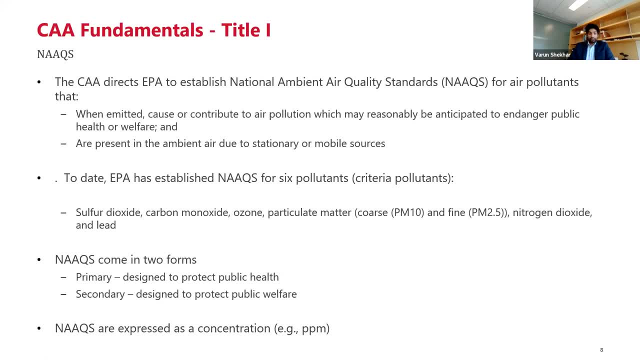 level ozone. at least two important precursors of that would be volatile organic compounds, or VOCs, and nitrogen oxides, which are a very common emission from, you know, engines and most combustion sources as well. So although this list is limited to six for NACs, it can be broader than. 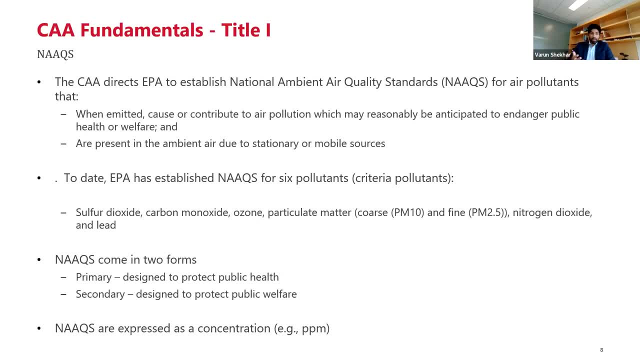 that, given you know what sort of precursors are involved in the formation of these pollutants. In addition, as Pam mentioned, NACs come in two flavors. We have primary NACs and secondary NACs. The primary NACs are designed to help protect public health. The secondary 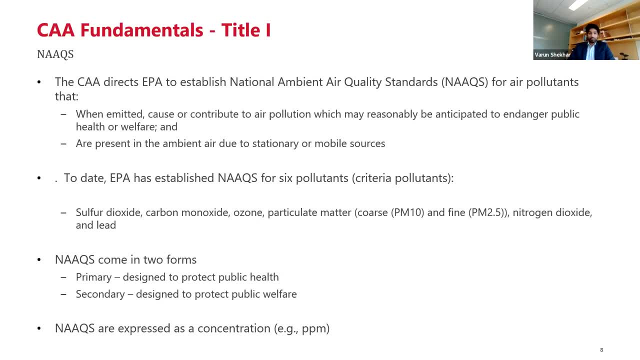 is more for kind of environmental. you know, when we're talking about things like decreased visibility, damage to crops or vegetation, Those are more of secondary NACs. Now, as far as what the NACs look like, they're a concentration threshold, So we're talking about parts per. 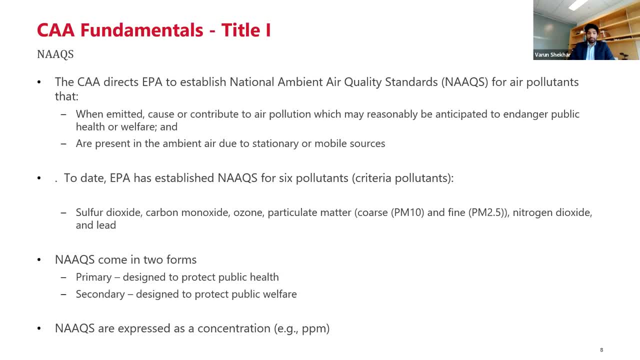 million parts per billion. sometimes it's micrograms per meter cubed, And I'm going to show what the current NACs are in a minute. But an important part of that is, you know, the NACs aren't directly applicable to individual sources, Rather they are kind of nationwide air. 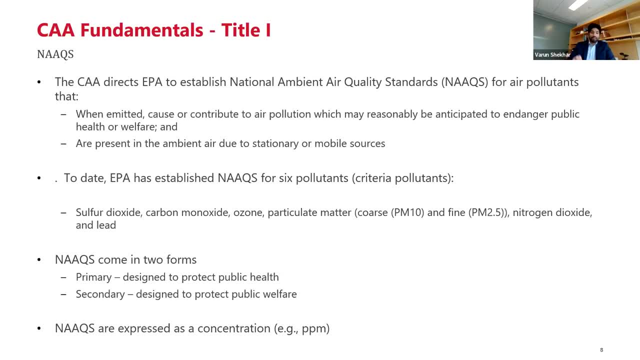 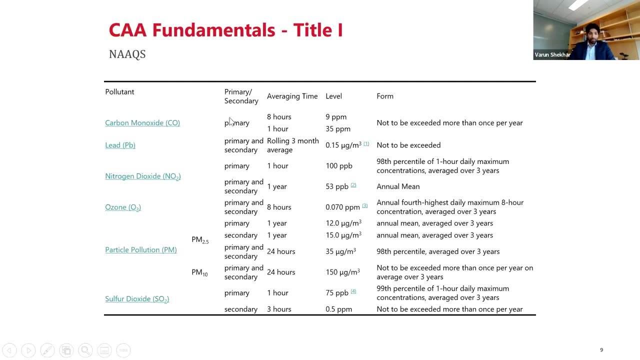 quality standards that EPA has set, But states have the onus on being able to attain them as far as the ambient air within its borders. So here is a table of the current NACs. As Pam mentioned, some have been revised Less often than others. Ozone SO2- have been kind of the more recent revised ones. 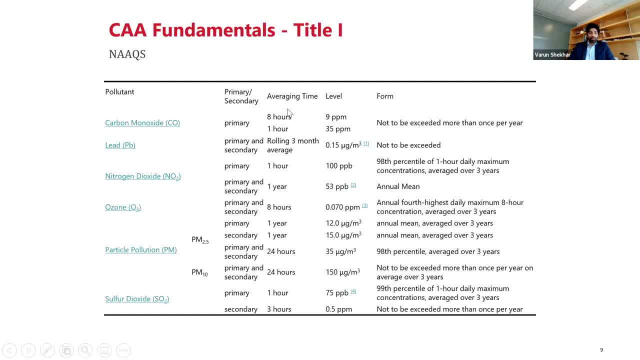 And a couple of things to point out here. So we have the list of criteria. pollutants on the left six: We have an averaging time, which is the third column from the left. So the important thing to point out there is: NACs can sometimes be designed for, at least when we're talking about, for. 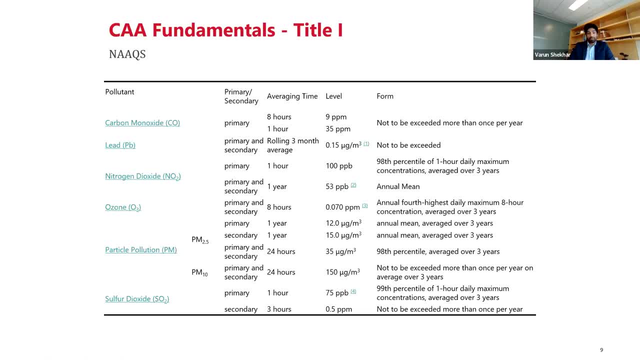 example, primary NACs designed for acute health effects as well as chronic exposure health effects, And so that's why some of these NACs have a shorter term averaging time. So, for example, ozone has both: We have an eight hour averaging time standard, as well as a one year NACs or annual NACs. 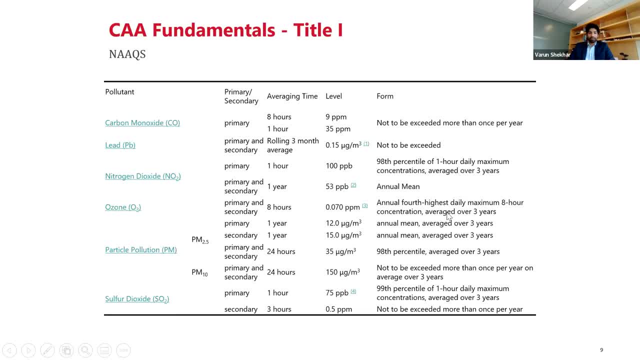 The other thing I want to point out is on the rightmost column, And the important thing with that is, as I'll talk about in a second- is that attainment of the NACs is predominantly determined through a network of ambient air quality monitors that we have installed nationwide And a recording in one of those monitors, that is. 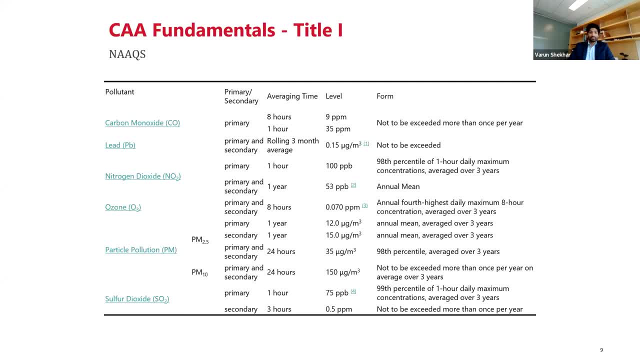 over the NACs. numeric limits here doesn't necessarily mean that you've exceeded the NACs or that you have non-attainment with the NACs. There is statistical analysis that has to go into that, based on a totality of data that's recorded by the monitor. 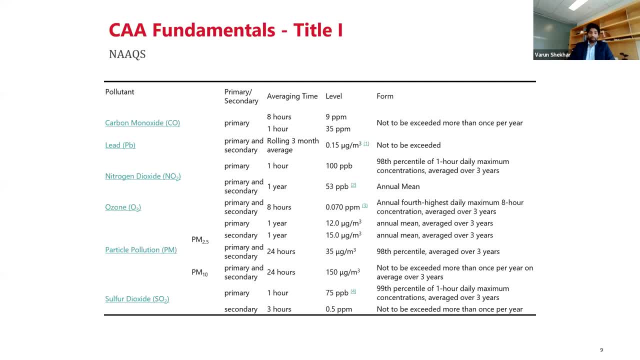 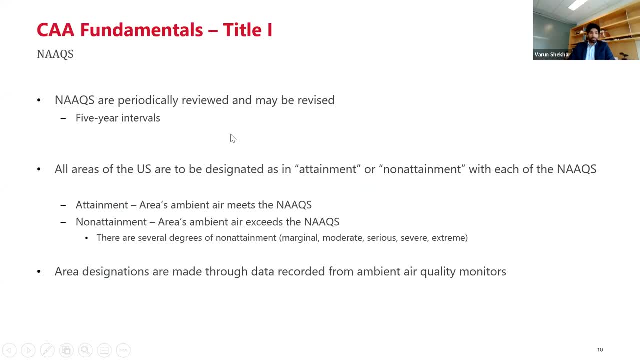 And so that's another important limitation to keep in mind when we're talking about attainment or non-attainment with NACs. As Pam mentioned, NACs are reviewed periodically. Under statute, EPA is supposed to do it on five year intervals. in practice, That doesn't always happen, And 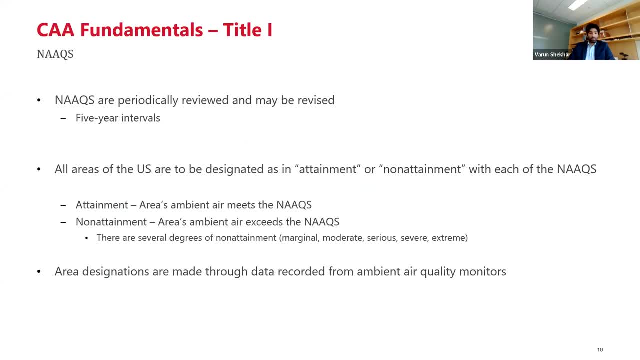 sometimes the NACs, even if there's a reason for them to be revised. EPA doesn't get around to revising them until much later, Dr Justin Marchegiani. Dr Justin Marchegiani, There's no litigation that ensues because EPA is kind of dragging its feet or a variety of reasons. 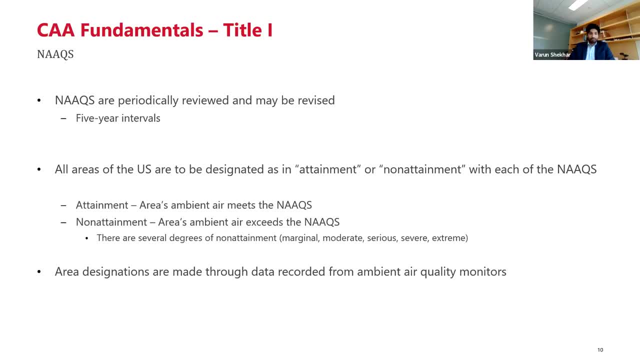 As I mentioned, all areas of the US will either be designated as attainment or non-attainment with each of the NACs. There's also a third category, unclassifiable, which is kind of self-explanatory. There's not enough data to kind of support one of those designations. It goes into that category. 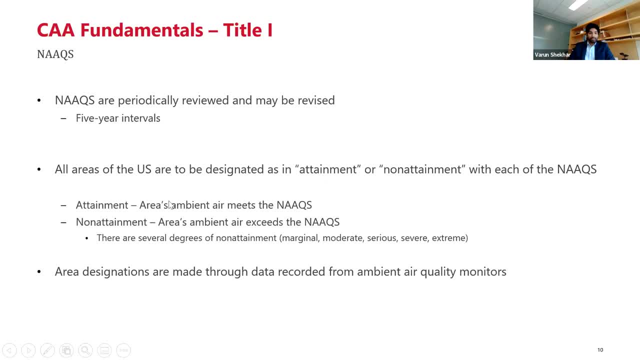 but essentially it's treated as attainment. So what those mean are kind of self-explanatory. Attainment means that the area's ambient air is at or below the applicable NACs. Non-attainment means it exceeds the NACs. 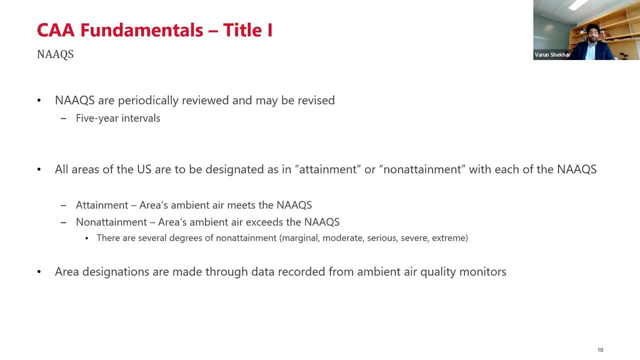 And you can have attainment or non-attainment on a pollutant-specific basis. So if an area has a relatively low concentration of ozone, for example within its ambient air, but has a very high concentration of ozone, then it's not a non-attainment. So if an area has a relatively low, 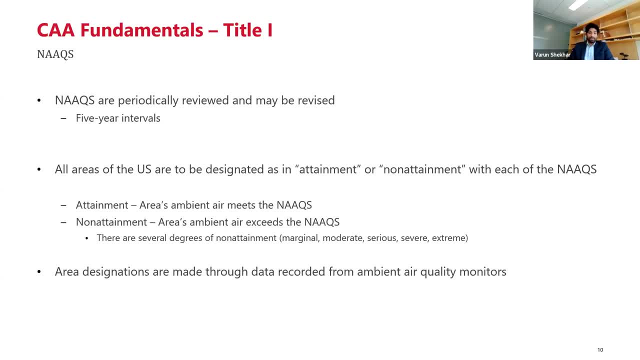 concentration of ozone, for example, within its ambient air, but has a very high concentration of sulfur dioxide, that area might be in attainment for ozone but non-attainment for SO2.. So it's on a pollutant-specific basis And, as I mentioned a second ago, the designation of 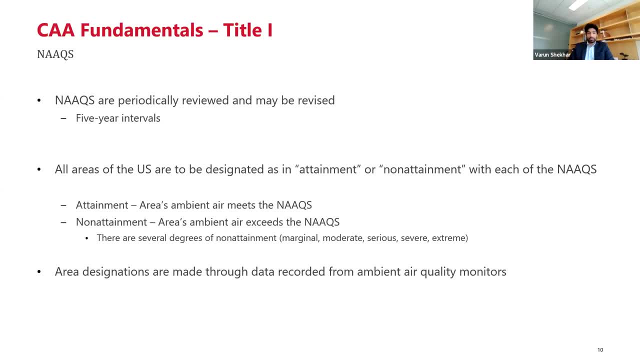 attainment or non-attainment is based principally on data that is recorded through a network of ambient air quality monitors. Sometimes the siting of monitors is an issue that comes up and there's kind of debates over it. Certainly if you have a big source- stationary source- that 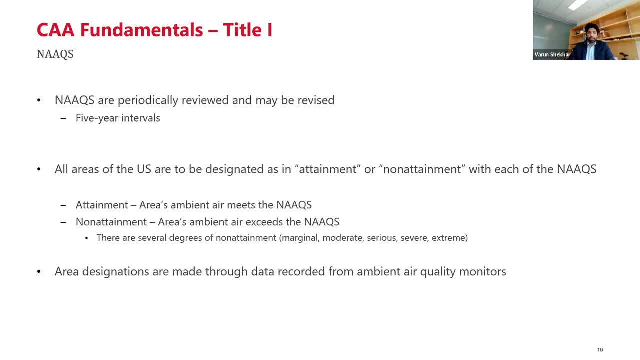 emits a lot of a certain pollutant or certain other pollutants. you want the monitors to be able to pick that up so that you're accurately characterizing what the ambient air quality is. But it can be tricky. sometimes Weather patterns might change or they're kind of variable. 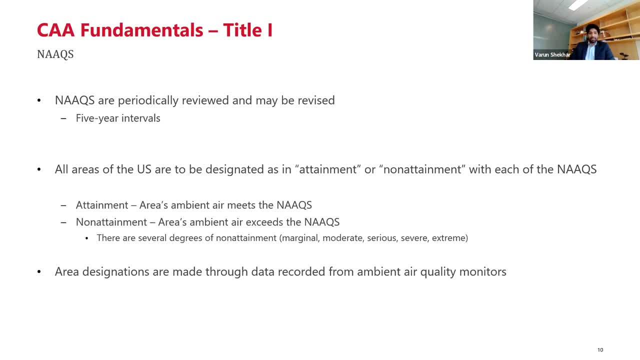 Topography can make it difficult to figure out where's the best place to site that, And obviously the universe of sources can change too. Sources open up or are newly constructed, Sometimes they relocate or close, And so it's kind of difficult to figure out where's the best place to site that. 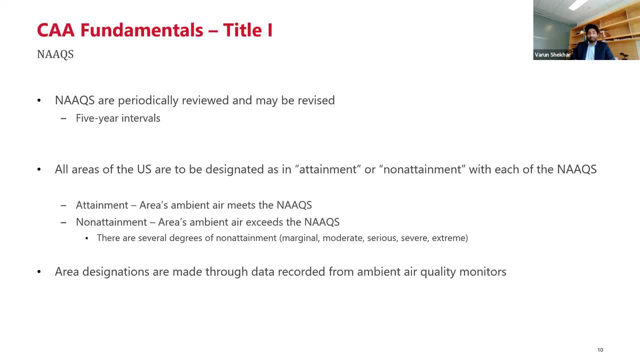 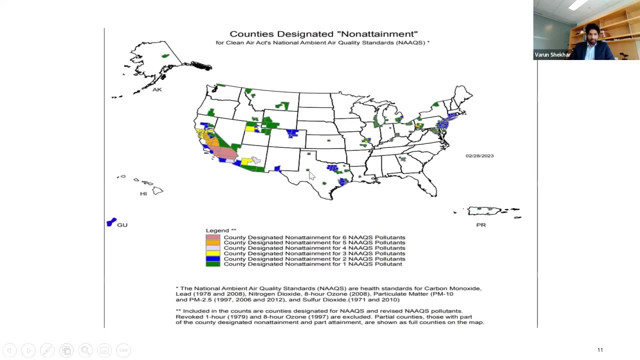 So here's what that monitoring network looks like is a very dynamic sort of process. So here's a map of the current non-attainment areas in the United States. Here, as I'll point out, California. You can see kind of in the Southern Central California area. 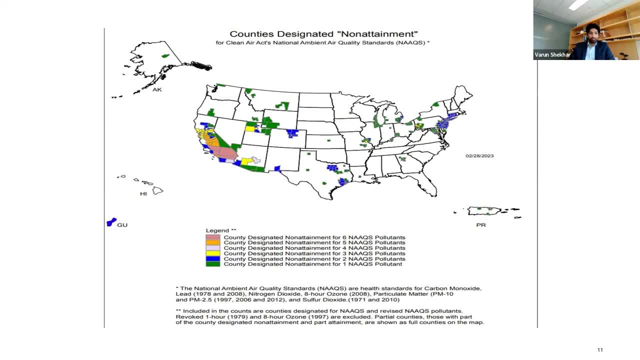 you have counties which are designated as non-attainment for all six whacks pollutants. California is kind of a of infamous in that respect for its air quality, but it's not completely due to, you know, a massive amount of industry or lots of mobile source pollution. California has kind of a unique 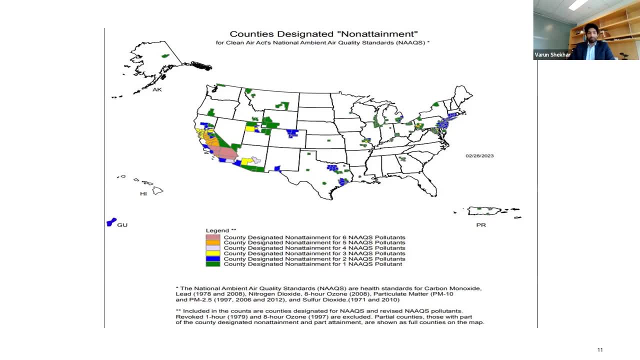 geography. There are a lot of valleys kind of dotted throughout and this can kind of trap some of the pollutants in the ambient air. There's also unique weather patterns. You have things like inversions. So you know, although those areas that are kind of shaded, you know. 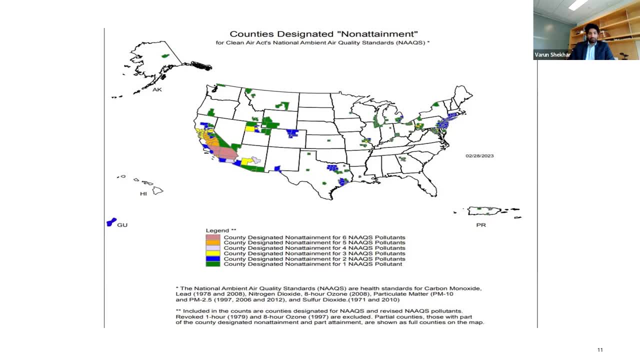 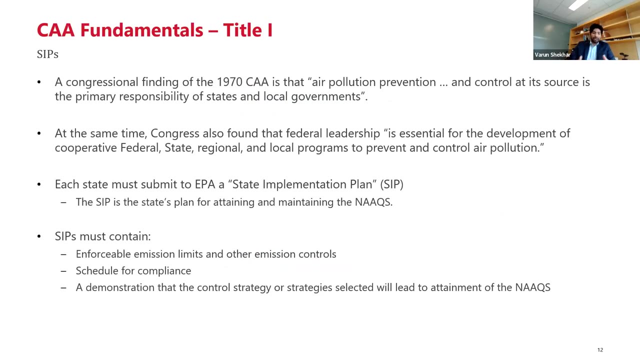 pink and yellow there are kind of isolated to California. you know there's a number of reasons for that, beyond just the universe of sources out there. So we just talked about the NACs and I mentioned the NACs aren't directly made applicable to the sources. How do they eventually? 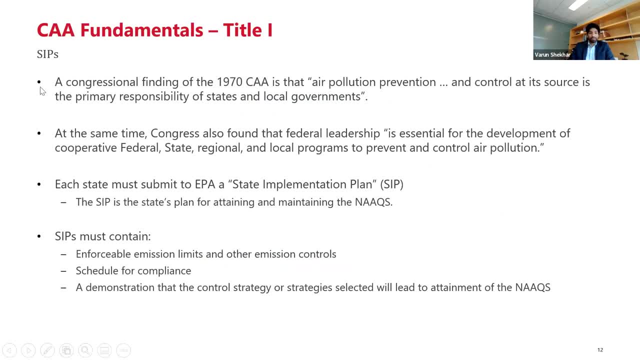 apply to sources? Well, it's through state implementation plans, or SIPs, As Pam mentioned. you know, SIPs were kind of born out of the purpose of the Clean Air Act, or one of the purposes of the Clean Air Act, which is to instill this notion of cooperative federalism, which is 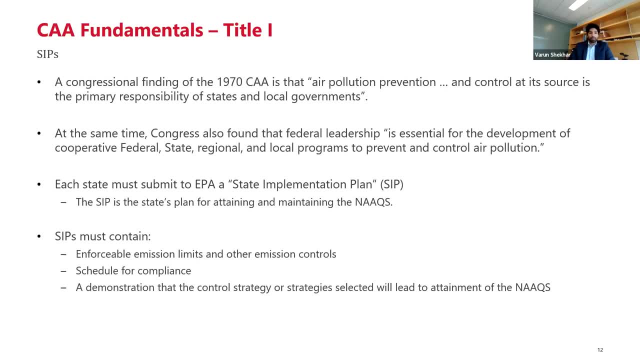 a principle that is also present in other environmental statutes, But essentially it relates to kind of these dual purposes, one being a recognition by Congress that states and local governments are to be the key agents to control air pollution, But at the same time, 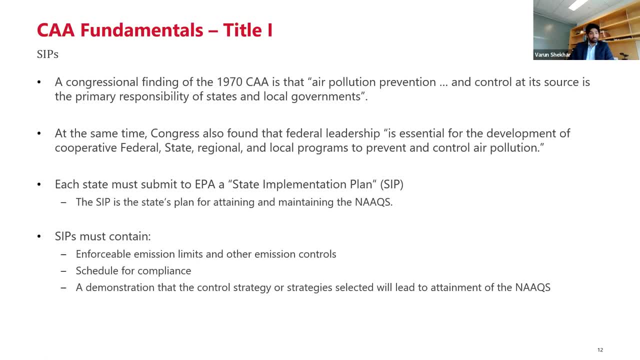 Congress also recognized that the federal government has an important role to play from policy development standpoint and in driving. you know the sort of standards, you know the state implementation plan framework And what it involves is states have some leverage or some latitude, rather, in designing what sort of control strategies that it would 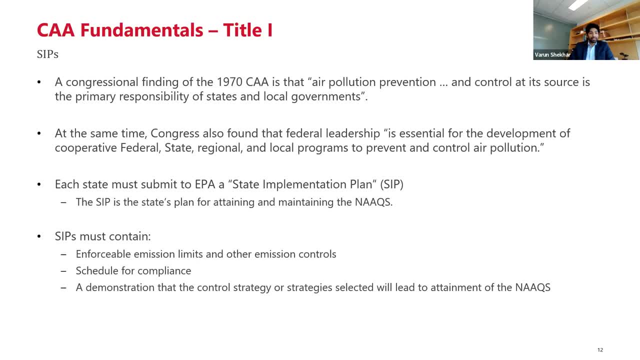 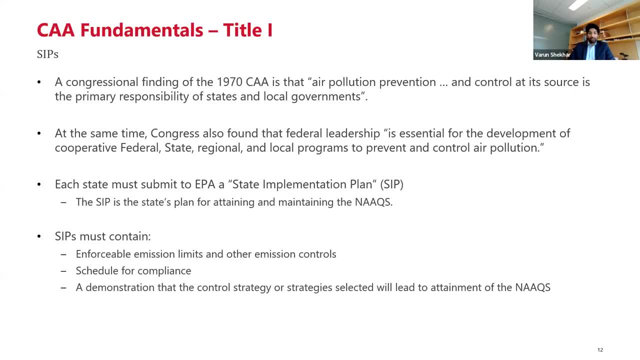 mission standards. It can be in the form of, you know, work practice standards. There are a variety of tools that states can use to put into its state implementation plan, But ultimately, what all SIPs have to contain would be some sort of a control strategy. It has to have a schedule. 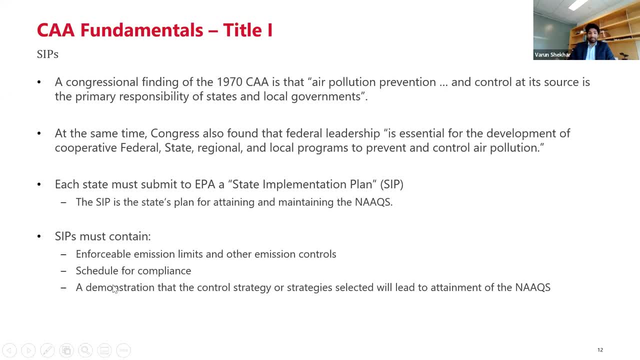 for attaining the NACs and a plan to maintain the NACs as well. And then, finally, there has to be a technical demonstration that the control strategy can be used to achieve the NACs. And so you know. 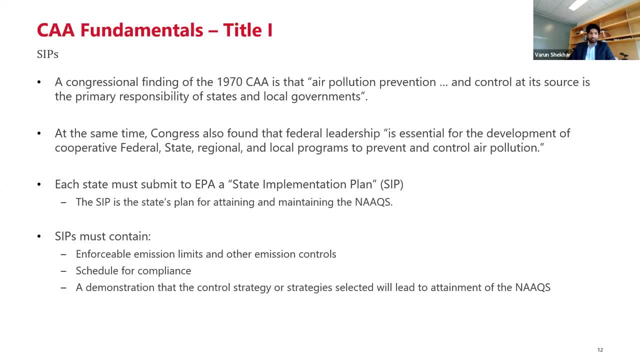 the control strategy or strategies that are chosen will actually lead to attainment and maintenance of the NACs. That last part can be. it is a very highly technical demonstration. It often involves air quality modeling, which, and this is at a very kind of high level, but it involves. 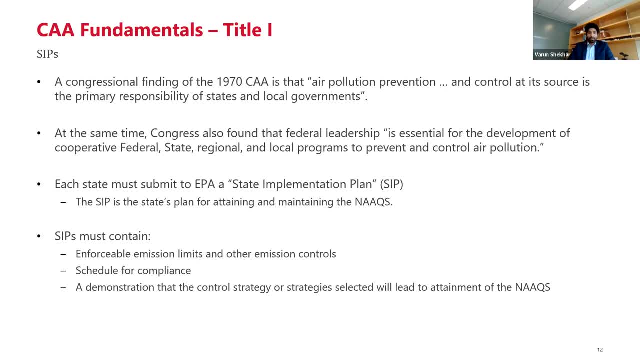 characterizing the universe of sources, the amount of emissions and the type of emissions that come from those sources, factoring in kind of a spatial aspect of the NACs, And so you know the geography aspect and weather patterns, and then using all of that and basically 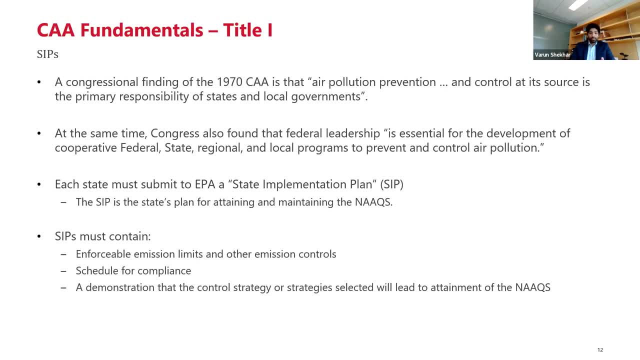 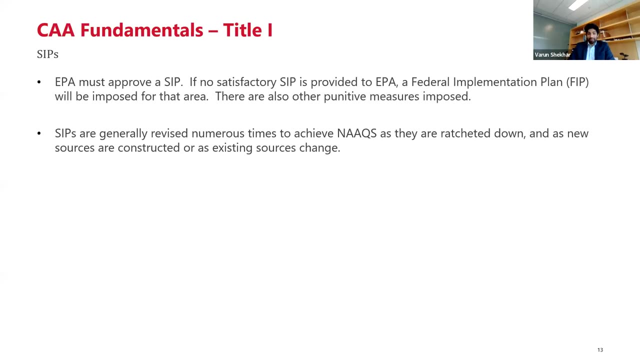 undertake implementing it in a computer program, And then with that you'll get an output which will say: well, here's what the ambient air quality is predicted to be, based on all those inputs. So all of that goes into the SIP, And the SIP is then submitted to EPA by the state. 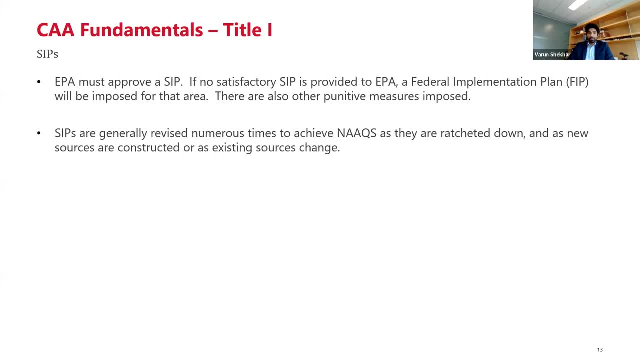 and EPA can either approve or disapprove those SIPs. If there isn't a satisfactory SIP, then the SIP is then submitted to EPA by the state And EPA can either approve or disapprove the SIP. EPA has the authority under the Clean Air Act to put in a federal implementation plan. 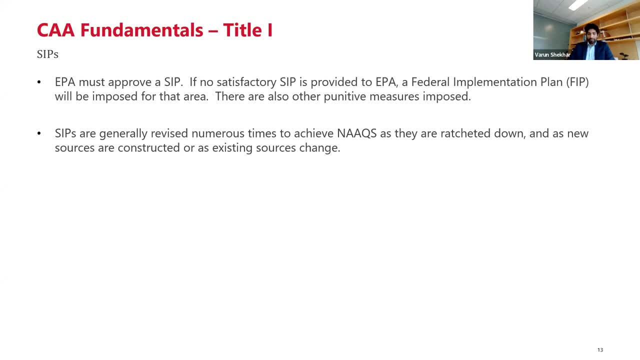 for that area And states never want SIPs because they're losing their authority to regulate the sources within its own state. So states usually are able to get an approved SIP. SIPs can also be imposed, not, you know, entirely over the scope of the SIP, but also in part. 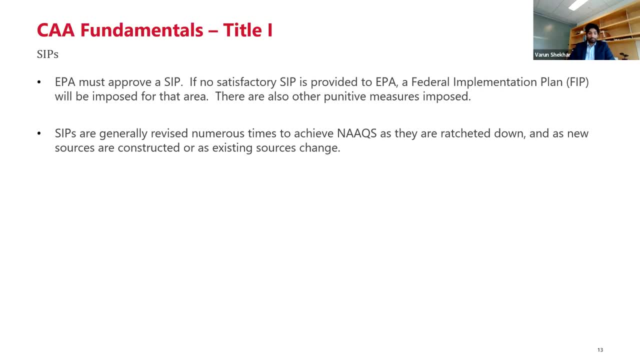 if there's certain aspects of the SIP that EPA finds unacceptable and the state isn't able to remedy that, you can have partial SIPs that just cover that area. There's also other punitive measures that are imposed if a state doesn't properly submit a SIP. 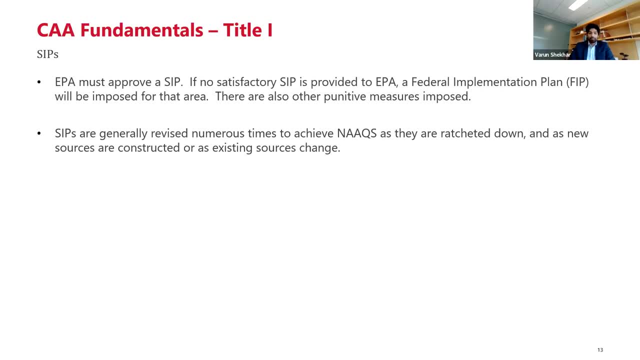 It can be things like loss of highway funding and there's other sort of offset controls that are imposed on them. So states generally try to avoid all that. Now there was a question. I saw it's a bunch of questions here. Let's pause here and go through some of these questions. I 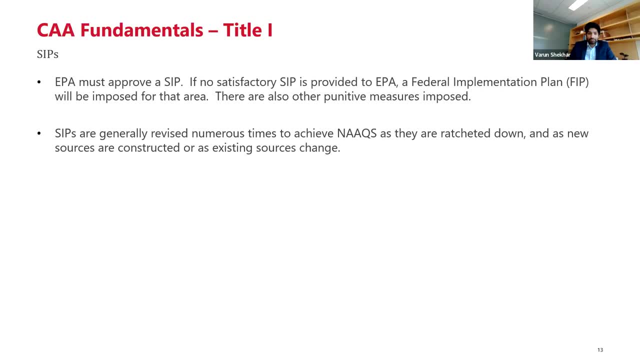 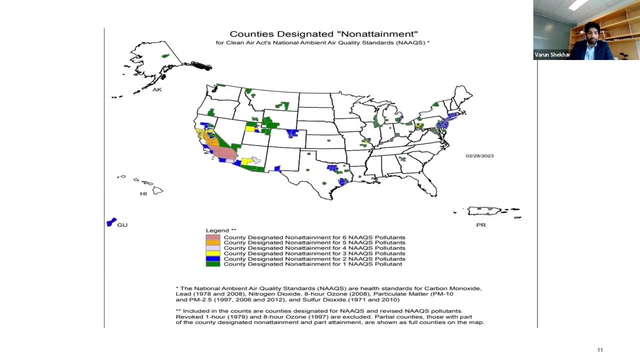 see one question. New Jersey is very clustered with two NAX pollutants. Can you speak to that a bit? What does that mean for the state high level? Let's go back to the map here. So I know I'd have to look up to see what exactly they're not attainment for. I believe. 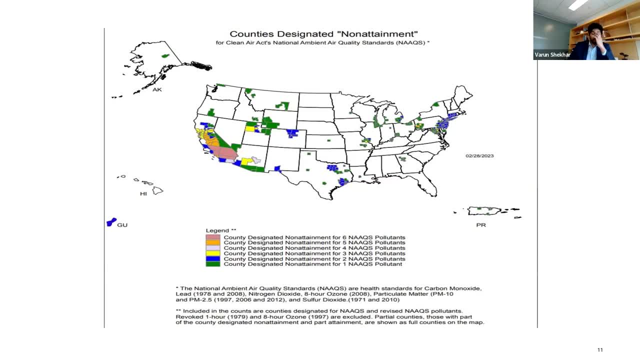 one of them is for ozone. New Jersey is also in an area called the ozone transport region, which is a kind of a bunch of states in the northeast And they're kind of treated as an odd attainment for ozone for all intents and purposes. As far as what does that mean for the state? 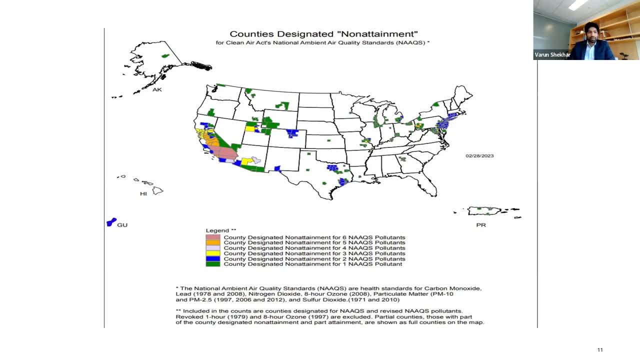 Well, I'm going to talk about that a little bit later, But if you're in a non-attainment area and if a company wants to construct a source there, that could be a little bit more onerous as far as what sort of permitting might apply. There's other sorts of controls that apply as well. 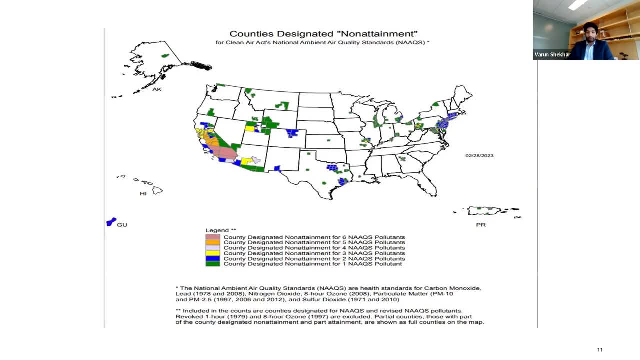 On the mobile source side, there might be evaporative fuel standards that are implemented there. I'll talk about that a little bit more. as to what happens if you're in a non-attainment area and what are the implications for sources within. I got another question: What happens when Canada? 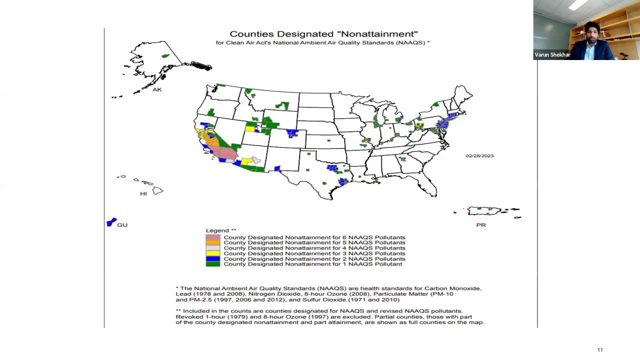 with wildfires and air quality effects are states. So internet air pollution. there is a provision in the Clean Air Act that talks about it. I'm not going to really cover it in my section, But ultimately a lot of that is covered through. 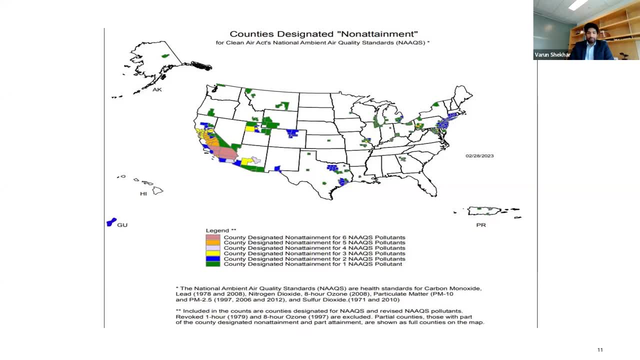 treaties And, as far as Canada goes, those do impact the next. So, if you have the monitors, when we're talking about fires, we're predominantly talking about. PM 2.5 is the main issue with that, And so those monitors, moment after monitoring very high concentrations. 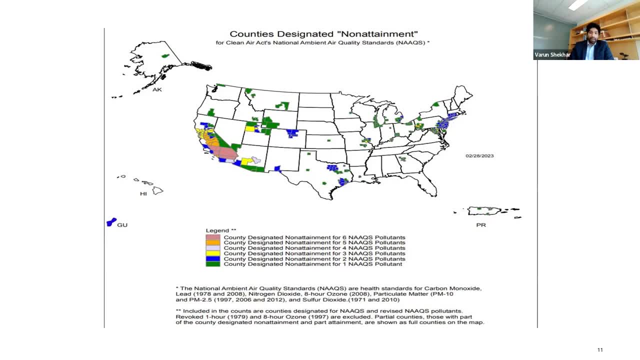 the PM will be now. So they are going to impact to some extent, or could impact, in kind of attainment designations, Although in practice the EPA is going to look at the long-term averaging of that. We go back to the PM standards. 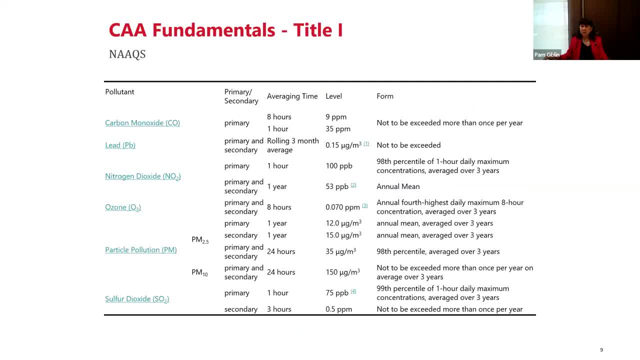 Go back to that real quick. Let me show this. Please go ahead. there is an exceptional events rule that's subject to a lot of litigation right now, so that wildfires, for example, either domestic or international, are not counted, and that's, like i said, it's subject to a lot of debate right now, but the exceptional events rule would also. 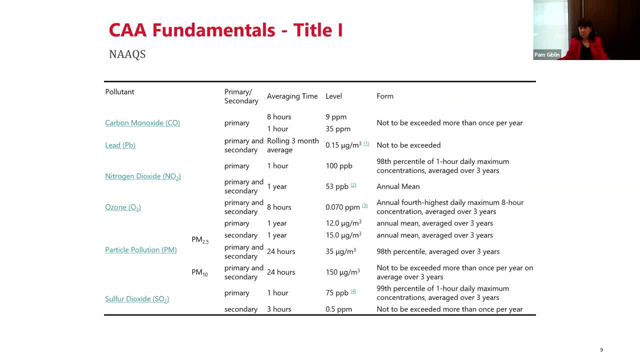 apply probably to canadian wildfires. yep, and that's that's a regulatory provision, that why it's under a lot of uh debate, but, um, that is, that is certainly a a provision. that's that's going to be argued here, uh, because otherwise states are going to have at least the effective 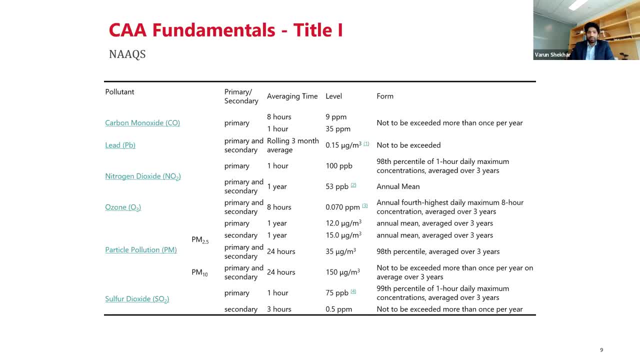 states are going to have a lot of non-attainment issues. um. can you speak to why the greater new york city area is designated non-attainment? so i i think one of them is ozone. i'd have to double check what the other, what the other pollutant is? um, why is it non-attainment? um, likely because of. 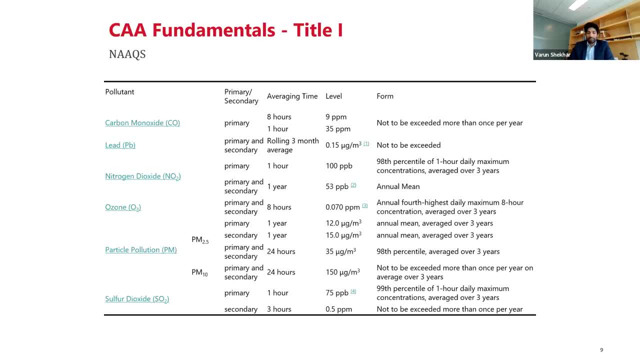 industrial impacts, uh, you know various sources in the area. the other thing i want to point out on some of these non-attainment is you can have downward impacts, and the clean air act has a provision called the good neighbor provision, which requires um epa to uh regulate uh interstate uh transportation of air pollution, and so there's. 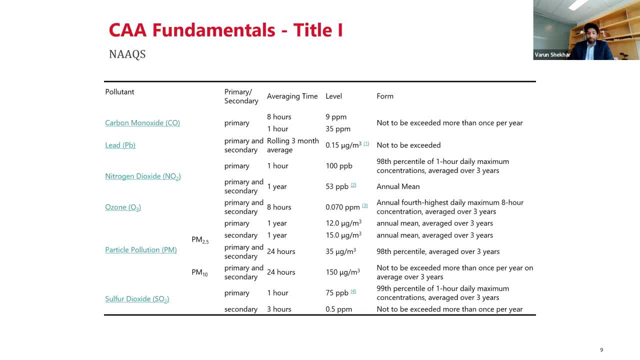 there's a rule that came out fairly recently called a good neighbor uh rule, uh, and a fit that was also imposed as part of that um, and so, uh, as- and i also mentioned earlier, uh, a lot of these are in an area called the ozone transport region, um, and so my, my guess is that, new york being in 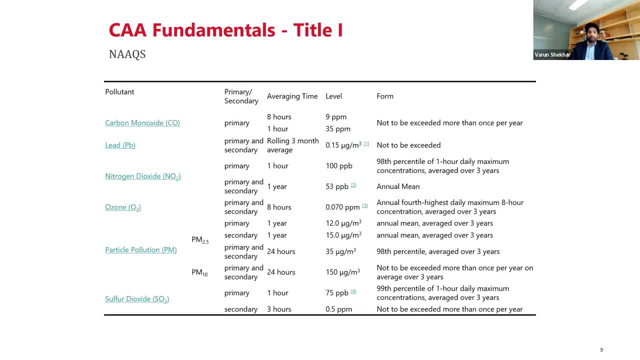 that location is probably impacted by some of that. uh, what do you think is the best advice or information to give employees when giving an educational presentation about the cleaner act or company? um, that's, that's a interesting question to, to feel i. i let we'll come back to. 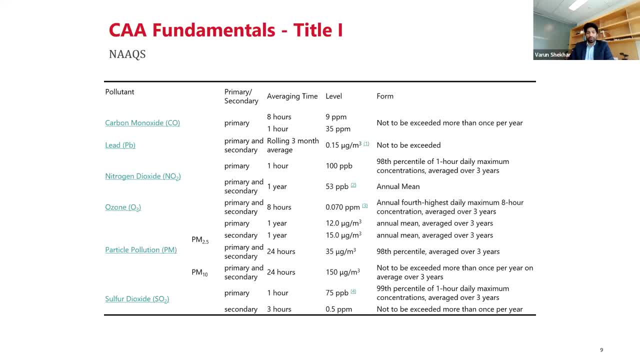 that i think maybe towards the end, once we have, when we cover all of the cleaner act uh provisions, what's the status of epa's pros or visions to the pm 2.5 standards? so i think i'm going to talk about pm 2.5 a little bit later. um, we'll come. 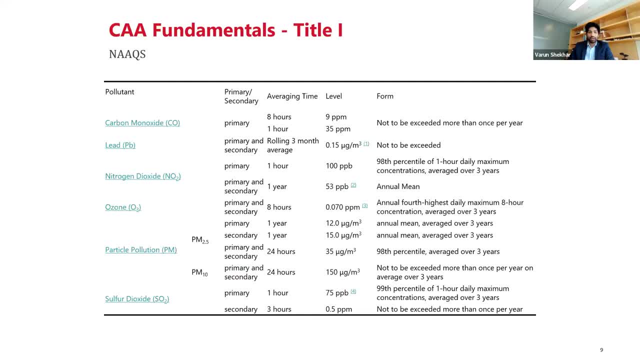 back to that as well. mobile source or engine is operated in a building at a stationary source, are the emissions considered mobile source emissions? are those considered part of the stationary source. so i what i gather is: let's say, you have a tractor or something that, a that is in a building. are those emissions mobile source? so the, so the engine that is part of that. 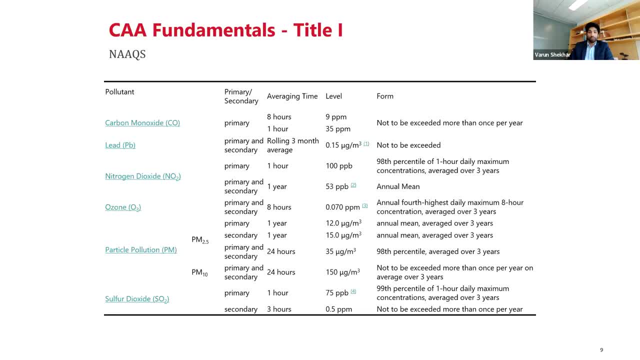 vehicle would be regulated most likely under title two. um, if it qualifies as a non, probably be a non-road engine at that point. uh, as far as emissions that come from the vehicle into the source and then from the source of ambient air, it kind of depends what emissions we're talking about. 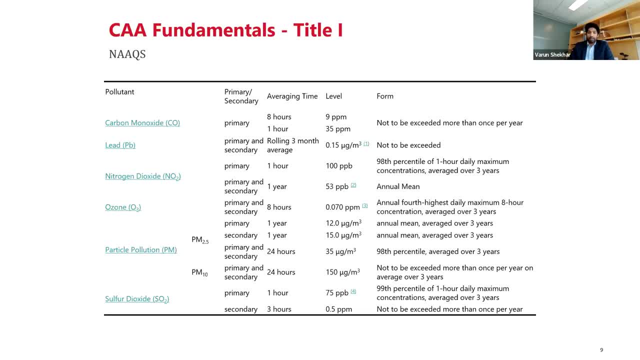 if we're talking about things like volatile organic compounds. um, epa has pretty detailed guidance as to when something that goes into the inner space of a building but might be exhausted out- uh, out of the building through a window or the exhaust system. when, when does it count as? 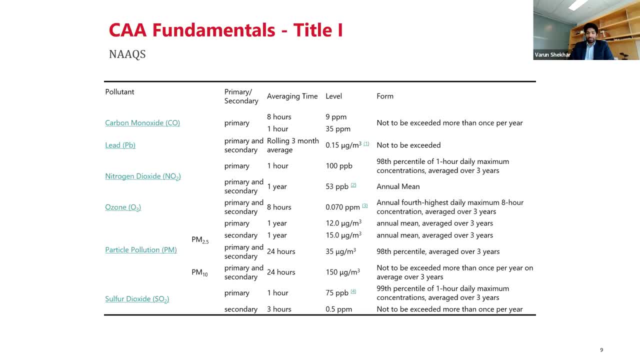 emissions of the ambient air. again it depends on the pollutant. if we're talking about something like voc, if that building has an exhaust system that basically collects it and just pumps it out to the ambient air without any sort of control of it or destruction of that, that might be. 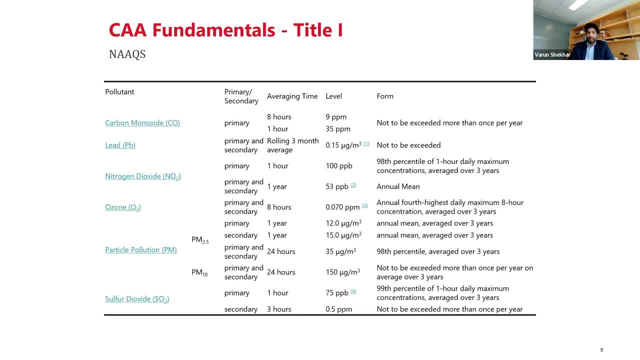 considered emissions from the stationary source. if it's something like pm uh that doesn't really exit the building and or if it just kind of stays trapped inside uh without much emissions coming from it, it arguably would be uh not considered uh regulated in the clean area. all right, let's pick. 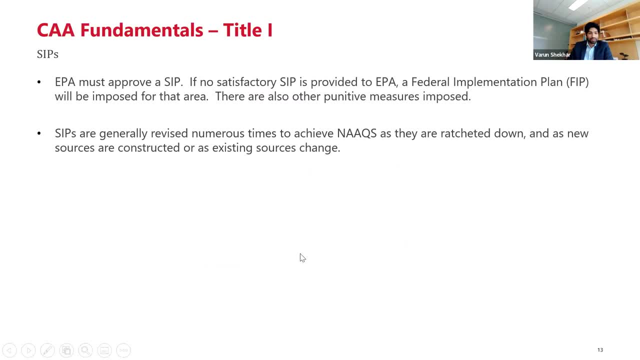 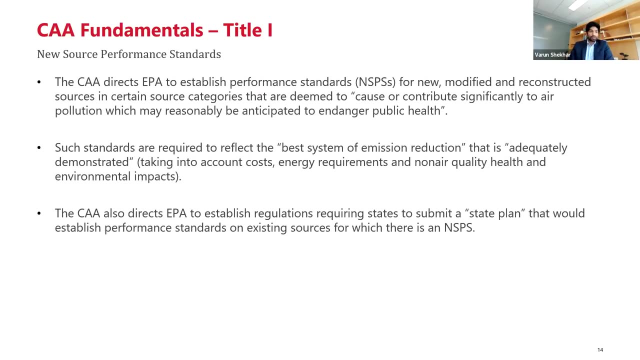 up again. where was i? so we talked about sips. um, so sips are one uh route to regulate air pollutants uh. another way that uh regulation occurs is through new source performance standards, and these are federally uh imposed standards and promulgated standards uh that are for new, modified and reconstructed sources that are in. 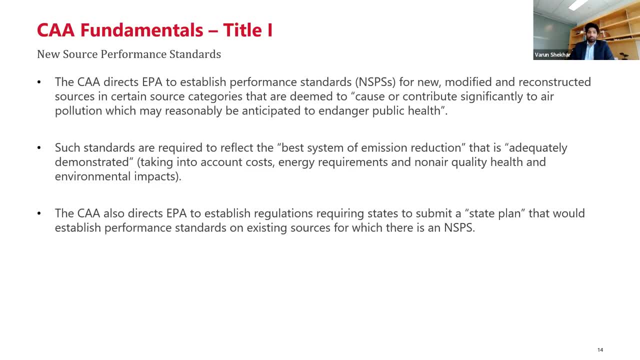 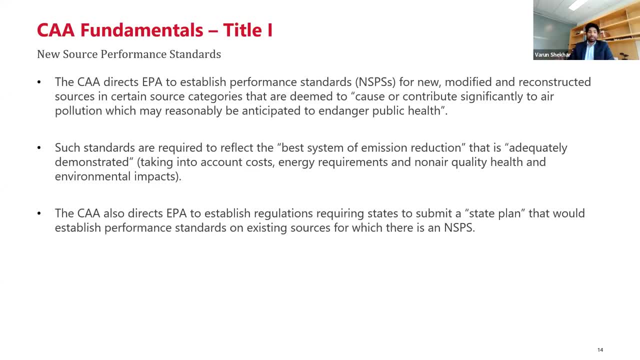 sources that are in those categories. um, the standards that are that that are imposed under the nsps program are required to reflect the best system of emission reduction. uh, sometimes short for bs. This was an issue that came up in the power plant carbon dioxide litigation: West Virginia versus EPA considered standards that were for existing sources, which I'm going to talk about actually in the third bullet. 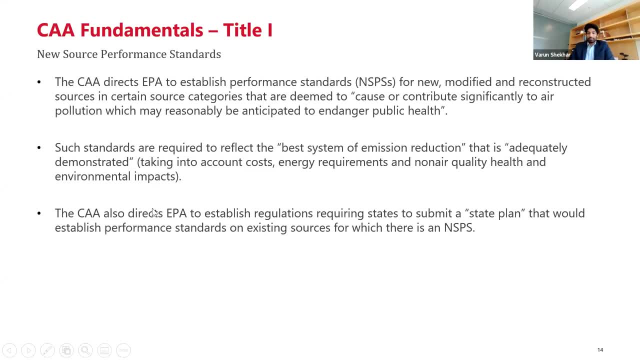 But the best system of emission reduction was a key element of that. What does that entail? Is it a control device That could be a best emission reduction? Is it something which is more industry-wide? Is it, for instance, shifting the sources of power generation away from, for example, coal-fired power plants over to renewables or natural gas-fired power plants? 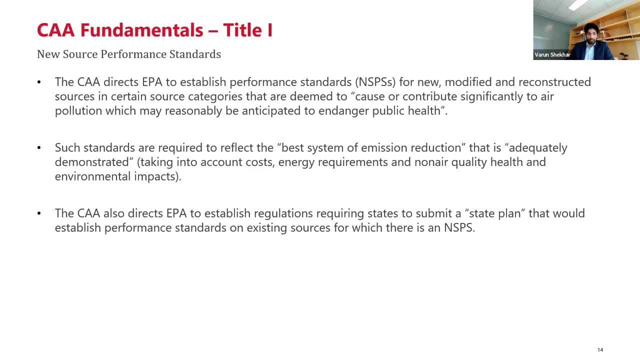 That's an issue that Ajay will talk about a little bit more in the West Virginia case. And then, as I said, we're talking about new, modified, reconstructed sources. There's a parallel section, This portion of the statute, which requires EPA to establish similar regulations on existing sources under those source categories. 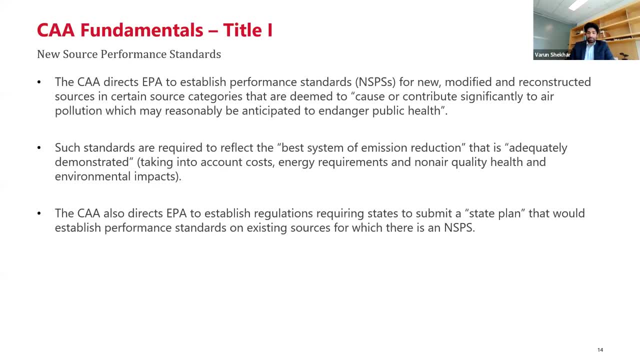 The standards wouldn't be a numeric standard that applies to the source directly, as it would for new sources. Rather, the way that those are regulated would be through a state plan. It's not a SIP, but it's a state plan that might be incorporated into the SIP. 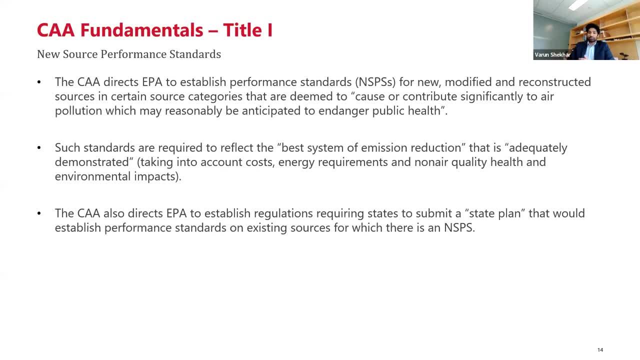 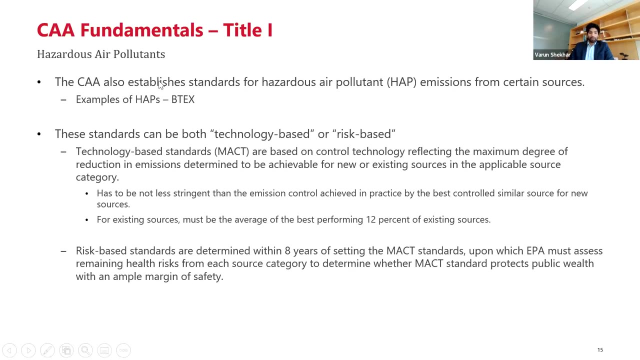 But it's a state plan where the state would have latitude to develop some sort of policy Or control strategies that would achieve the existing source performance standards under that provision. Another aspect to regulation of air pollutants is for hazardous air pollutants or air toxics. 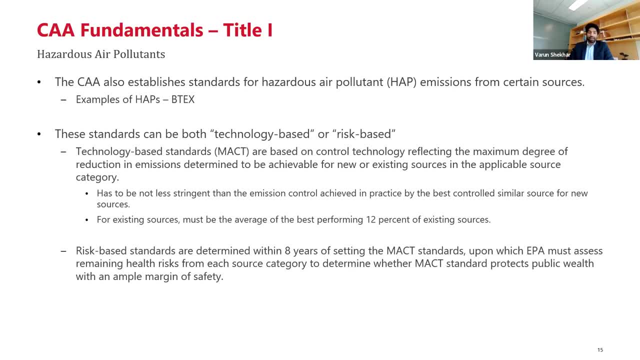 The Clean Air Act had provisions on this, but they were really ramped up in the 1990 amendments. And when we're talking about hazardous air pollutants or HAPs we're talking about. There's a long list of them, but the ones that kind of come to mind first are the BTEX constituents. 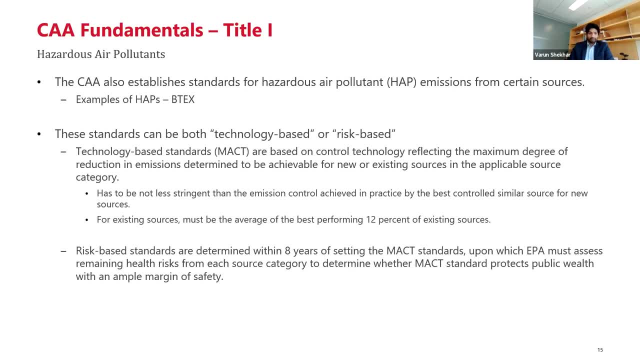 Benzene, Colluene, Ethylbenzene, Xylene. These standards can be both technology-based as well as risk-based. The technology-based standards are also sometimes called MAX standards- Maximum Achievable Control Technology. Achievable Control Technology. 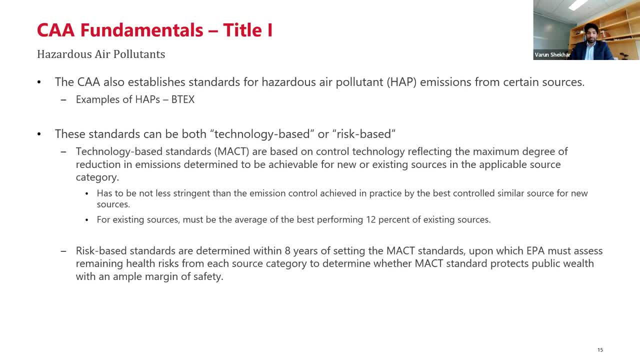 And they are based on control technology that reflects the air pollutants, That reflects the maximum degree of reduction in emissions. How does That's achievable? How does EPA determine that There's a statistical analysis to it? For new sources, they would look at the best controlled similar source. 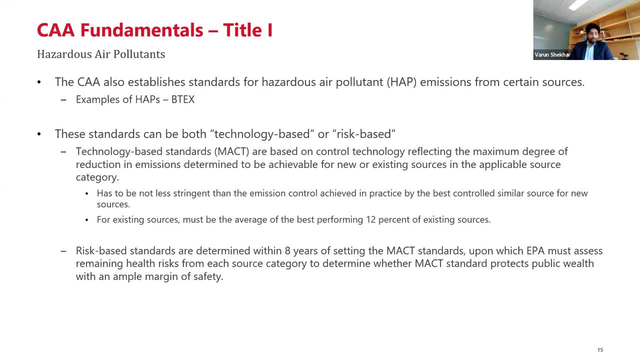 And they see what sort of controls are in effect there. Whatever emission rate is being achieved through that, that becomes the MAX standard for new sources. For existing sources, The MAX is determined through the average of the best performing 12% of the universe of existing similar sources. 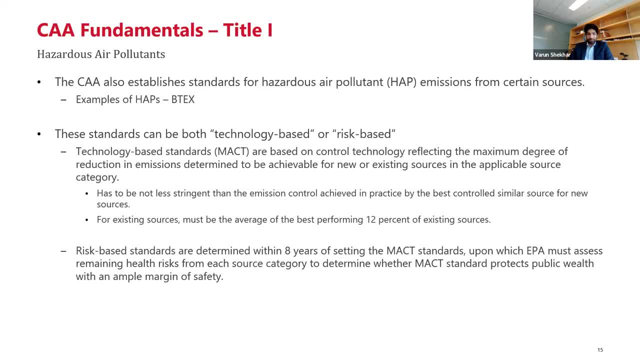 So those are the technology-based standards, But there's also a second component to it. Those are risk-based standards. So every eight years EPA is supposed to do a review of the adequacy of the MAX standards And if there's deemed to be a residual remaining or residual risk to public health, 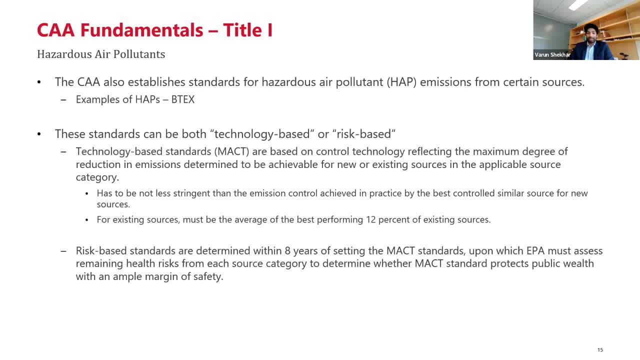 In those You know from those standards. if they're not adequate enough, EPA can impose what's called a risk-based standard, And the risk-based standard is based on kind of these health endpoints And they're set where it allows for an ample margin of safety. 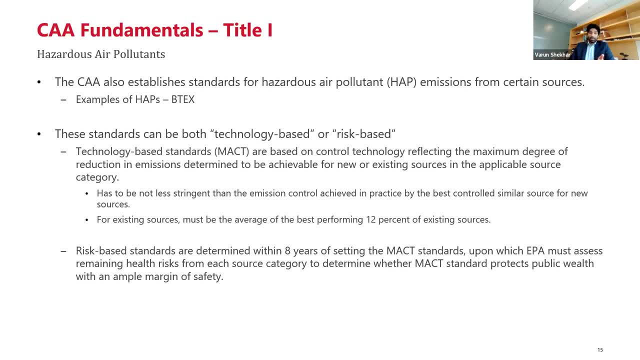 So you'll have a certain, for example, carcinogenicity risk And EPA will consider that They'll have a certain margin of safety that they seek to implement And out of that comes a numeric standard that's applied. These are for again, for certain sources. 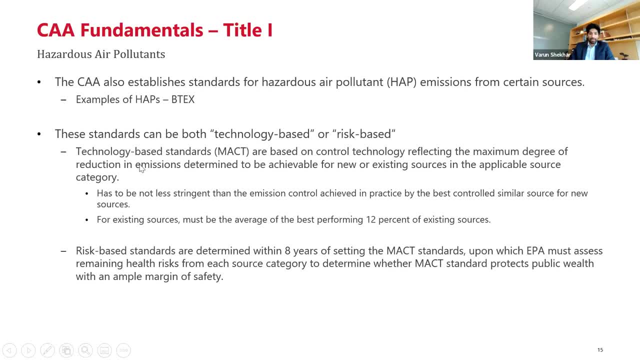 Another alternative term for them are NSHAPs- National Emission Standards for Hazardous Air Pollutants- And there's a couple of questions I see here on this. Where are we? I think there was a question. I kind of lost my place. 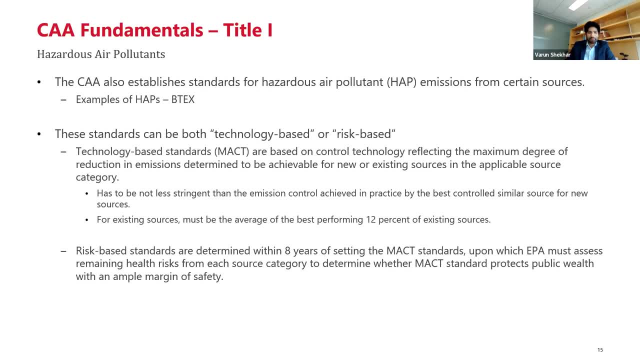 But I think there was a question as to how do the hazardous air pollutants, or the NSHAPs, mesh with the NACs. So they're separate. The NACs are for the criteria pollutants, Criteria pollutants. none of them are HAPs. 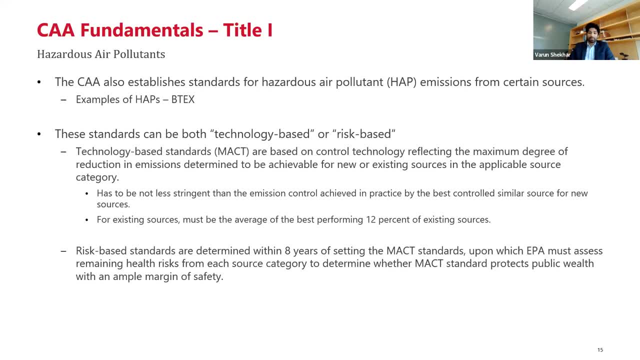 The HAPs are separate from that, And the NACs, as I mentioned earlier. how do we achieve the NACs? There's a variety of ways you do it. The state implementation plans, That's kind of the key tool in achieving. 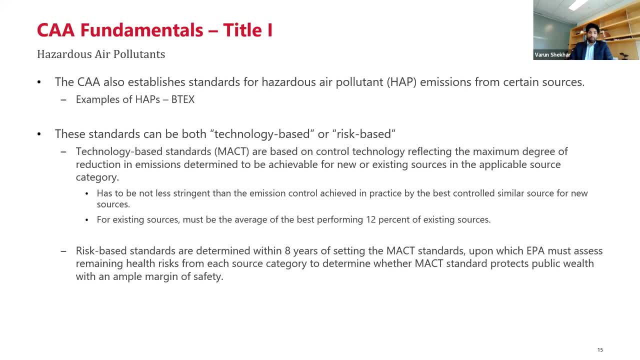 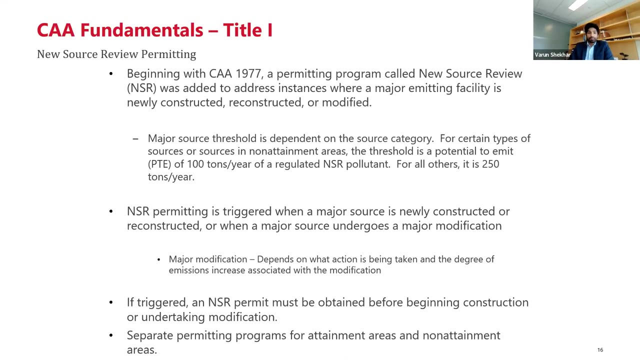 The NACs. But the NACs are separate from these standards. They're completely different statutory provisions and they address different pollutants altogether. All right, So I'm going to move on to permitting. Pam mentioned pre-construction permitting. This was a mechanism that was added to the 1977 Clean Air Act amendments. 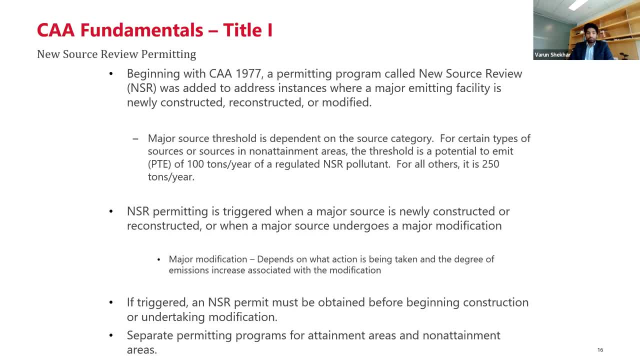 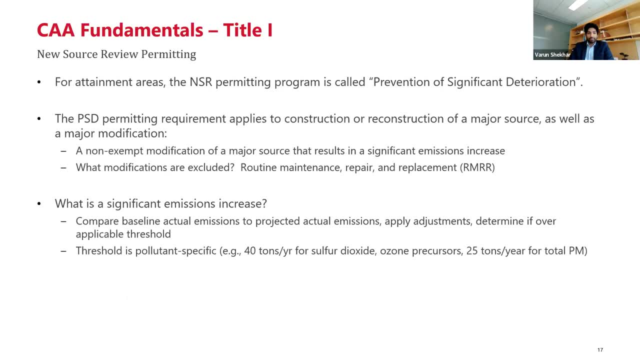 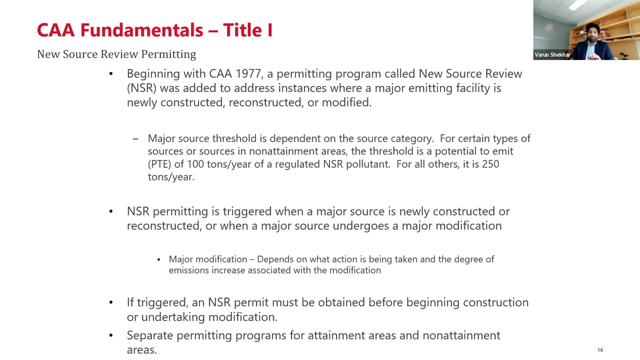 And there's two parts of it. You can have a pre-construction permitting for areas that are in attainment areas And you can have a parallel pre-construction permitting framework for areas that are in non-attainment areas, And there's a couple different levels to this. 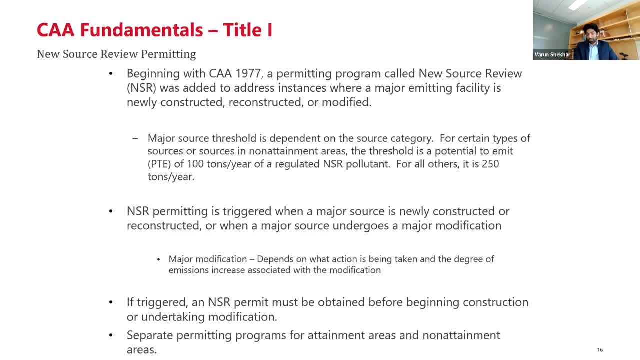 There's what is sometimes called by practitioners as MIPS. There's what is sometimes called by practitioners as minor new source review And there's something called major new source review. The Clean Air Act provisions pertain predominantly to major new source review. What is major new source review? 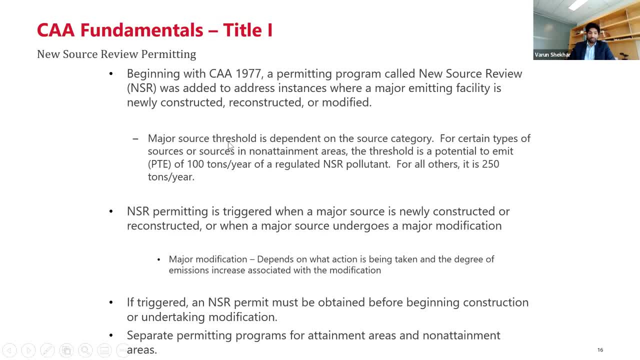 Well, it applies to sources that are classified as a major source And when they make a major modification or if it's newly constructed or reconstructed. So you have a major source or a major emitting facility if it exceeds a certain emissions threshold. What that threshold is is dependent on the source category. 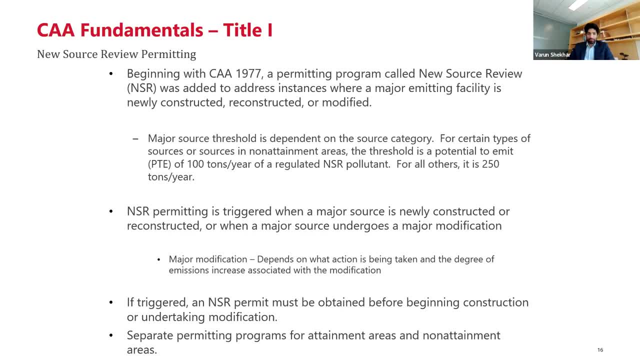 Certain source categories. it's a lower threshold of 100 tons per year of a regulated NSR pollutant. The regulated NSR pollutant can be broader than your criteria pollutants But in general there's a lot of overlap between them. For all other sources- sources in other categories- it's 250 tons per year. 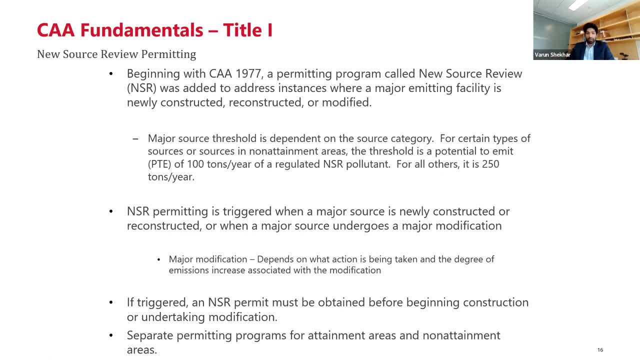 So that's the major source aspect of it. Now there's a major modification if we're talking about, you know, certainly if it's a newly constructed or reconstructed major source that will trigger a major NSR, permitting The modification is a little bit trickier. 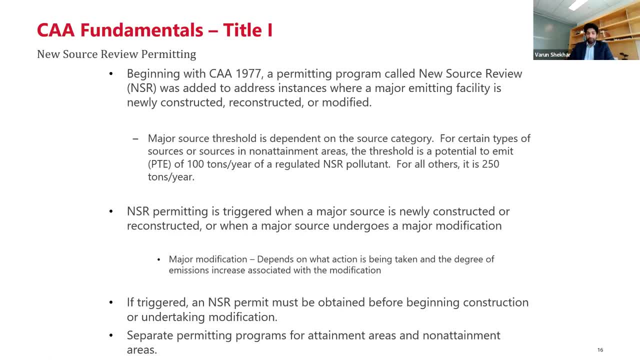 You need to rise to the level of a major modification And how do you determine that There's an emissions threshold, increased threshold that you would have to determine in order to find whether or not you've triggered this major NSR permitting The minor new source review is largely a creature of a state implementation plan. 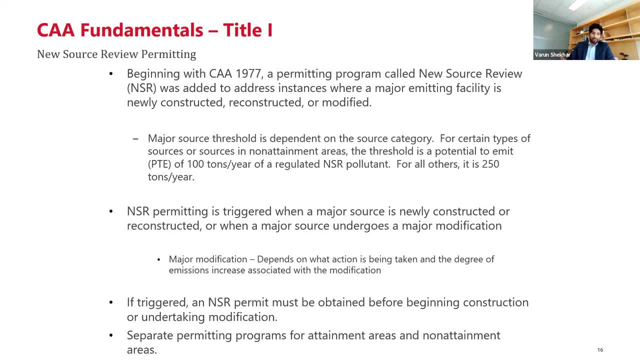 So if you have a source that doesn't you know meet the criteria I was just talking about- a major source or a major emitting facility or doing a major modification- states will still have their own pre-construction permitting requirements for that, And those are called minor new source review. 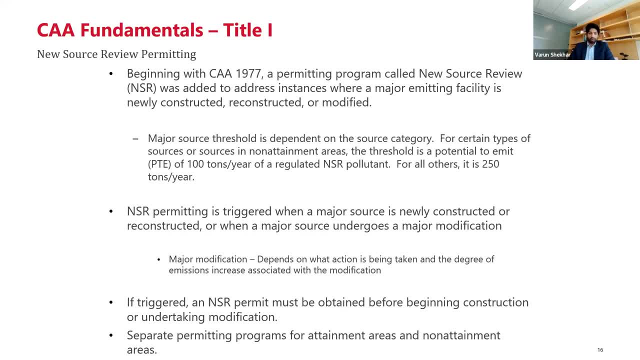 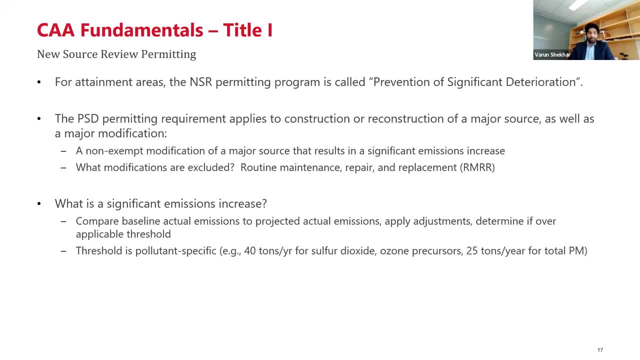 Those vary across the board But in general there's a requirement to, you know, apply for a permit before the construction takes place or the modification takes place. So I mentioned there's two kind of avenues for attainment areas. There's a new source review permitting that is called prevention of significant deterioration or PSD. 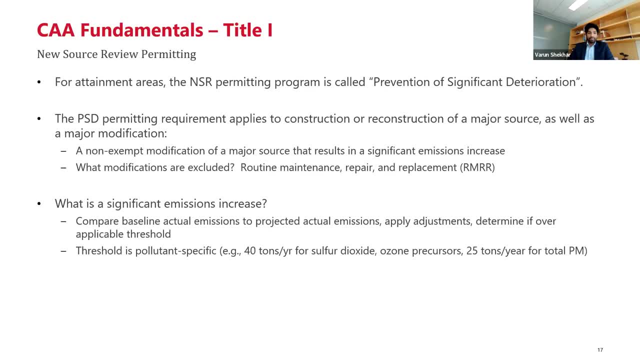 For short The PSD. permitting, as I said, is pre-construction and it applies to construction or reconstruction of major source and also a major modification. With respect to what's a modification, there are certain exclusions to that. The big one I'll highlight is something called routine maintenance, repair and replacement activities, or RMRR. 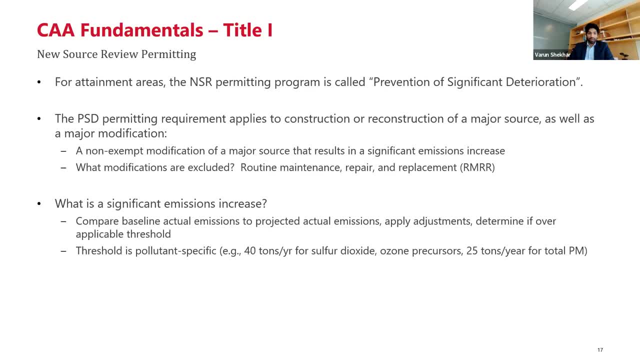 There's been a lot of litigation and fights over what that means. Right, You know? let's say you have a factory and you're replacing, you know a widget or you're changing the color. Is that a modification? Modification is defined as pretty broadly as any physical change or change in the method of operation of the source. 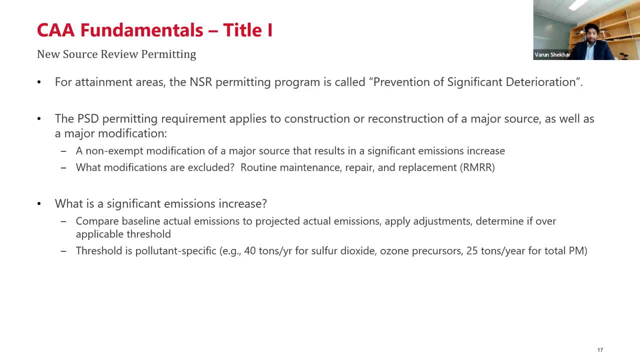 So something like that arguably could be a physical change, But does it rise to the level of a non-excluded major modification? So routine maintenance, repair, replacement, there's a bunch of factors that go into it, Things like cost, the nature of the project- if it's something where you know it's going to take years and years. 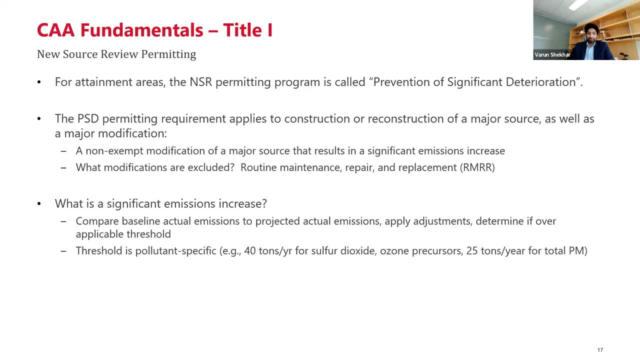 Those are factors that are considered in determining: is that routine maintenance, repair and replacement- or is it non-routine? If it's non-routine, it would count as a modification that you'd have to then go through determining: is it a major modification? 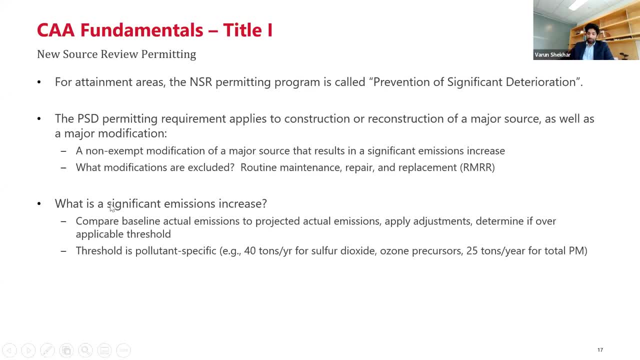 With respect to determining a major modification I mentioned, there's a certain threshold of emissions crease that qualifies it And we're talking there about for PSD purposes. there's a couple emissions tests. The test that most sources will use is called baseline emissions to projected actual emissions. 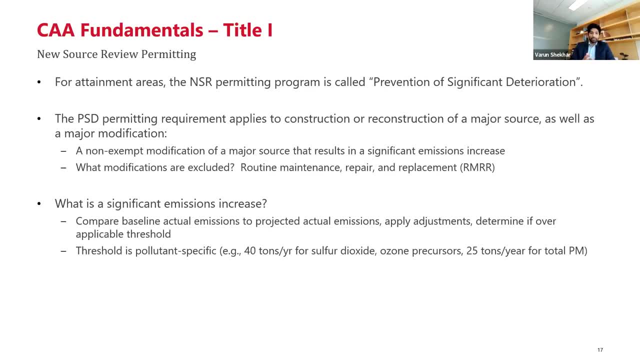 Basically, you will look at a previous number of years on an annual basis- What were the average amount of emissions? And then you compare it to. okay, once I implement that change that I want to do, what are your projected actual emissions afterward? 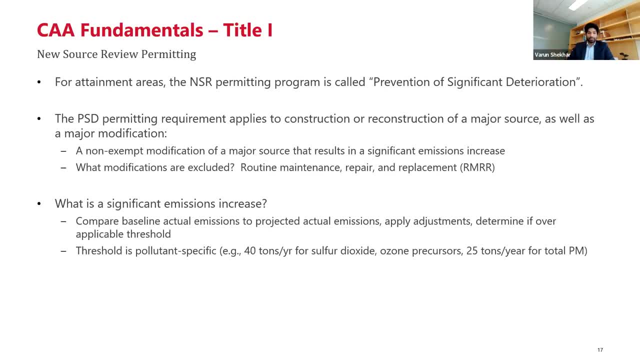 And you compare, you do a net analysis of that And if that difference is more than a certain threshold for that pollutant that's impacted by the change, then you would. it would constitute a major modification and a significant emissions increase. That threshold is pollutant specific. 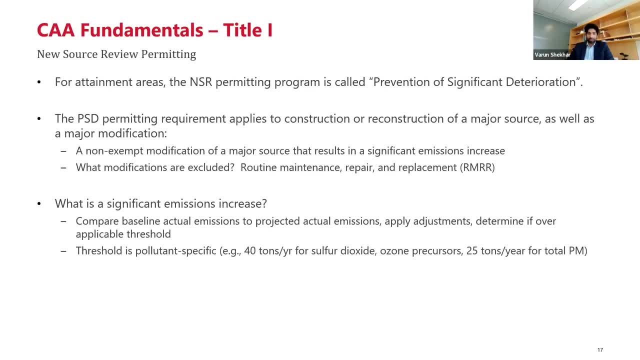 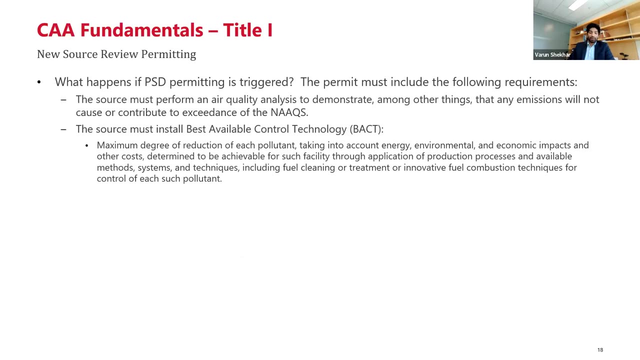 It's 40 tons per year, for example, for sulfur dioxide. It's 25 tons for PM. So that's something that you'd have to kind of go through on a pollutant by pollutant specific basis. So I talked about how do you trigger PSD, but what's the significance of PSD? 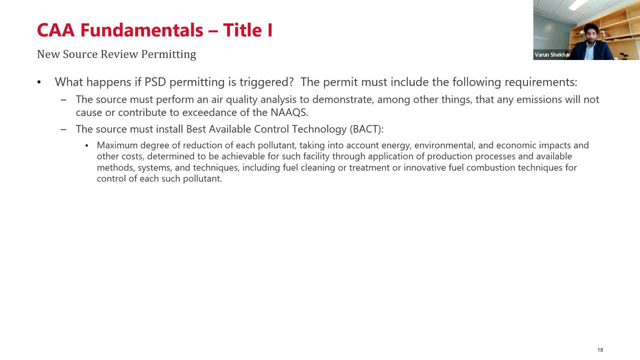 If you trigger PSD permitting and you have to get a pre-construction permit, the main things that apply are: you have to do an air quality, a detailed air quality analysis that's going to demonstrate you're not going to cause or exceed the. 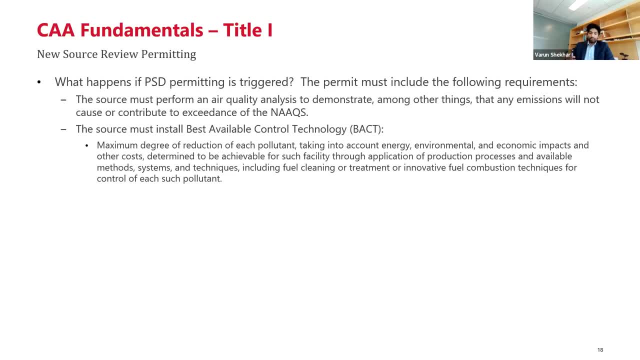 exceedance of the NACs. There's also a related concept called a PSD increment, which is, you know, even if your change is going to be within the NACs, there's a certain margin that you're sort of allowed. 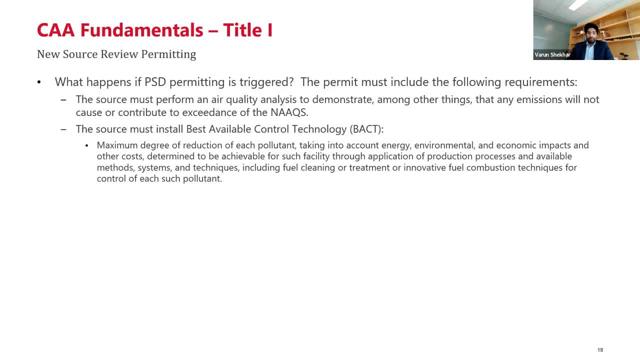 That's called the PSD increment, meaning to fall within that. The other big thing is the source would have to install best available control technology or BACT, And this can be costly for sources And that's why sources a lot of times try to do it. 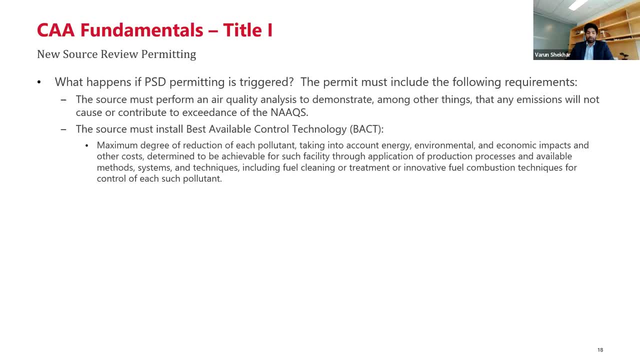 try to structure their operations or their changes or projects so that it avoids triggering. PSD. BACT is- I have the definition here- but it does take into account cost. It takes into account what's available out there in the industry. A lot of times there'll be a threshold, a cost for emissions reduction threshold. 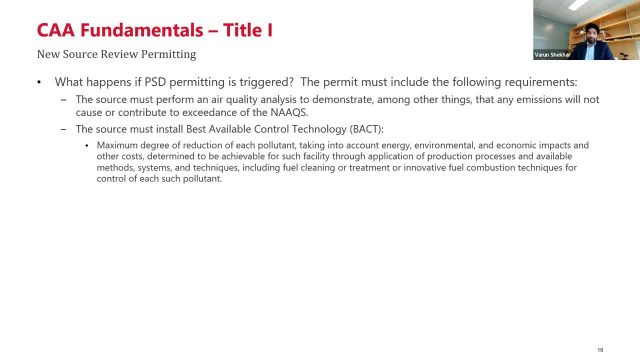 Does that qualify as BACT? To make this easier, sometimes EPA will point sources to something called a BACT clearinghouse- The BACT clearinghouse will. it's kind of a repository of what sources by category have used to implement as BACT. 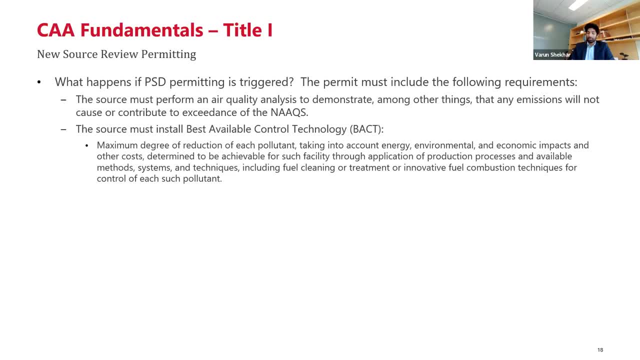 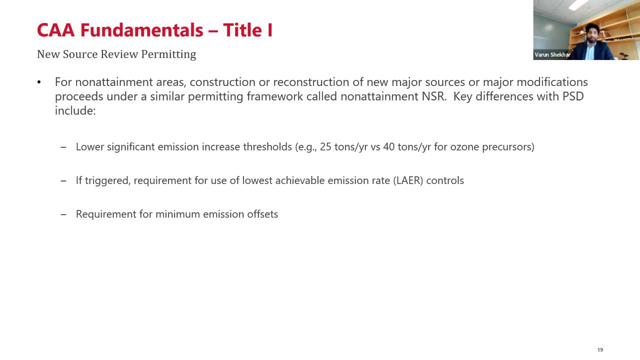 But those are the two big things And, as I said, those can be costly to a company, And so that's why a lot of times, companies will try to avoid PSD and structure it in a way that does that For non-attainment areas. 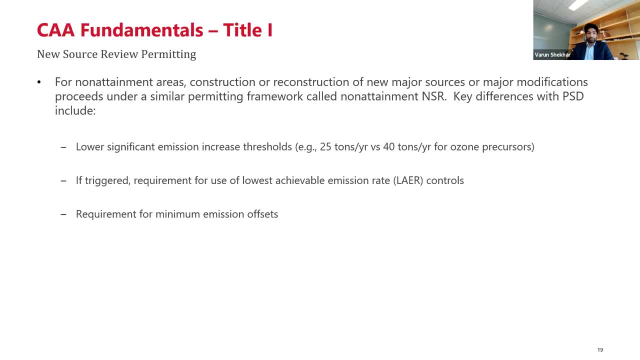 there's a parallel permitting pathway, a pre-construction permitting framework. The key differences are: in general, there's going to be lower significance for emission increases thresholds. So for example, for ozone it's 40 tons per year For PSD. 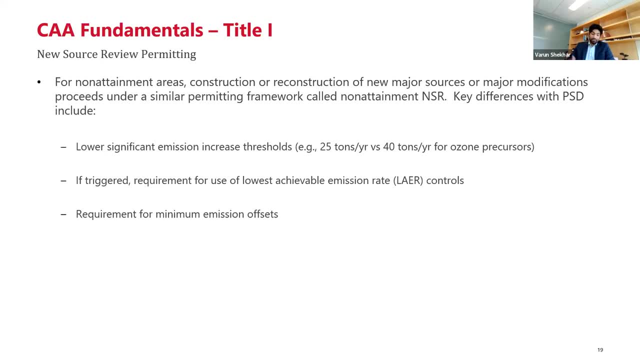 it's 25 tons per year in general, and it can be lower depending on the degree of non-attainment we're talking about. In addition, I mentioned BACT for PSD. Well, BACT on steroids is something called lowest achievable emission rate, or LARE. 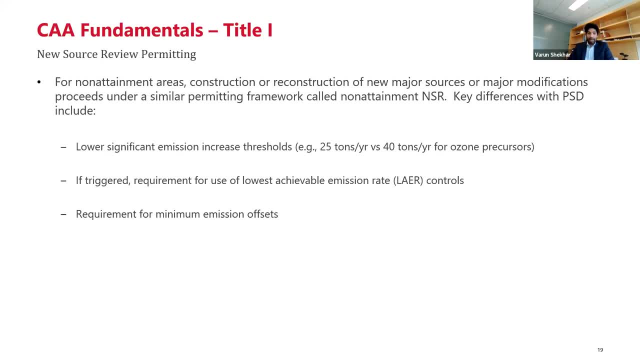 And that's even more stringent controls, less emphasis or consideration of costs and more on what sort of technology is available, And so this can be even more costly than BACT. And the last thing is, there's also a requirement for emission offsets, And so some states will. 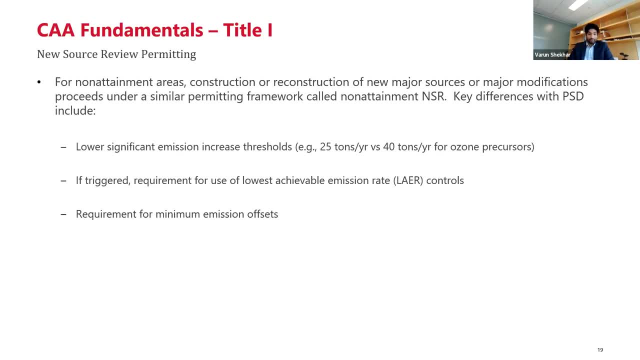 in some states it's implemented through a trading program. You have things like emission reduction credits, where you'll have, for example, a facility shuts down. they've reduced their emissions, or emissions to that state's air. There's some credits, So a lot of times there's an offset sort of framework. 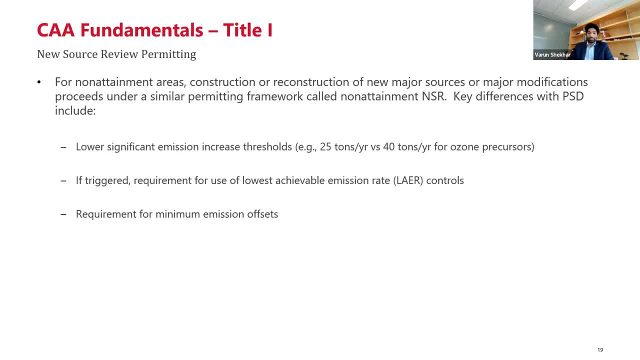 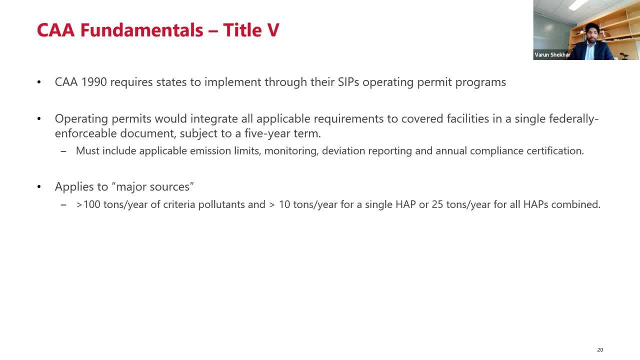 which is a trading aspect. There's a trading aspect to it which is required under non-attainment. new source review. All right, Let's try to speed things up a little bit here, but title five permitting- Pam mentioned that applies to stationary sources. 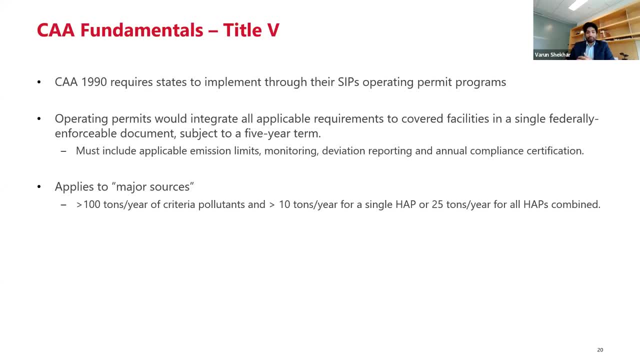 The big thing with it is it constitutes kind of an integrated permit or a permit containing all of the integrated requirements that apply to it. So this includes things from the SIP, It includes things from an NSPS or a MAC standard or NESHAP. 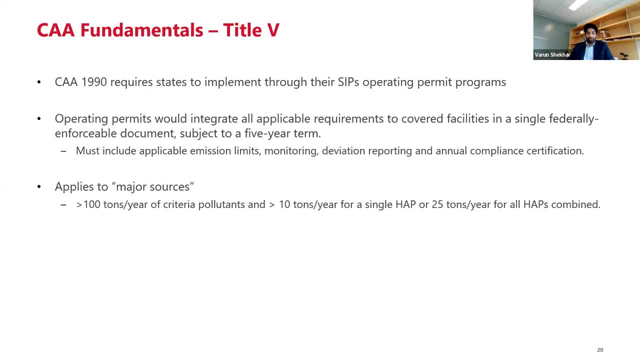 And it's a one-stop shop that a covered facility can refer to to say: okay, here's all the requirements that apply to my facility. In addition, the title five permitting provisions require annual compliance certifications as well as periodic deviation reporting. 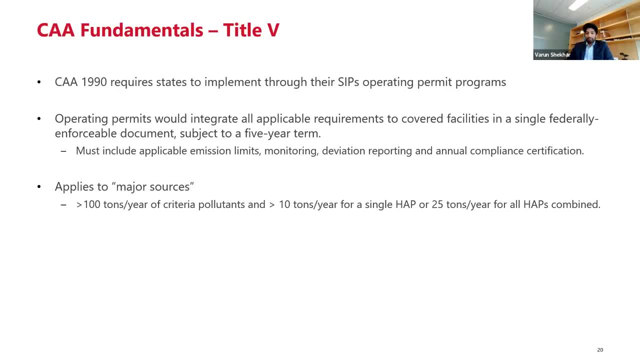 So this is important because sources have to basically do not not so much an audit, but they have to take a tally of what sort of noncompliance is out there And they go through their permit condition by condition. Am I in compliance with it or am I not in compliance? 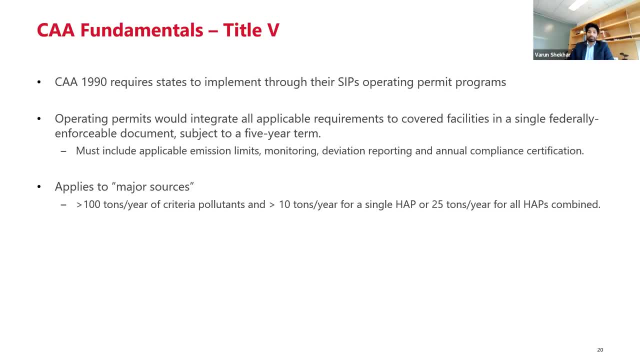 And if they're not in compliance they must report that to the agency. The title five permitting framework applies to major sources and note that this is different than the major emitting facility threshold in the NSR program. This applies. the major source for title five purposes is if you have. 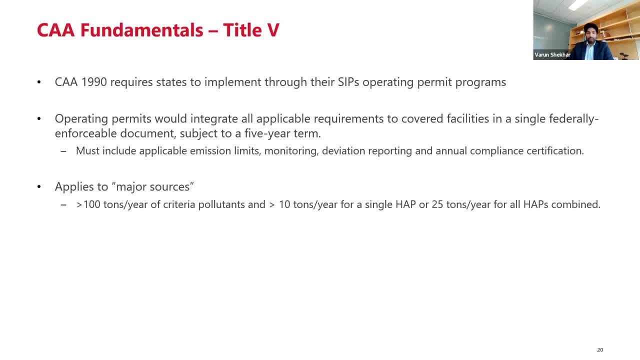 greater than a hundred tons per year of a criteria pollutant, or, or over 10 tons per year for single hazards or pollutant, or 25 for all haps combined, And so if you exceed those thresholds, you're part of the title five permitting framework. 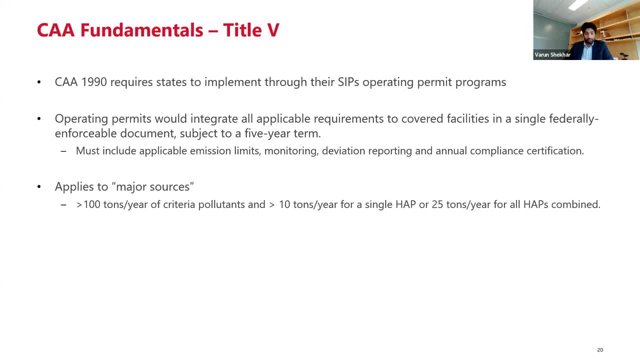 you have to apply for a title five, operating permit. So it's not just pre-construction permitting, but operating permits. And again the permits, the text of them are going to contain detailed limits or or provisions On how you operate your. 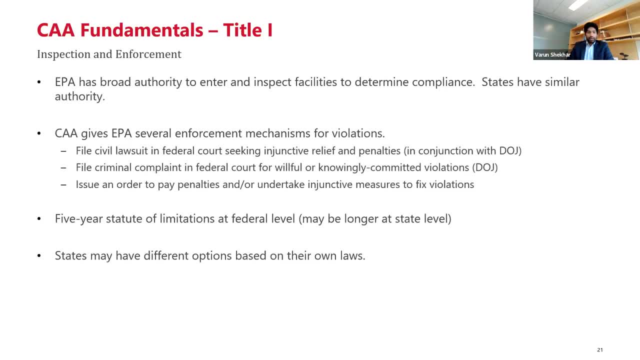 your facility. Just a couple of closing thoughts. in title one, EPA has pretty broad authority to enter and inspect facilities. They have an investigatory Avenue called information requests under section one 14. They can serve requests on facilities and the facilities have to answer. 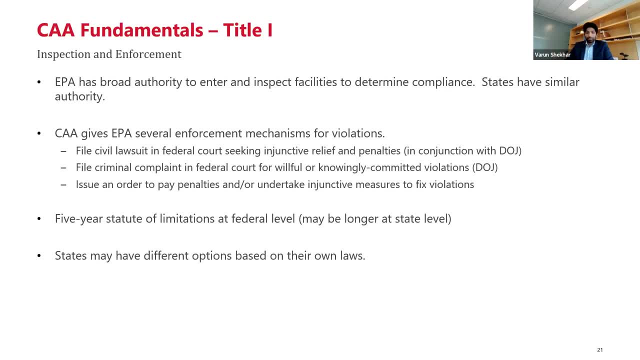 those EPA can say: you know, tell us about, what are your emissions for your emissions for this year or for this period, Tell us about. you know the nature of your, your processes, And so they have very broad inspection abilities on that front and a 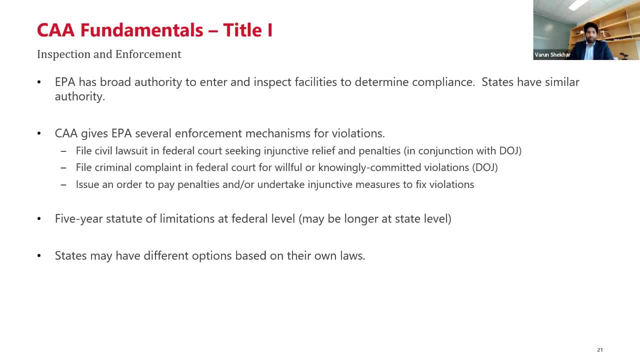 lot of tools that they have at their disposal. As far as enforcement goes, there's a few avenues that EPA can proceed under. if there's alleged violations, EPA can file a civil law lawsuit in conjunction or through DOJ, the department of justice, In federal court. 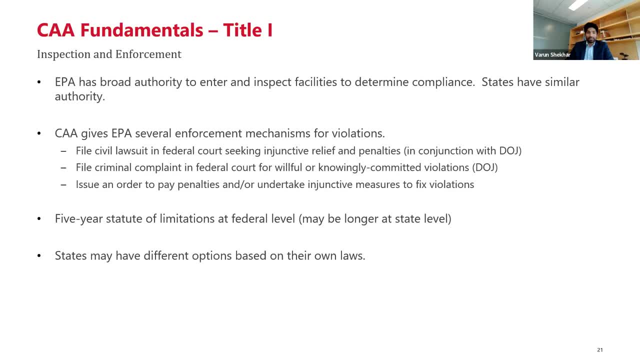 And they can seek Penalties, civil penalties. They can seek Injunctive measures. So it could be something like you know. it gets installed as control technology. That's an example of an injunctive. It can pursue an egregious cases criminal. 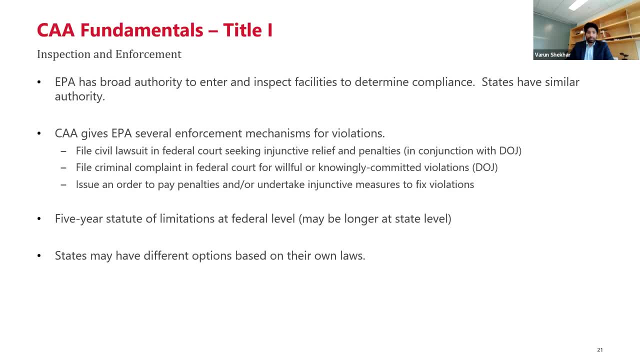 Sanctions In federal court, again through DOJ. These are typically for willful or normally committed violations, And then, finally, it can proceed administratively, So it doesn't have to actually go to court. That has the authority under the clean air act to issue an order to. 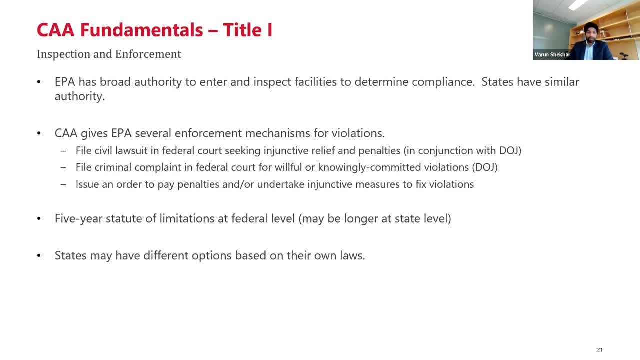 pay penalties, Civil penalties, or it can Also issue an order for the facility to undertake Again some of these injunctive measures. A lot of the times these are under consent. So you know the the, the EPA will issue a notice of violation or finding a violation. 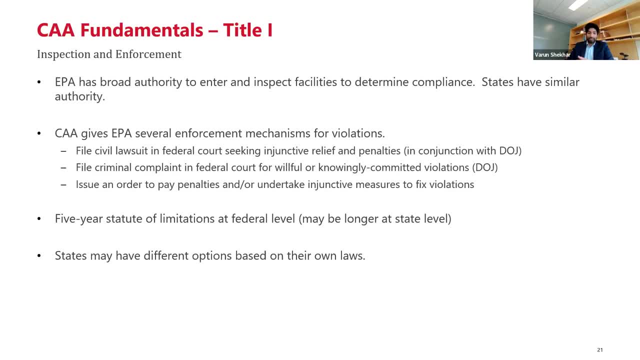 The parties will confer And then, rather than you know, deciding to go to litigation, they'll say: let's, let's resolve this Administrative Lee, and These orders that will require these aspects are done through A consent, on a consent basis. 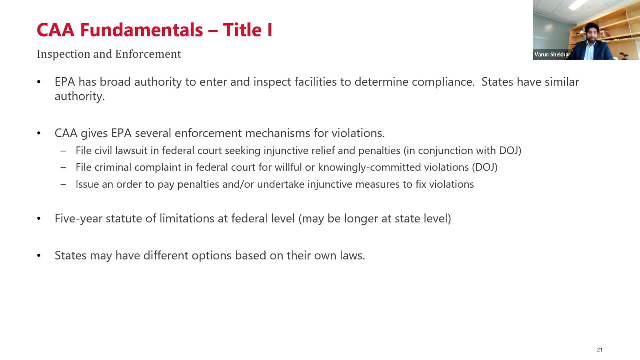 There is a five-year statute of limitations. This isn't in the cleaner act itself, It's in a more general statute, Federal claims. But keep in mind that there are parallel paths of enforcement here. The state enforces its state laws. EPA. 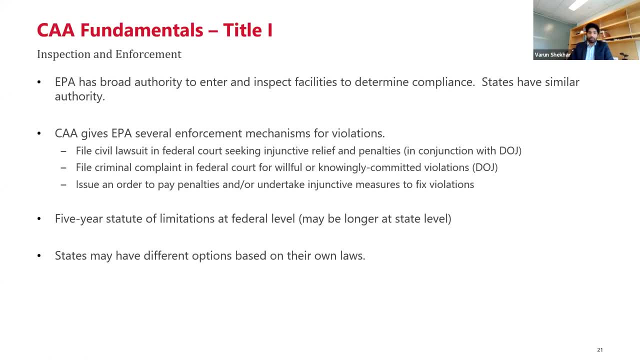 Enforces the SIP, which is incorporated into the federal law, And so you know EPA. you could be subject to enforcement by EPA And or the states as well, And the states when they're enforcing their own kind of state regulations. 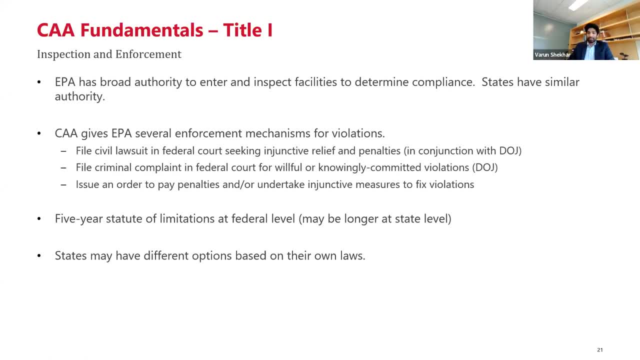 The statute of limitations. It depends on the state I'm very familiar with, for example Pennsylvania. I do a lot of my work there. They have a seven year statute of limitations. And then a last thing on enforcement is citizen suits. 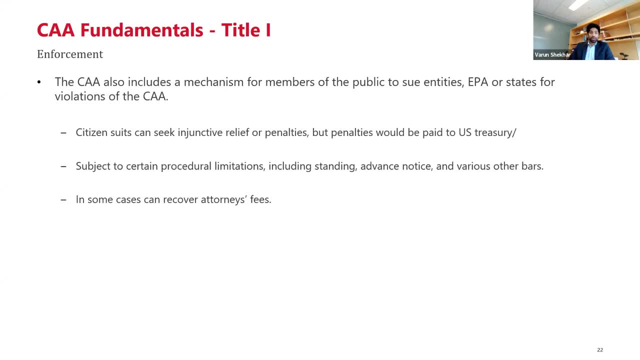 So enforcement doesn't have to only proceed through a public agency. Members of the public can also bring suit, And they can sue not only companies, but they can sue states or EPA for violations of the cleaner act. And the remedy is that are available are similar to what's available. 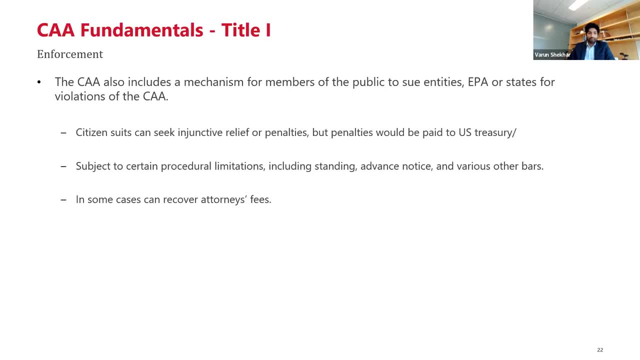 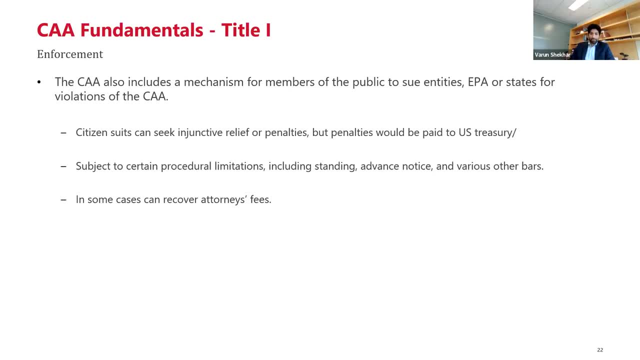 They don't get the penalties themselves. They don't get the penalties themselves. That goes to the U S treasury. But there may be other avenues for them to recover. In some cases they can recover attorneys fees And there's a certain standard to ship to get those. 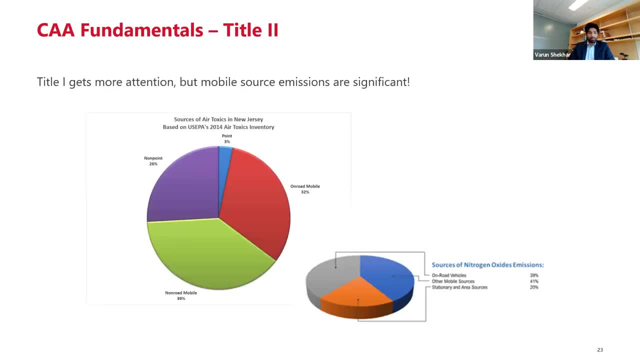 All right, real quick, Cause I'm a little running, a little long, but real quick. I want to make a mention of title two, which is mobile sources. Title one, which is stationary sources stuff Gets a lot more attention, but mobile source emissions are really. 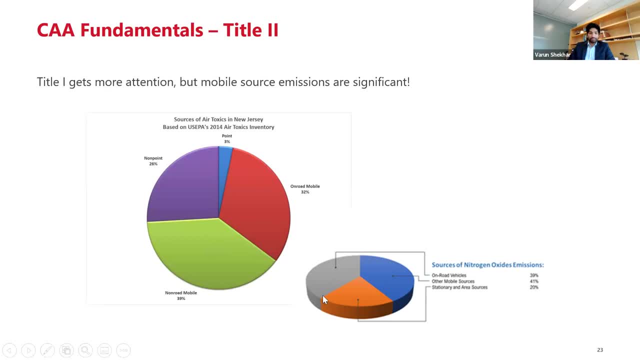 really significant when it comes to air quality. I have a couple of graphs here. One is from New Jersey And the green part of this pie chart is non-road mobile sources. The red part is General other on-road mobile sources. So things like, you know, cars and trucks. 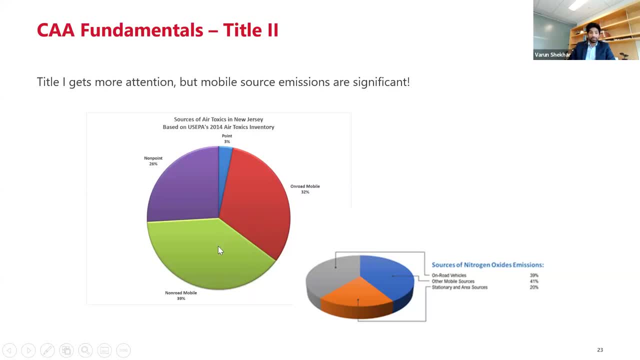 And that becomes, for the majority of Emissions of at least air, toxic in the, in this case To the ambient air, With respect to nitrogen oxide, Which is a precursor to ozone, As I mentioned earlier. This is, I believe, from California. 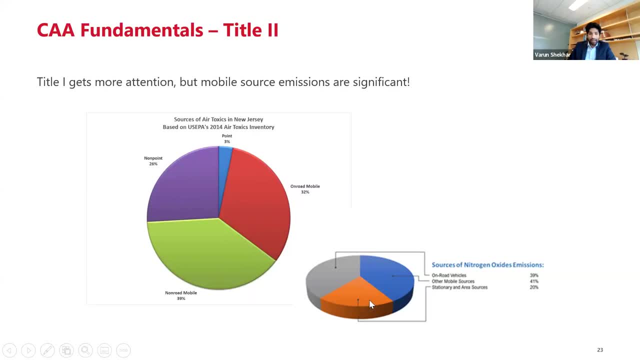 In the bottom right pie chart And the combination of the blue And the gray are mobile source emissions of Knox. So again, the majority of it is coming from mobile sources. So you can't truly appreciate Air quality. and how to you know? Solve issues with air quality without also regulating mobile sources. I think this helps explain to some extent Why New Jersey and California Have such so many exceedances in national Air quality standard. A lot of it is mobile sources, And especially when they're idling installed and they're not moving. 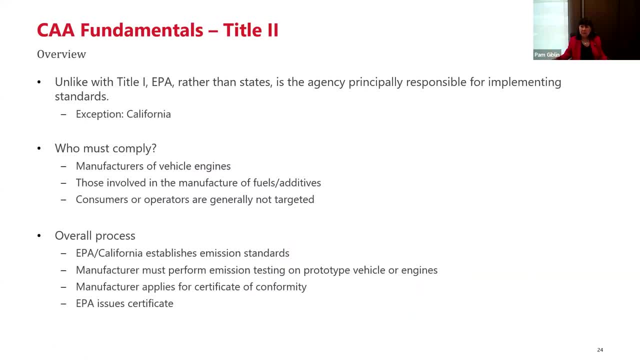 rapidly. As you know, that could exacerbate the problem. So I think that that sort of shed some light on The anomalies that people were seeing In those two states. Absolutely, And California, You know California- is one of those states where 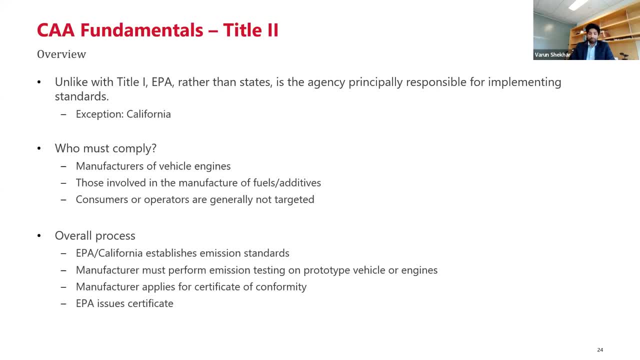 You know California well, especially Southern California, known For its high volume of vehicular traffic. I think, combined with its kind of valleys and its meet geography, Can They have very large contributions of not from to a non-attainment standpoint from mobile sources. 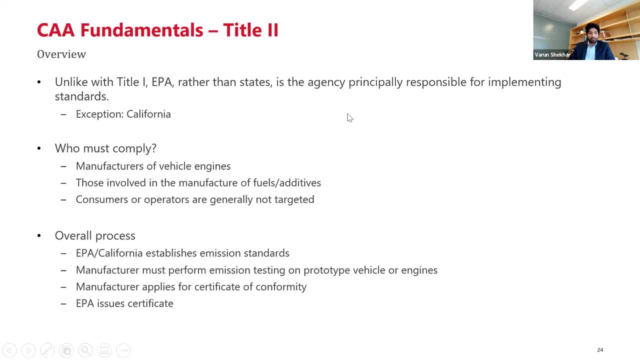 So I'm just going to kind of Real quickly skim through this. I was hoping to get into a little more detail, but So when we're talking about regulation under title two, it's a little bit different than title one I mentioned with title one and stationary sources. 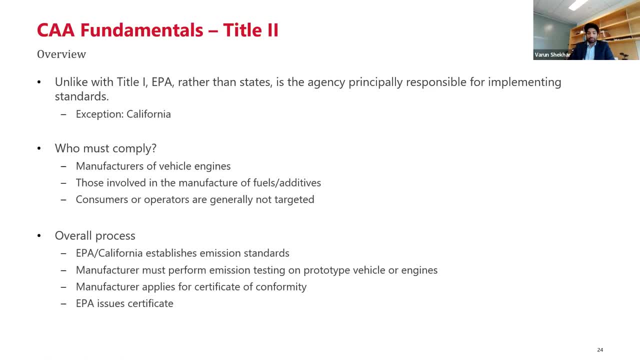 This cooperative federalism approach. States are in many respects the driver of Of air pollution regulation. It's a little bit different on the on the mobile source side. EPA is for mobile sources, The principal driver of standards, And the standards aren't imposed on the operators. 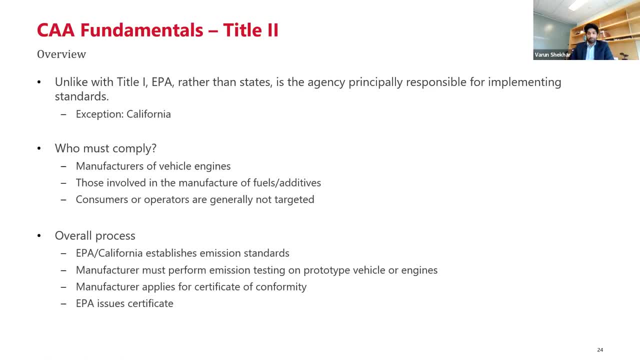 Or the owners of sources like they are On title one for title one. Rather, the standards predominantly apply to Manufacturers of vehicle engines As well as manufacturers of fuels or additives. So you know, if you know, if you have a car, and it's kind of. 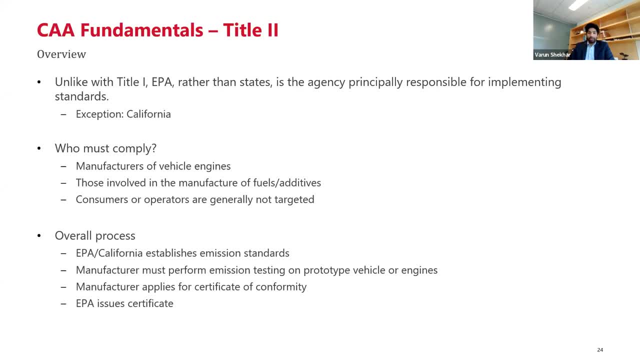 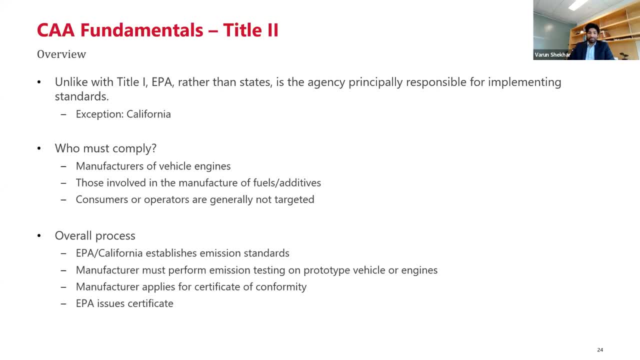 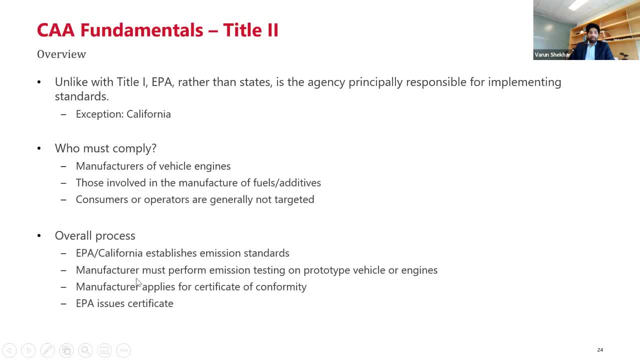 How does the regulatory process look like? Well, EPA- And to some extent California- We'll talk about in a second- Establishes a mission, standards, prototype vehicles or engines And, once it does the testing, it submits it to EPA, who will review. 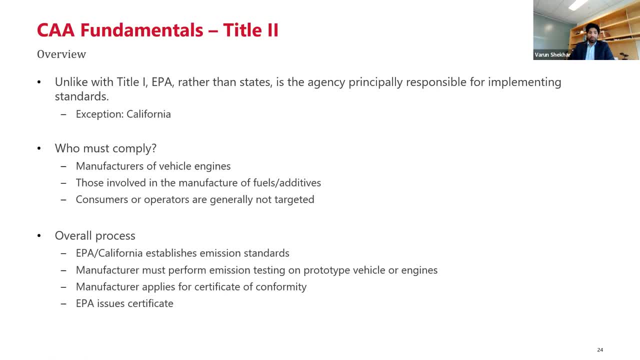 it. Sometimes EPA does its own testing And then EPA will issue a certificate of conformity with the emission standards upon application from the manufacturer. So each car out there, at least since the enactment of Title II, is supposed to have a certificate of conformity. There's 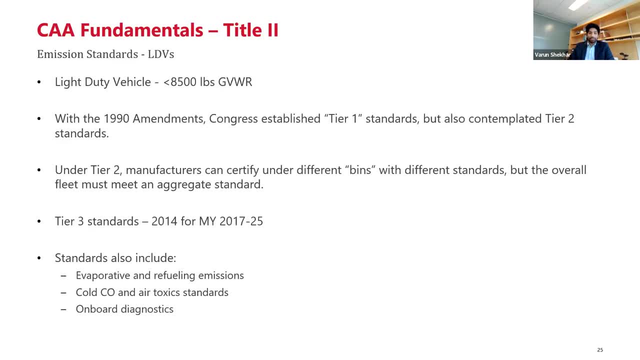 limited exemptions, but in general each engine needs to have a certificate of conformity. There are light-duty vehicles and heavy-duty vehicles. Light-duty vehicles are kind of the passenger cars and trucks. There's a weight threshold that I have here And the thing I'll 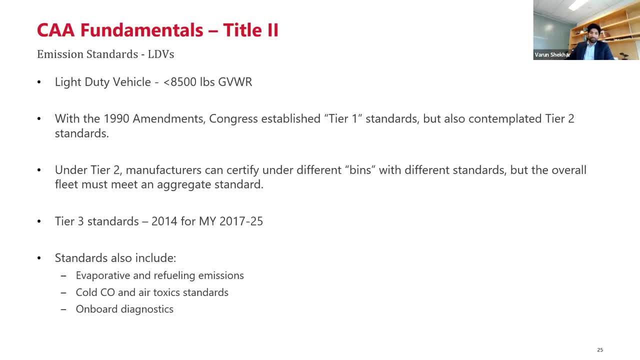 point out here is there's been various iterations of standards. They're called tier standards: Tier 1, Tier 2, Tier 3.. We have new standards that have been proposed in April, which pertain to not only the emission standards but also the emission standards, And so there's a lot of. 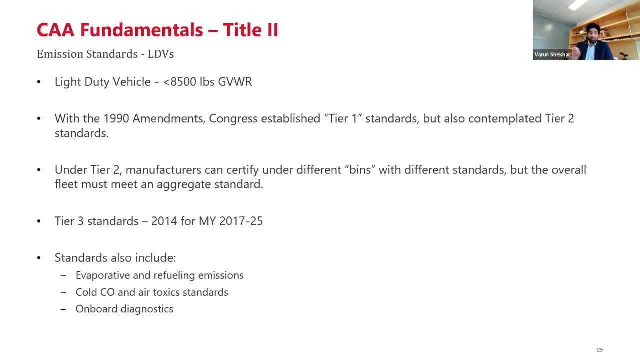 criteria-like air pollutants. They're a little bit different on the Title II side but for all intents and purposes they kind of match up nicely. But there's also in the most recent proposed rule standards for greenhouse gases. They got this mainly from California, which they did at the 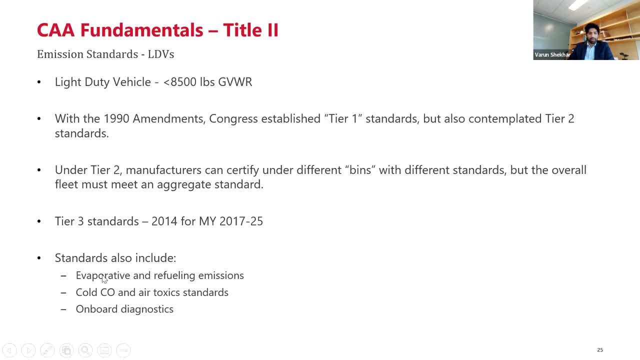 state level. There's also standards for other things other than just these sort of criteria. air pollutants: There's standards on evaporative emissions. You just park your car outside. it's going to have some losses from the fuel and those are emissions into the ambient air, And so 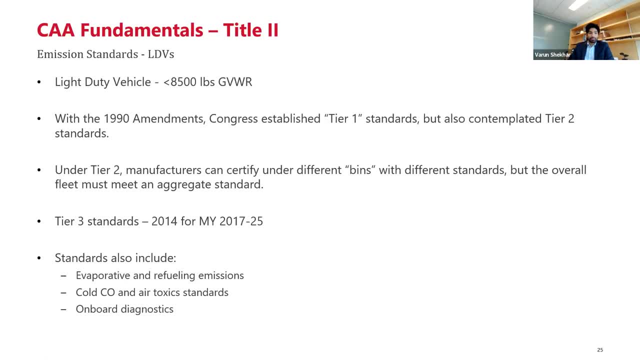 there's standards on that for cars. There's other standards for onboard diagnostics. So if you have an engine or an emission control equipment in the engine that has failed, there's requirements for cars after certain years to have diagnostics that will alert the user. hey, this is not working. 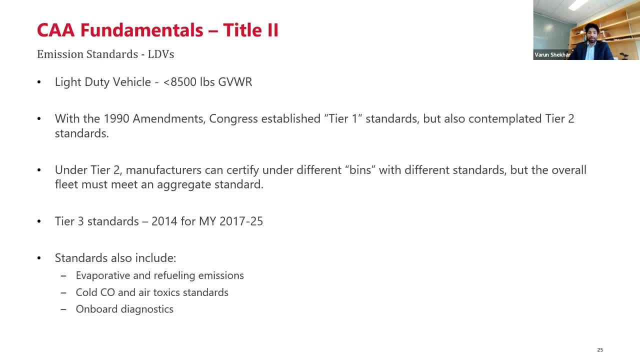 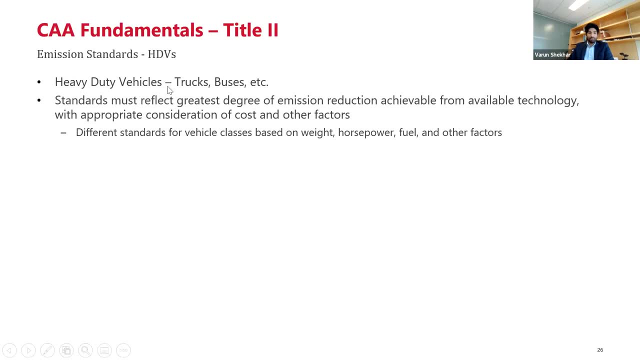 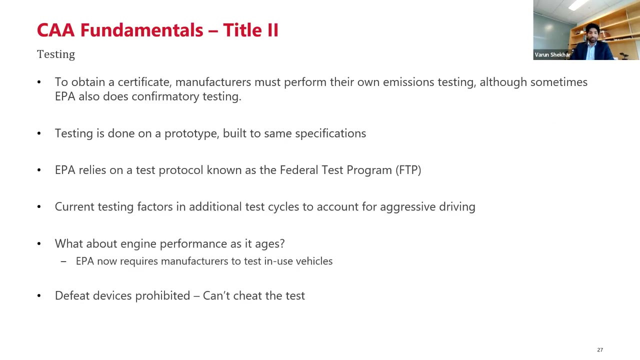 right and so that it promotes getting those things fixed in a timely fashion. Similar standards for heavy-duty vehicles, things like trucks and buses, and there's a hodgepodge of standards depending on the weight and the horsepower nature of the engine. The testing aspect, as I mentioned: the manufacturers do a test. 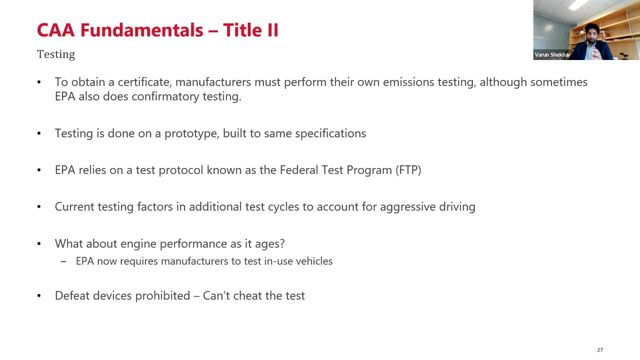 There's a certain protocol that they have to follow when doing the test, and this is important because if you test it at certain standards that aren't reflective of how the car is or the vehicle is normally driven or operated, you're going to not have a true test. So if you test it, 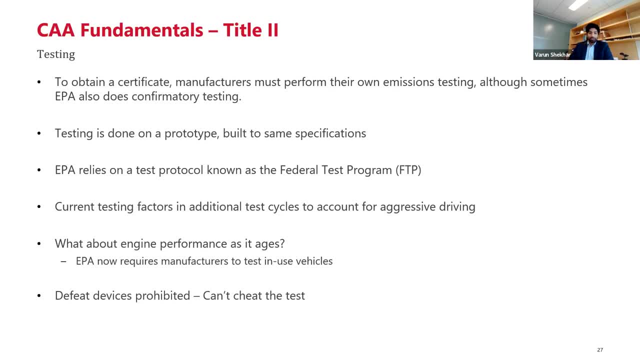 at certain standards, you're going to not have a true representation of what those emissions actually look like, and from an air quality standpoint that's obviously untenable. And so the thing to note here is there's a kind of a centralized test, federal test program that 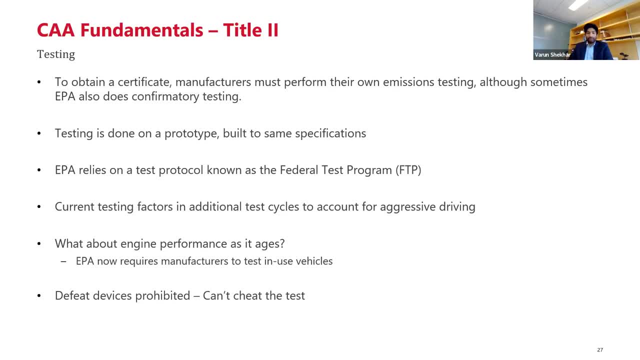 EPA promulgates It, revises it over the years depending on driving habits. In the early years it was a very kind of steady state sort of framework which was not reflective. They've thrown in additional test cycles for aggressive driving. you know starts. 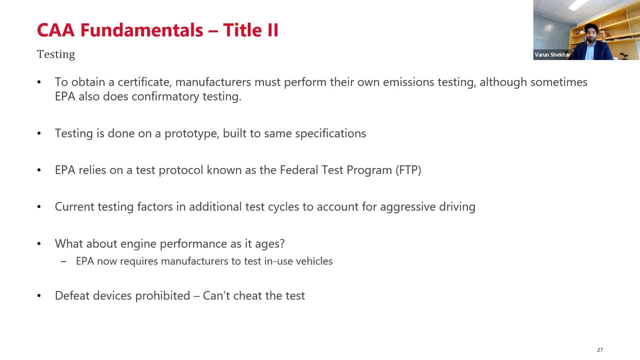 aggressive starts and stops. Also, you know various operational conditions like weather, And the other aspect of testing is that engines can age and if you test it when it's brand new, you may not get the same result if you test it three years in. So EPA also requires manufacturing. 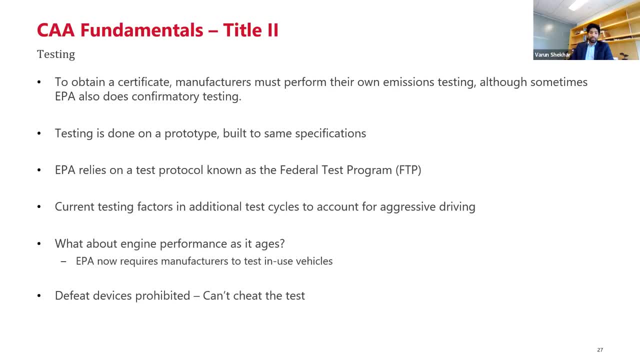 test in-use vehicles after a certain number of years. I'll also mention at the end an enforcement case with VW. but But you can't cheat the test. You can't put in devices that when you're testing it, you suppress emissions and then, when you're not testing, you remove it or stop operation of that. 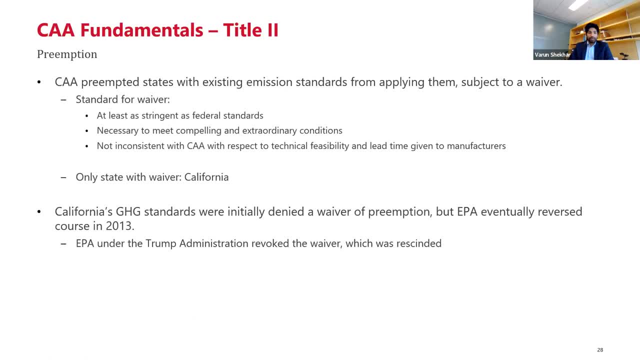 control and then you have a larger amount of emissions. Preemption- important part of Title II. the Clean Air Act- generally preempt states from imposing their own emission standards on mobile sources. There is an avenue for a waiver from that and California has it. California waiver had to meet certain requirements. The three elements are up here at the top. They have to be at least as stringent as federal standards. They have to meet compelling and extraordinary conditions and also has to be consistent with the Clean Air Act as far as technical feasibility and lead times. 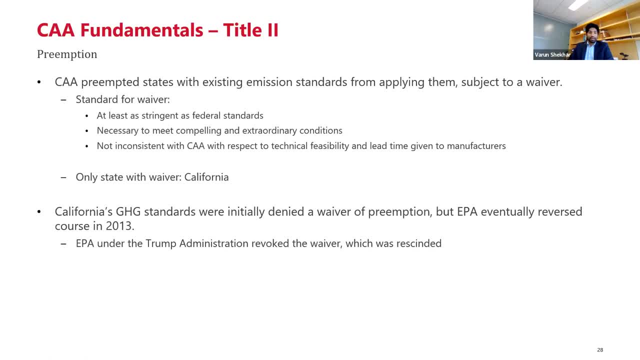 that are given to manufacturers. as far as the compliance schedule goes, The waiver can be on a item-specific basis. So you know, California has standards for the various sort of criteria- pollutants, as I mentioned, but they also have standards on greenhouse gas. They initially got. 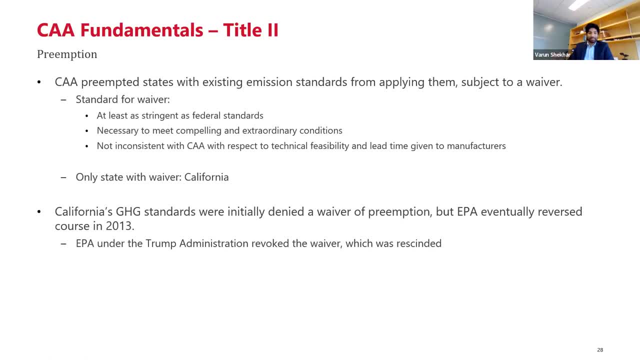 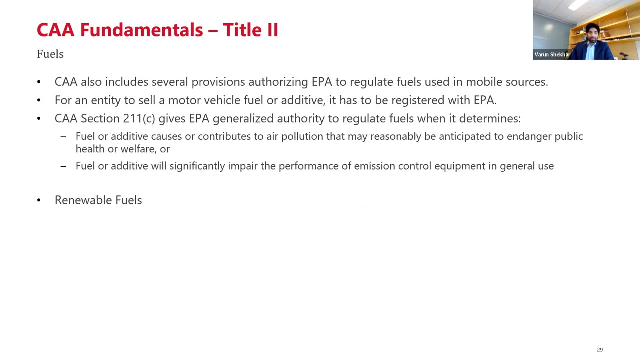 a waiver, but there's a back and forth about that. So ultimately, the EPA currently has reinstated their waiver for greenhouse gas standards. There's also a fuel component. Title II regulates the manufacturing of greenhouse gas. So you know there's a lot of information about the 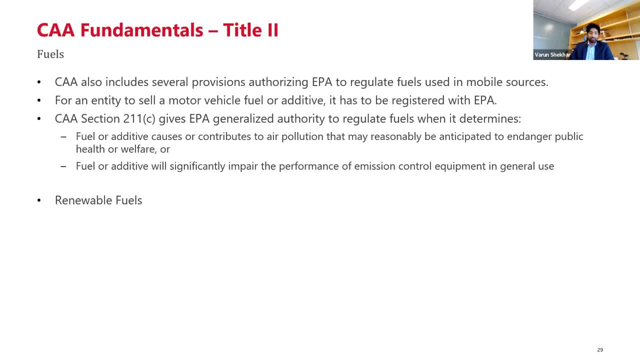 manufacturer of fuels. Manufacturers have to regulate- I'm sorry, register emissions of fuels when they are manufacturing a new one, And there's a lot of demonstration that goes into the registration process. There's a testing aspect: Is it performing as it should? There's a 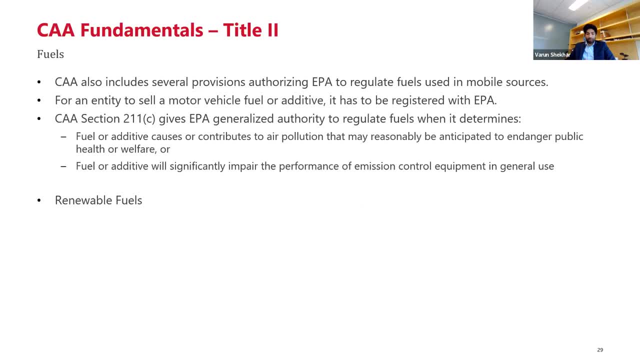 baseline fuel that serves as a reference, And then when you have a target fuel that's introduced to the market, they have to show that the performance is at least comparable or better. The other thing I'll make reference to is renewable fuels. This was enacted through 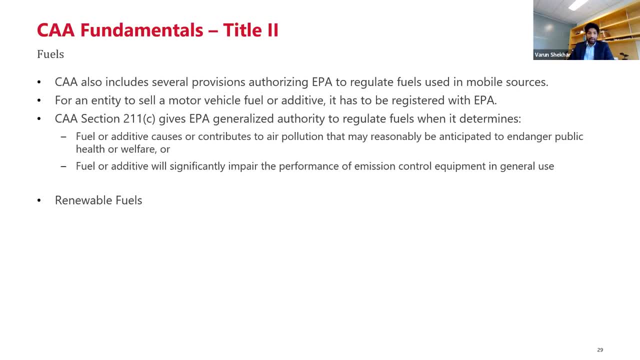 2005 legislation called the Energy Policy Act, And basically where we're at with that is there are requirements for fuels sold in the United States- at least a certain percentage of them- to incorporate renewable components to it, And so you know, when you fill up, you might see. 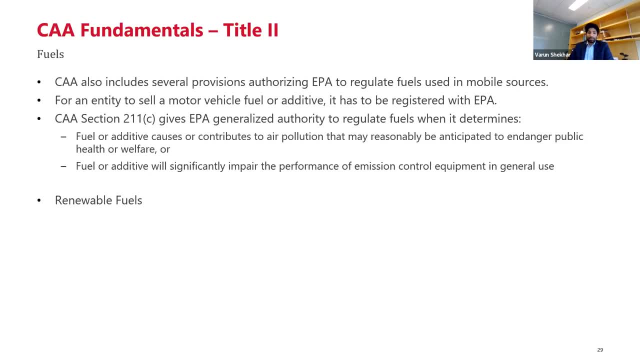 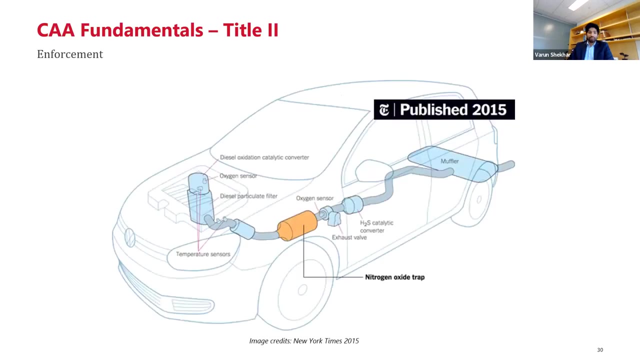 something like, you know, 10% ethanol. That was largely a product of this legislation where we're trying to- not just you know, we're trying to introduce newer, more renewable kind of sustainable fuels as part of that, And so there's going to be an increasing amount of renewable. 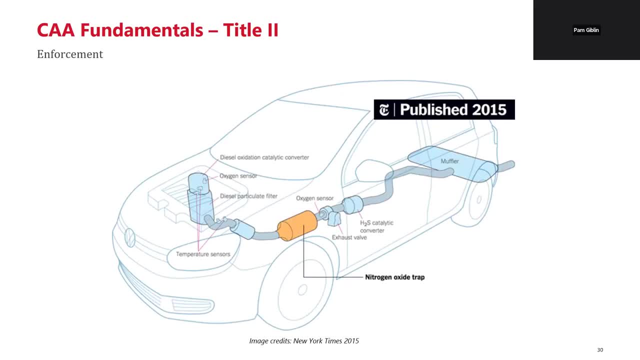 components to fuels that are on market. The last thing I'll talk about is enforcement under Title II, Pretty similar to Title I, similar sort of remedies available to EPA. I'm going to bring up the case of Volkswagen because we've got a lot of headlines. a few years ago, What happened there was Volkswagen. 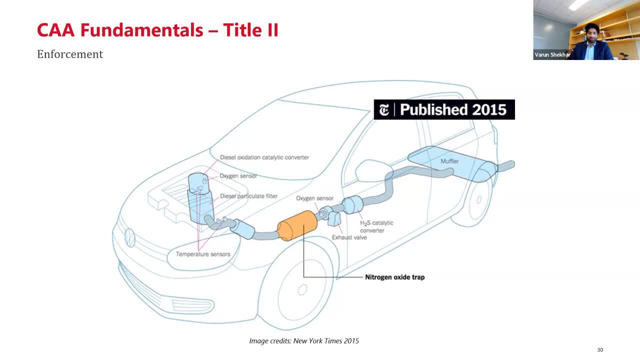 well, there was a university that did some testing on Volkswagen vehicles and they were getting unusually high results from its diesel vehicles, And so it was reported to EPA. EPA looked at it further And what was found was that Volkswagen- and, keep in mind, these vehicles- are very 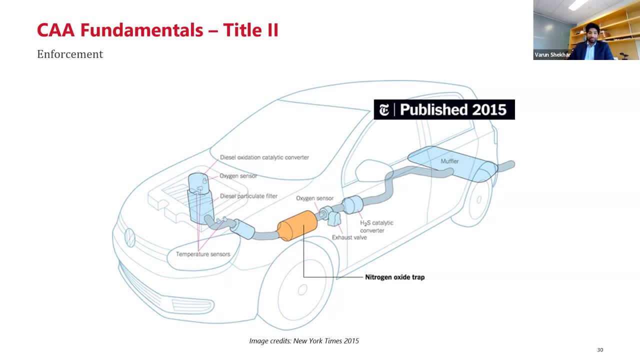 computerized these days and they're very sophisticated. EPA programmed the engine components that it would be able to recognize when a test was being done- emissions test was being done- And it would go into a different operating mode And then 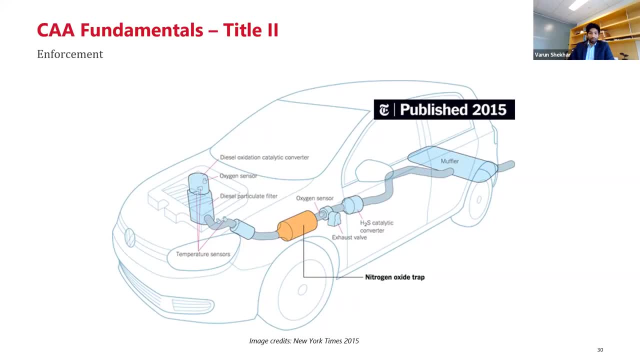 when the vehicle detected that the testing was no longer being performed, it reverted back to a different operating mode which had higher emissions, And the reason why it did that was because there were some benefits to being able to claim a higher fuel economy and a better fuel economy, And so this sort of setup was deemed by EPA to be a defeat device. 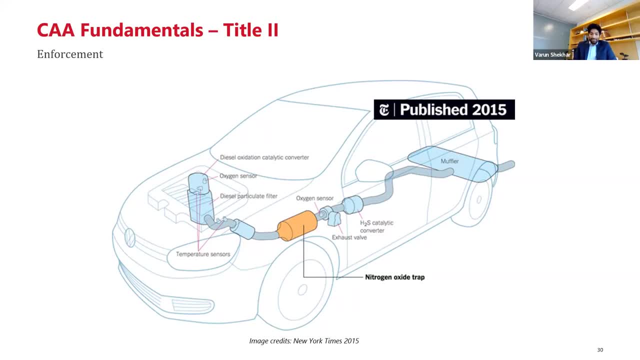 They cheated the test by going into this sort of phantom standalone testing-only mode, which suppressed the emissions that were recorded during the test. Volkswagen was hit very hard. They culminated in a $14 billion settlement. They had a number of other sort of sanctions that were imposed on them: restrictions on how many vehicles it could sell. 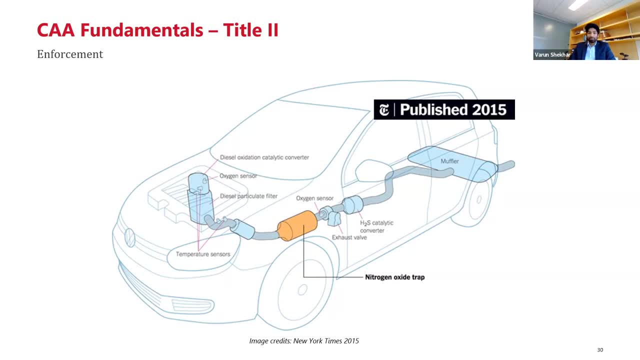 They had to recall all of its diesel vehicles to fix it- Very costly for Volkswagen. It also culminated in criminal sanctions too. They were charged with conspiracy to defraud the federal government in violating the Clean Air Act. They pleaded guilty and there was another very 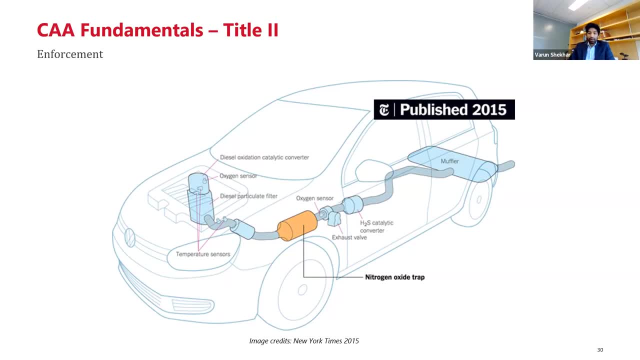 substantial criminal penalty that was imposed on top of it. So an example of willful, knowing violations that rose that were egregious enough to rise to the level of criminal sanctions. Criminal sanctions are pretty rare under both Title I and Title II, but they occur every now. 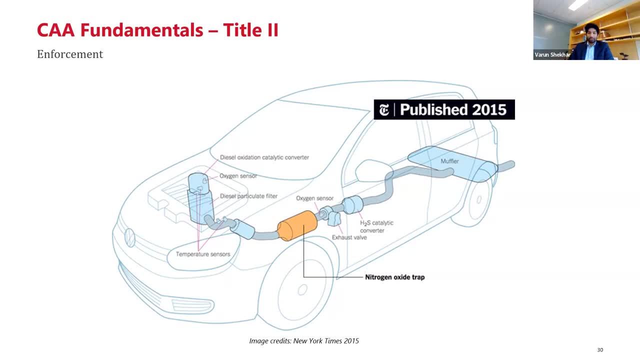 and then. But it's important to note that if you're advising a facility or representing a facility, you're not counsel them to knowingly or willingly violate the Clean Air Act, because there are dire consequences that can come out of that. So that's a very high level overview of the Clean 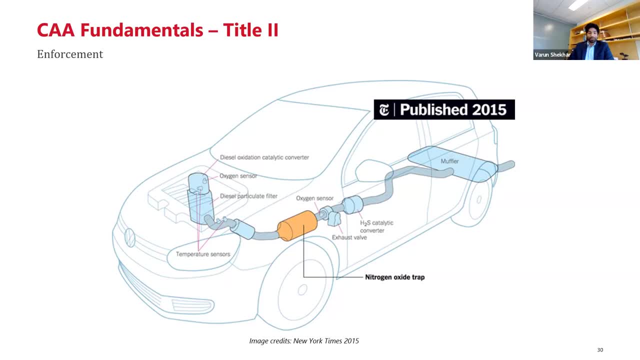 Air Act. You can practice For decades and still, you know, as I said, learn new things about it. But I hope to provide some of the tools that are kind of provided to EPA and other entities under the Clean Air Act statute. 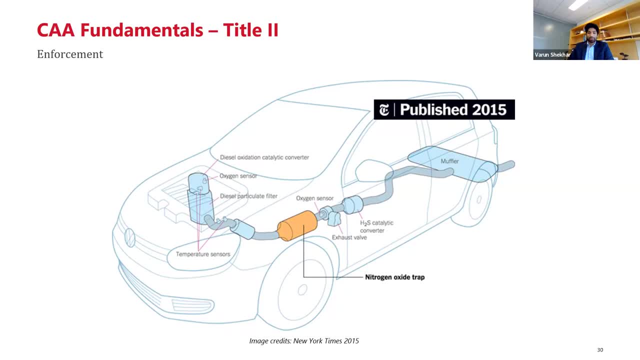 And I'm going to turn it over to Jay to talk about some specific issues, namely climate change and how some of these provisions I talked about have been applied in those contexts. Thanks, Varun. Yeah, that's exactly right. We have a really good setup now as to kind of how the Clean Air Act works. 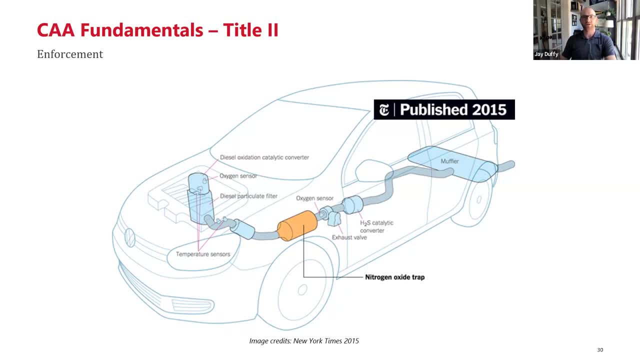 to then think about how climate change has fit into it and, in some cases, not fit into it. I'm going to request control Varun. I've also been going through the questions and answers and answering what I can if you want to hop in there, And I think there will be a little bit of time. 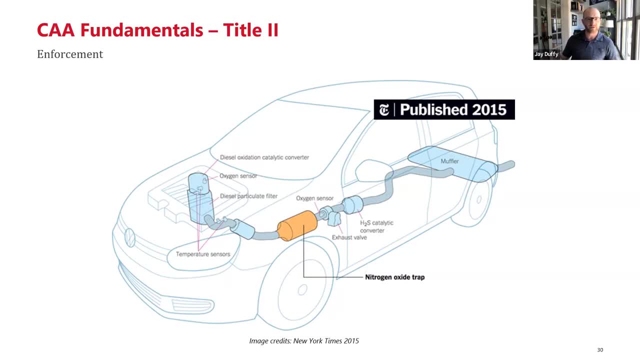 left at the end here, but it might not be as much as we had anticipated, So feel free to put things in the question and answer. We'll answer those as we go, And also the contact information. One of the things ELI has always been great about is telling people. 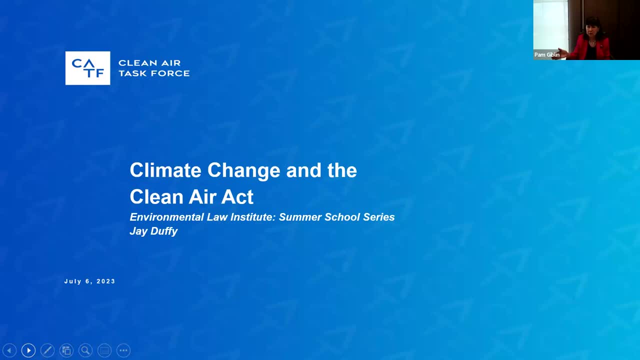 feel free to contact some of the speakers if you have follow-on questions at some point. Yes, absolutely. I think both Varun and I are happy to take questions if we don't get to yours, but we'll try and answer things in the Q&A there. So good afternoon, You know. as Pam mentioned, 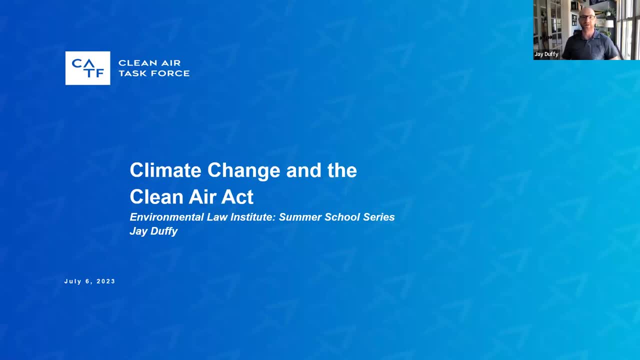 earlier. my name is Jay Duffy. I am the litigation director at Clean Air Task Force. We're Boston-based, but a global environmental NGO focused particularly on climate change, So I graduated from Villanova Law School in 2010.. That was just after the Waxman-Markey bill failed. 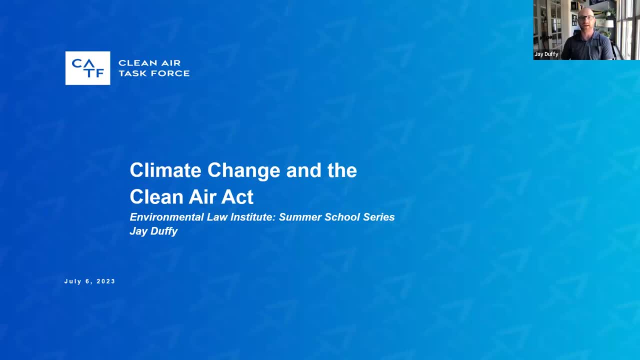 Its full name was the American Clean Energy and Security Act, And what it would have done is establish an economy-wide cap-and-trade system. It would have capped greenhouse gas emissions and allowed companies to buy and sell their energy, And it would have allowed companies to buy and sell. 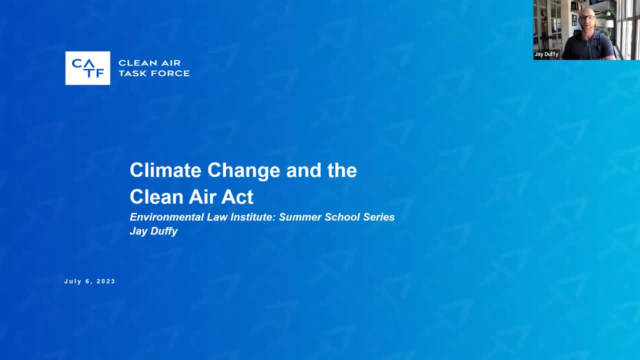 them with a cap that was declining over time. So it passed the House on June 26, 2009 by a really slim margin, but the Republicans in the Senate threatened to filibuster and the bill never made it to a vote. So this is kind of all happening as I was in school And with those prospects gone. 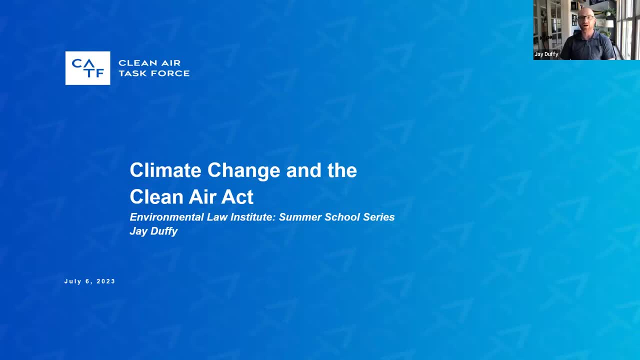 folks started looking to existing laws to regulate. you know the ballooning greenhouse gas emissions And you know there's a lot of things that are going on right now that are going to be a threat to the environment. you know threats of climate change And, as Pam, kind of 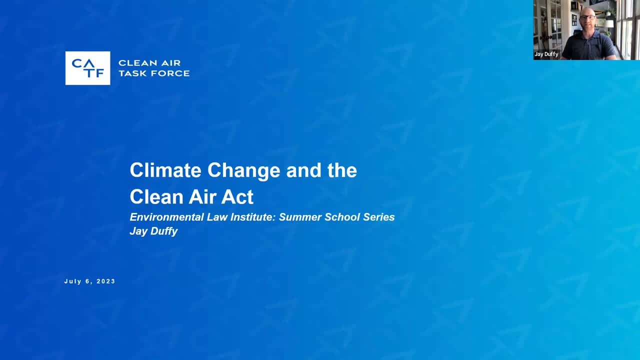 mentioned at the outset, the Clean Air Act is a flexible and broadly written statute that can encompass, you know, emerging problems, different sources of pollution, different pollutants. So I was on the Villanova Environmental Law Journal and I was, you know, reviewing article. 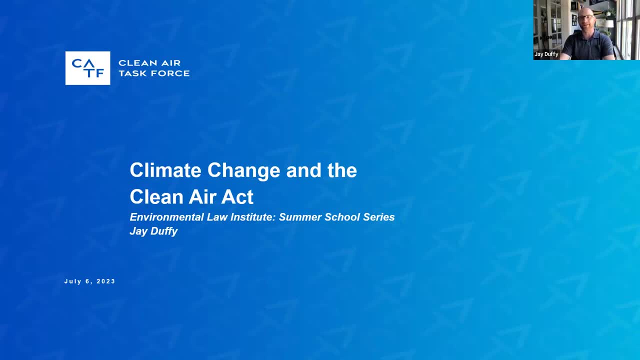 after article of people trying to figure out: okay, the Waxman-Markey bill failed And I was looking at different sections of the Clean Air Act. Should it be a NAX? Should we look at section 115 that Varun mentioned, which is the interboundary international transboundary? 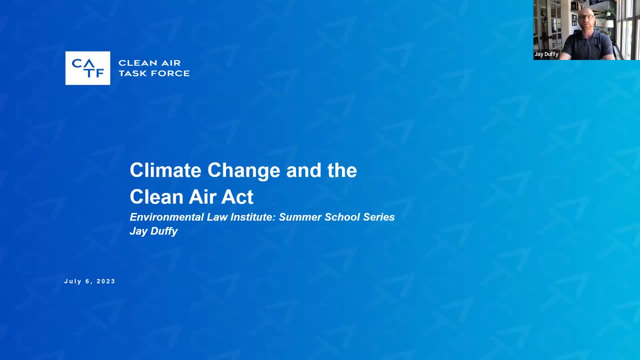 pollutant regulations, public nuisance law folks were looking at. So it was a really kind of exciting time And it's very rare in law- although it's becoming more happening more and more often- that we're at kind of the beginning. 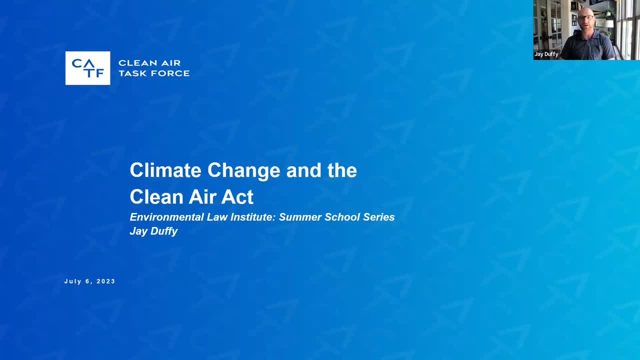 of something but the beginning of an issue, And so it's what I've dedicated my career since then to. I worked. I worked on permitting the new infrastructure associated with fracking in Pennsylvania during the Marcellus shale boom at Clean Air Council in Philly, after law school. 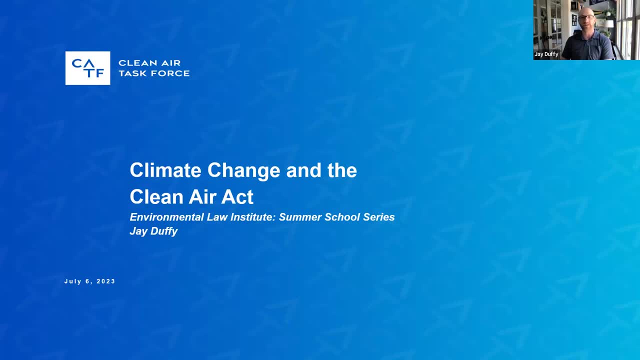 and then made my way over to Clean Air Task Force in 2013,, where I've been working for the past 10 years trying to get greenhouse gas emission standards for power plants across the finish line, And more recently I've been- I've been focusing more so on greenhouse gas emission standards for the 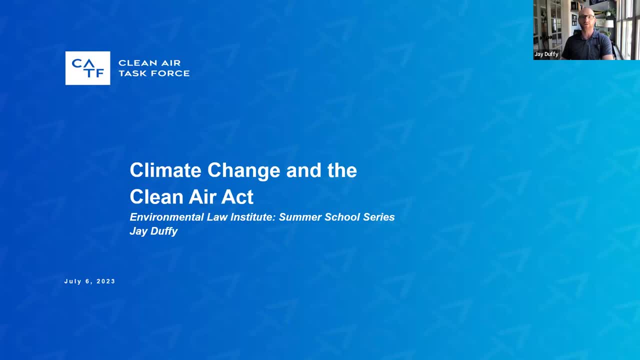 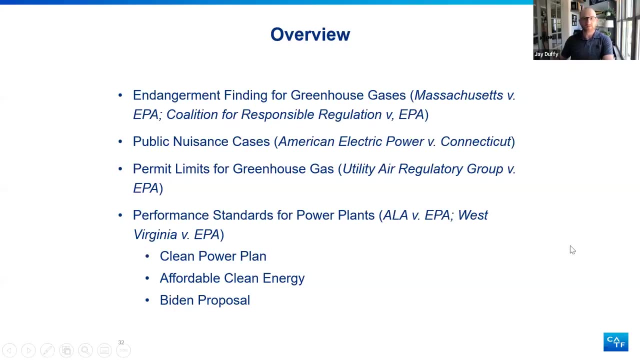 transportation sector And I have colleagues who focus on methane emission reductions from the oil and gas sector. All right, so we'll go on to our slides here. There we are. So, as a kind of intro here, what we'll be going over: we'll look at the path to the prerequisite finding for regulating pollution under 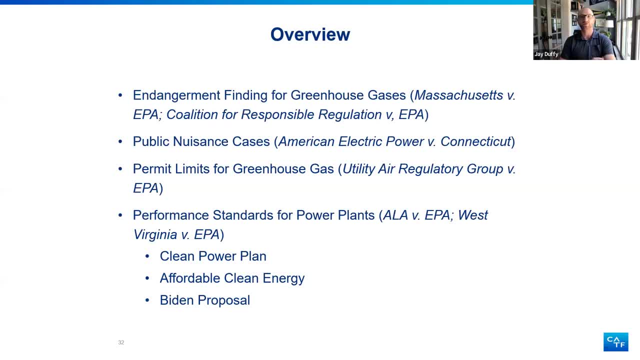 several of the Clean Air Act sections, And then we'll talk briefly about the, the failed attempt to use public nuisance law to get carbon emission limits on power plants and what that ended up meaning for the Clean Air Act. We'll look at EPA's attempt to fit greenhouse gases into the permitting structure that Varun went over. 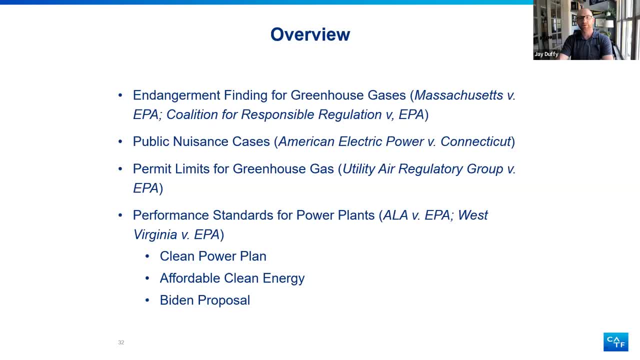 for individual sources and how that teed up what's called the major questions doctrine. that has become very prevalent in climate change law, in in things dealing with the pandemic, and has been been more, more top of mind at the Supreme Court lately. Then we'll we'll spend some time, spend most of the time on these three attempts to set the floor standards, the new and existing. 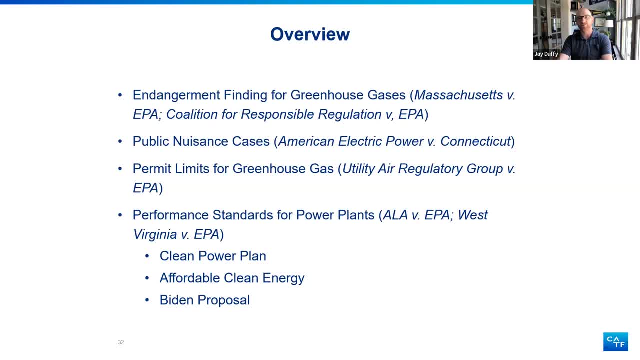 standards for power plants for their CO2 emissions under Section 111 of the Clean Air Act. As I said, I kind of thought I'd be able to cover a bit more, but even just this was a was complicated enough for for my full full time. 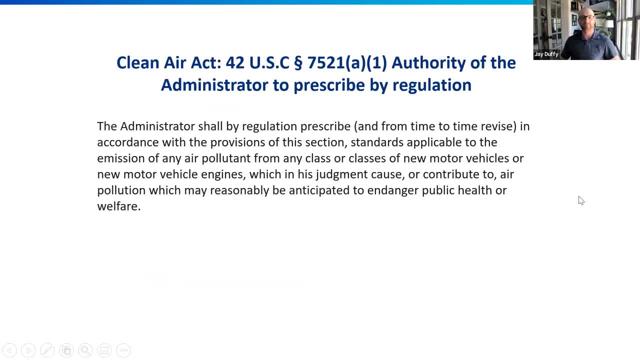 All right. so, as Pam mentioned, it's really important to get comfortable with these statutes and the relevant sections. that's that's kind of where it all begins. sometimes the case law is really exciting, the, the, you know, the policies are really exciting, but where it all begins is is with the statute. so 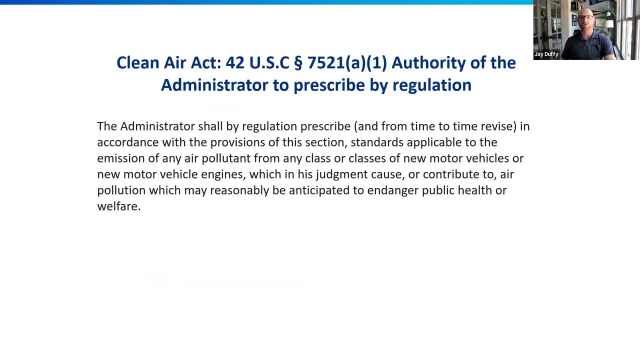 as we go through this discussed congress, you know, wrote the clean air act and delegated to epa multiple different jobs in order to ensure that all dangerous pollution- um, you know criteria- pollutants, hazardous pollutants, ones that don't fit into either of those um, as well as a um, a nax kind of backstop to ensure. 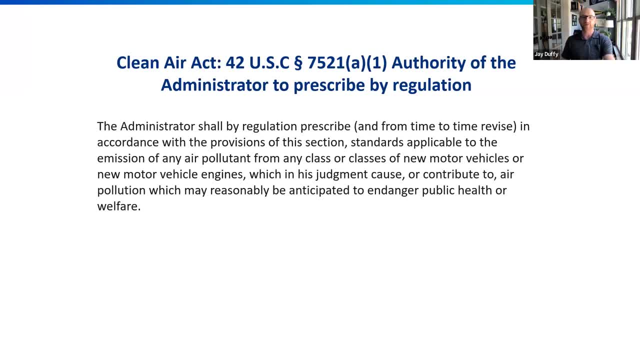 that that air quality is um meets, meets public health standards, so that those are all um those, all those multiple jobs uh have been assigned to epa and to ensure that we kind of have overlapping um uh provisions to ensure that we have have healthy air. so the first attempt to regulate: 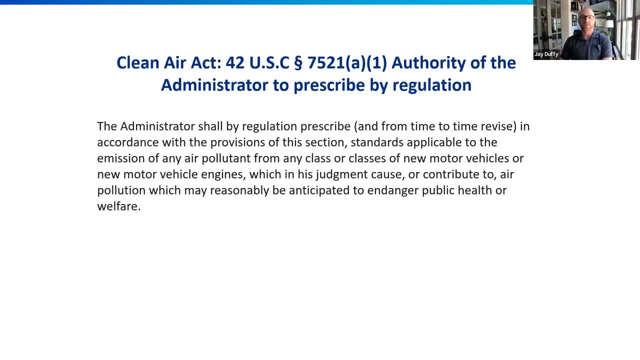 greenhouse gases under the clean air act was under uh started with section 202 a1 of the act, and this is under title 2, that that which regulates mobile sources- um, it instructs the epa administrator to prescribe standards applicable to emission of again, and this is, this is the uh- um any air. 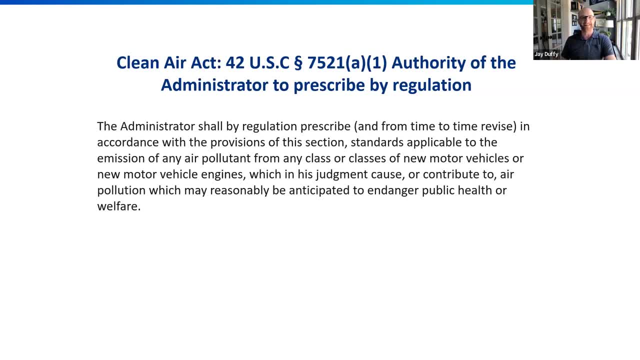 pollutant. um, and what does an air pollutant mean? it means anything right, as varun went through, but any air pollutant which causes or contributes to dangerous air pollution. while this particular finding is the prerequisite for standards for vehicles, once that finding is made, that you know greenhouse gases are dangerous and and harm public health and has implications, 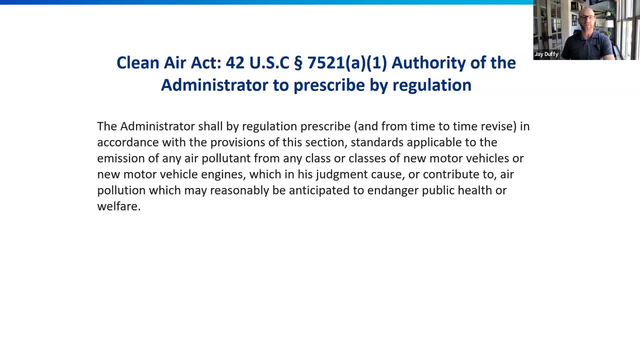 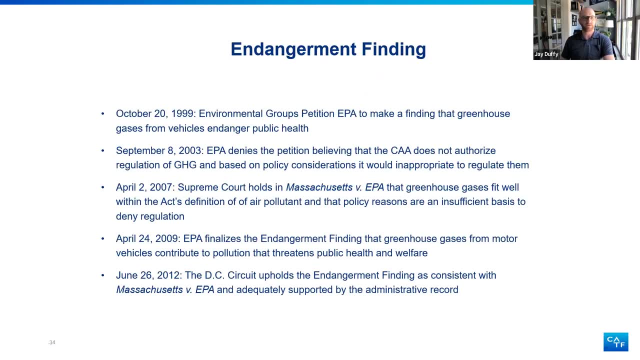 for um, the rest of uh for many other sections of the clean air act, all right. so the endangerment for um greenhouse gases comes from not only the their VISTAs who socialize, but the public living community as well, which means ouruz friends and our community are my friends. i always joke that. 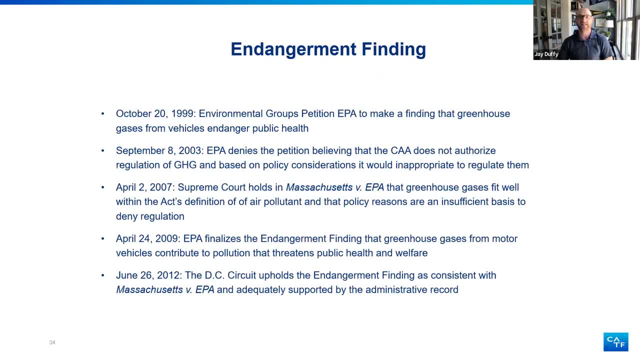 needs to be up with with the peace of um. Gym P in 2003 denied that petition And they said: you know, we believe that the Clean Air Act doesn't authorize us to regulate greenhouse gases And they also set forth a number of policy reasons. 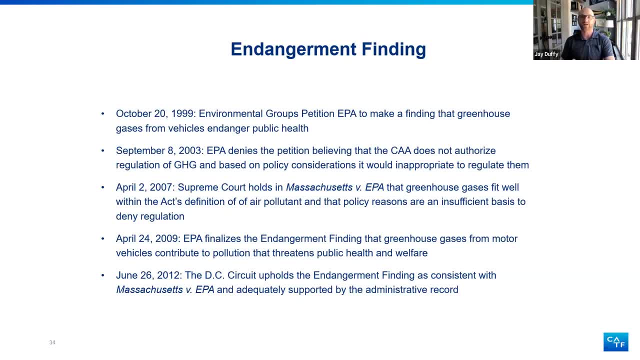 that they thought. you know, either way, it's not appropriate to regulate greenhouse gas emissions under the Clean Air Act, And these reasons included President Bush at the time's policy approach to climate change, which at that time, you know, didn't include Clean Air Act regulation. 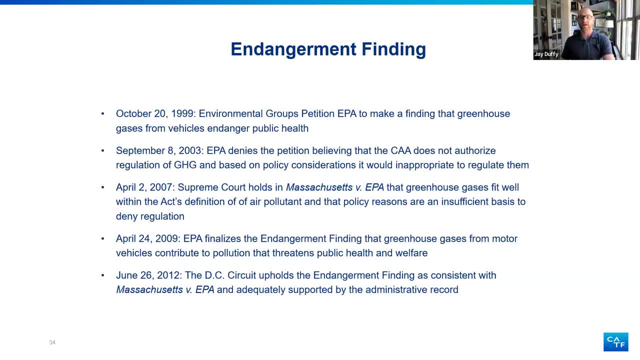 as well as the. you know it included other things, but not Clean Air Act regulation and the international nature of climate change. So they denied that petition and then several states and others, they challenged this denial And this ultimately results in the landmark 2007, Massachusetts. 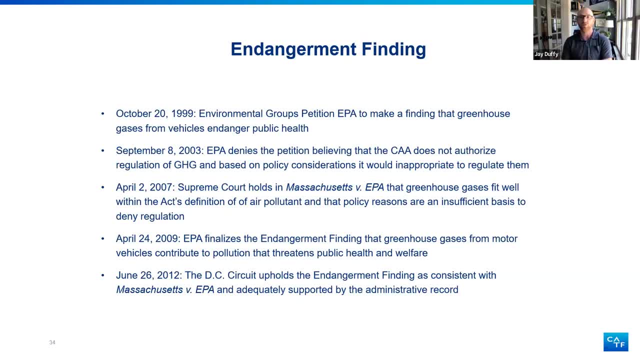 versus EPA Supreme Court opinion. And so there the court held that you know the Act's broad definition, that we've talked about a few times, of air pollutant unambiguously covers greenhouse gases And therefore EPA is obligated to regulate those emissions. if it makes this finding, that makes the 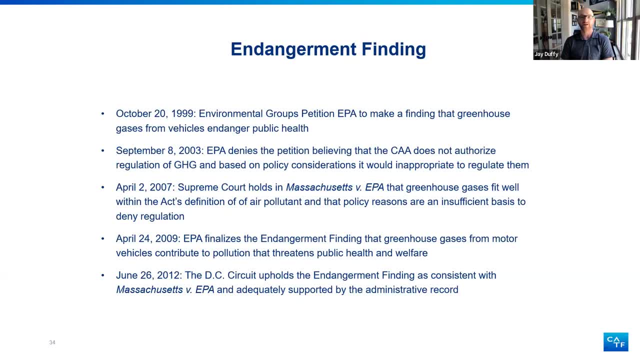 finding that greenhouse gas emissions endanger public health or welfare. the refusal to to regulate can't be based on policy considerations, it just has to be a scientific determination. you know if, if greenhouse gases endanger public health, then you must regulate according to the Act's instructions. So it was interesting at that time. 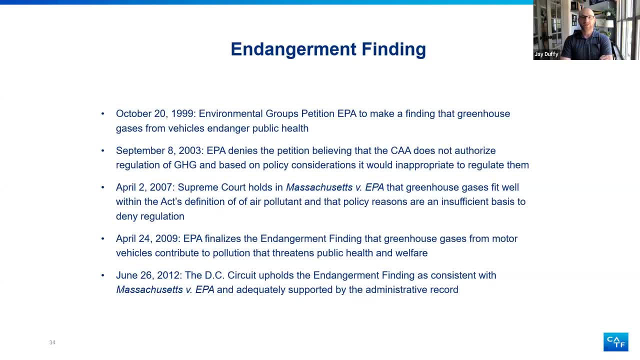 when EPA denied the petition, the majority of the court, you know, explained as I, as I just did, that it is covered by the Clean Air Act and and the policy considerations are irrelevant. But the Chief Justice and Justice, Scalia and Thomas and Alito, at that time they would have deferred to EPA's 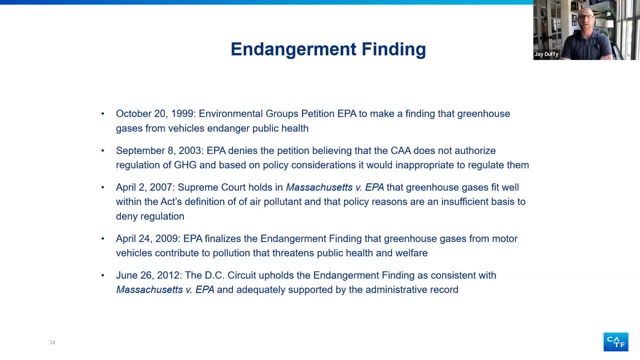 policy reasons. they said that you know, no matter how big of an issue climate change is, you know Congress passed this really malleable statute which gives broad discretion, you know, not to a court, but to EPA, and they would defer to the agency. And we'll see as we. 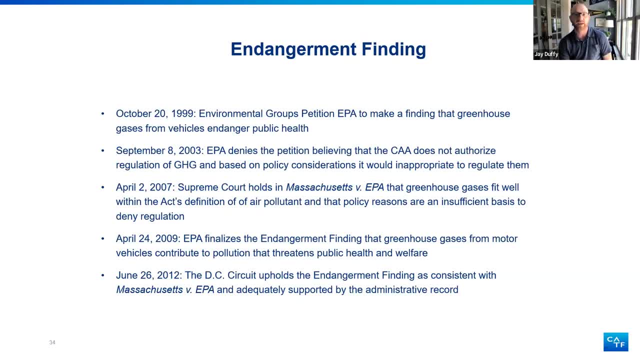 fast forward. they are no longer, you know, deferring to to the agency when it comes to issues associated with with climate change in many respects. So the court sends the denial back to the agency to reconsider in light of these new instructions. So then, in 2009,, the Obama 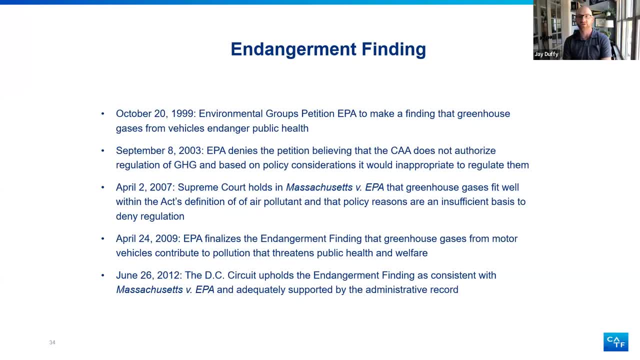 administration finalized the endangerment finding, they concluded that the agency was not able to make a decision that included that greenhouse gases do indeed endanger public health, And then that decision was upheld by the DC Circuit Court of Appeals in a case called Coalition for Responsible Regulation versus EPA in 2012.. The court found that the finding was consistent with 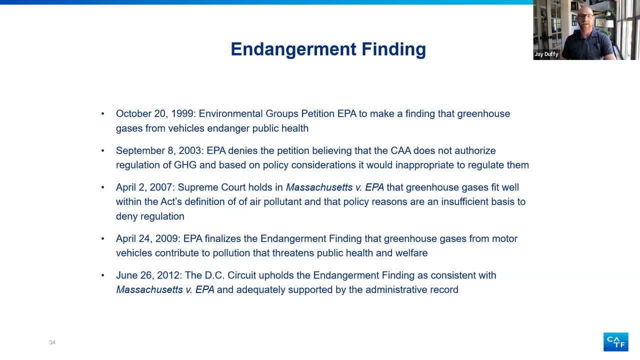 Massachusetts versus EPA and that the text and the structure of the Clean Air Act is is adequately just and it's adequately supported by the administrative record that that EPA put together all the science and data that they put together, the court found was sufficient. But you can see here: 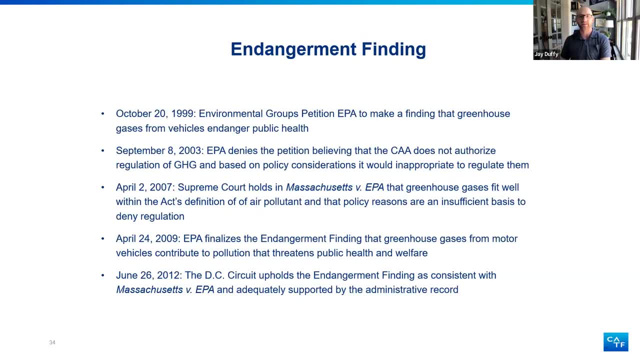 you know it took from. it took a petition in 1999.. Until a final. you know, 10 years later, the Obama administration finalized the endangerment finding and then it is upheld in 2012.. So these things take take significant time And you know the this finding continues to come under. 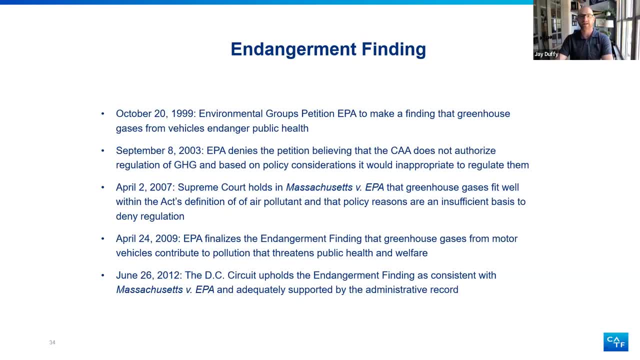 come under attack. Just this past year I represented clients on the side of EPA funding off additional petitions to reconsider the endangerment finding. The DC circuit rejected those challenges Because none of the challenges had standing. they couldn't show how they were. 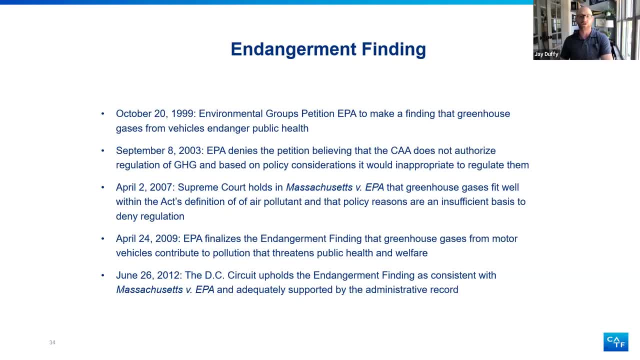 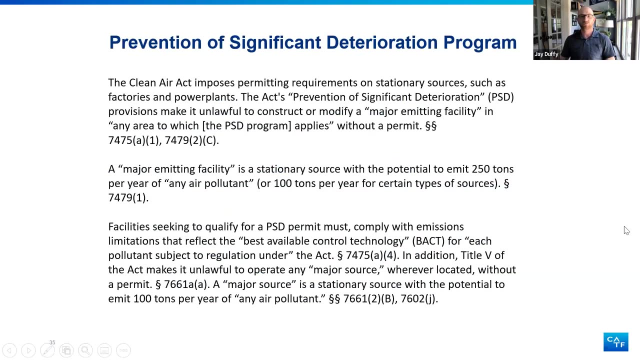 harmed by the endangerment finding. And then also Congress codified Massachusetts versus EPA that ruling in the Inflation Reduction Act last summer, kind of trying to make it crystal clear that greenhouse gases are covered under the Clean Air Act. So we move on. So now we're going into the last slide. at this point I will turn it over to you. and I think, again, this is an important part of it. I think this is a key element, I think it's an important, So we move on. So now we're going into the last slide, I think, and I think it's an important. 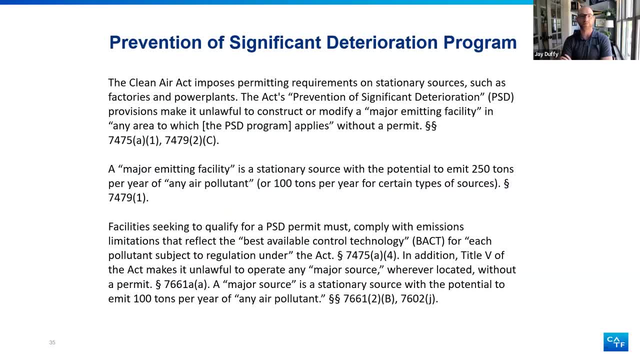 So we move on. So now we're going into the last slide. I think it's an important. So now we have this finding that the greenhouse gas is in danger of public health, but we're not regulating it yet. So how do we figure out how the greenhouse gas regulation fits in with the other provisions of the Clean Air Act? 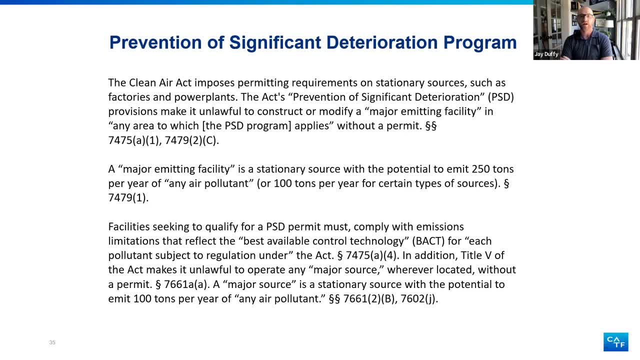 We'll talk about Section 111 standards a little bit later. but they set the floor for the standards And 111 also pulls in unregulated existing sources. But once you set that floor of these performance standards under 111, the Prevention of Significant Deterioration Permitting Program sets source-by-source standards, not standards, for you know what's the floor- that the whole source category can meet. 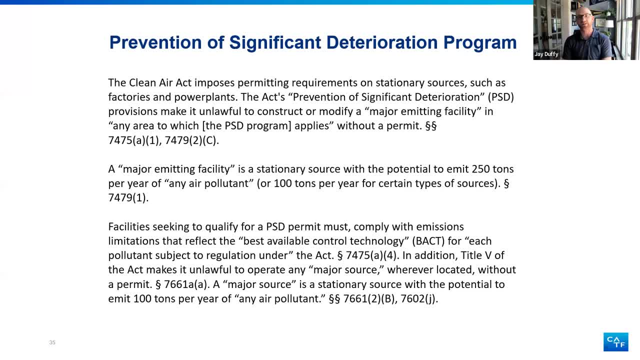 The permitters then go in and look at each particular source and determine what's the what's the best available control technology available for that particular source And a major source of- And this regulates major sources here. in this particular instance, A major source is one with the potential to emit either 100 to 250 tons per year of pollutant, depending on the air quality where the source is located. 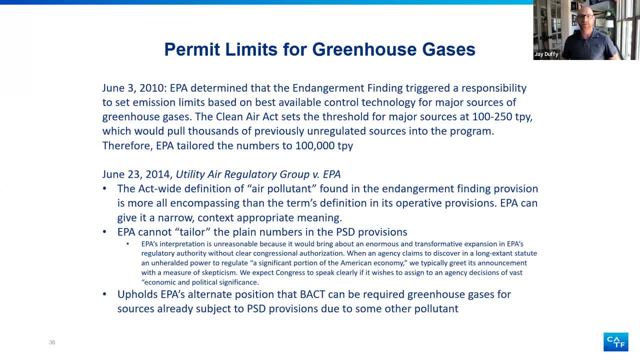 So since EPA found that greenhouse gases were an air pollutant that endangered public health, they assumed that they were compelled to regulate major sources of that air pollution. The problem, of course, was that greenhouse gas emissions are much more prevalent than other pollutants that are subject to the Act. 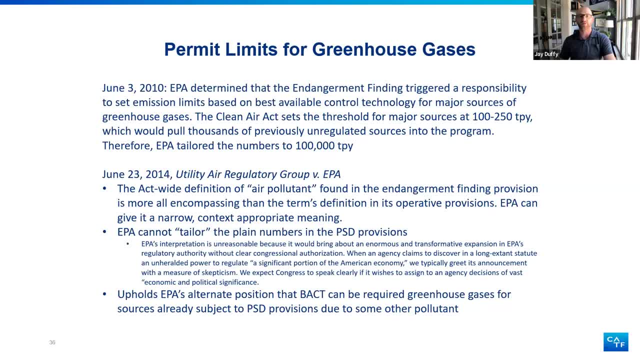 So regulating every new and modified source of 100 to 250 tons per year of greenhouse gases would pull in tens of thousands of previously unregulated sources into the purview of the Clean Air Act. So EPA tailored the Act And they said they would only regulate sources that emit over 100. 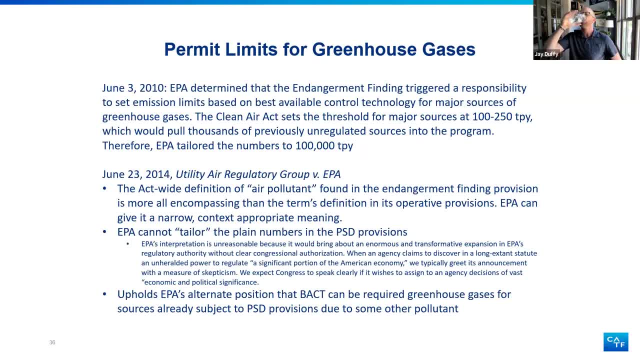 1000 tons per year of carbon dioxide. So in Utility Air Regulatory Group versus EPA- and this was the first set of briefs I worked on, actually, when I came over to Clean Air Task Force- there the Supreme Court determined that the Act-wide definition of air pollutant- that was the one relevant in Massachusetts- versus EPA and the endangerment finding provisions 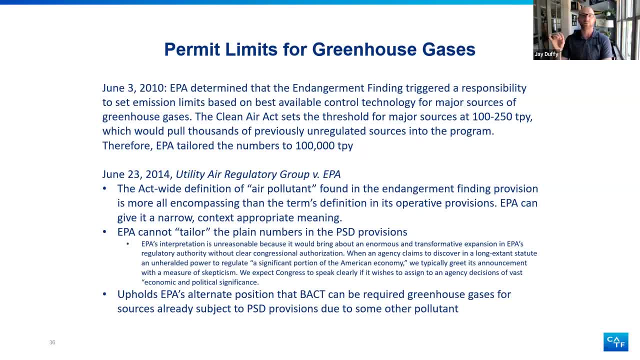 they need not have the same breadth in their. There were provisions of the Act like the permitting provisions, So there was no automatic trigger resulting from the endangerment finding to cover greenhouse gases in the permitting provisions. So further, the clear language of the Act said 100 to 250 tons per year of pollution and EPA has no authority to rewrite what Congress wrote. 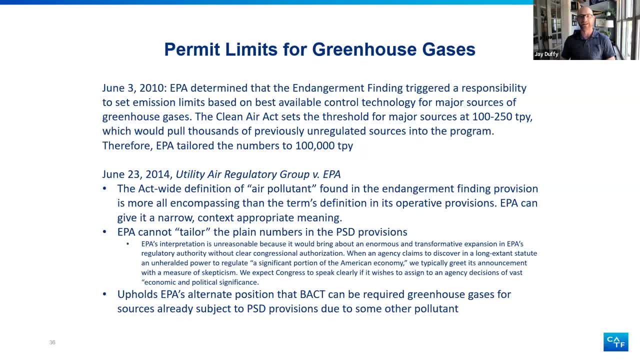 That's kind of basic statutory interpretation 101.. You can't cross out 100 to 250 and put in a new number. So the court in an opinion written by Justice Skilfer Leah. they also remarked that EPA's reading of an automatic trigger, as I said, contradicted the plain language of the statute. 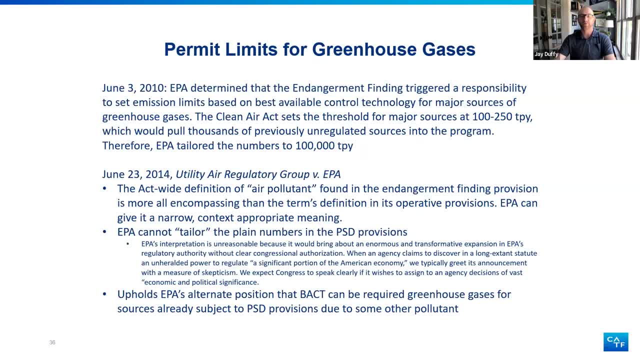 It was also unreasonable because- and this language comes up over and over again now- because it would bring about an enormous and transformative expansion of EPA's authority without clear congressional authorization, When the agency claims to discover in a long extant statute an unheralded power to regulate. 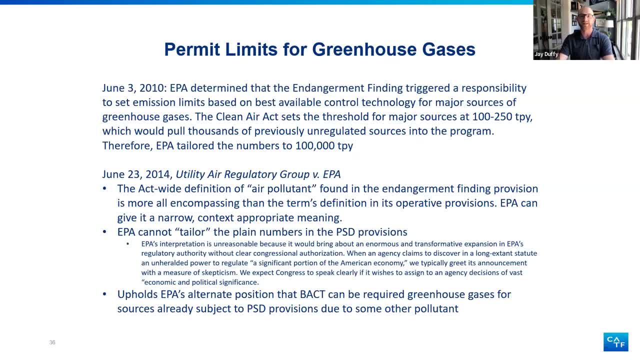 a significant portion of the American economy, we typically greet its announcement with a measure of skepticism. We, the court, expect Congress to speak clearly if it wishes to assign to an agency a decision of vast political and economic significance. So at the time, we, the folks who have been working on this case, we read this just as commentary. that made sense. 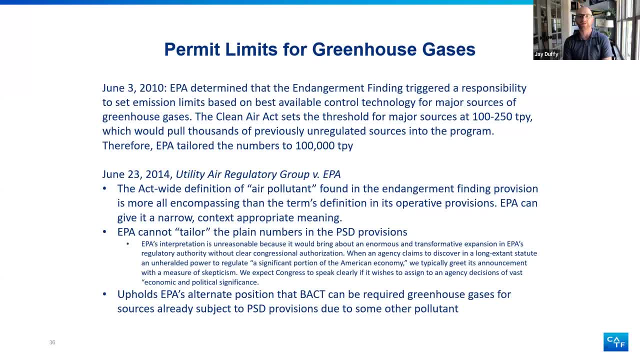 because reading the Act to trigger greenhouse gas regulation in accordance with that 100 to 250, 100-per-year limit would lead to regulation of tens of thousands of very small sources, you know, laundromats, hotels, residential buildings. But so at that time that all kind of made sense. 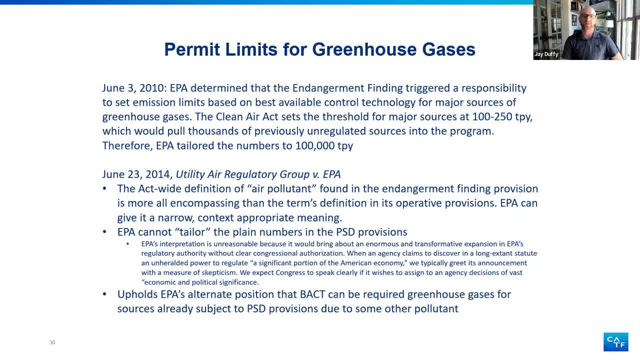 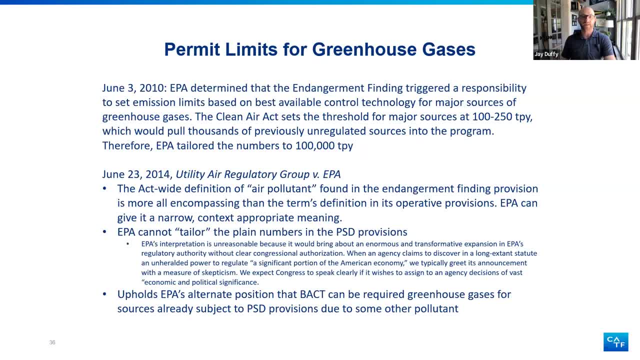 of EPA's backup position And that was that they could regulate greenhouse gases under the PSD section for sources that were already subject to the permitting provisions by virtue of some other pollutant- And they call this the anyway sources. They're covered by these permitting. 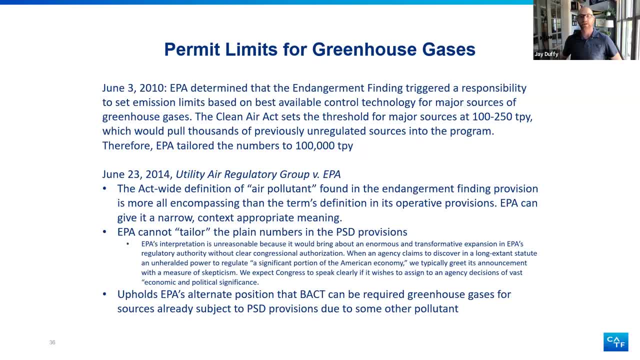 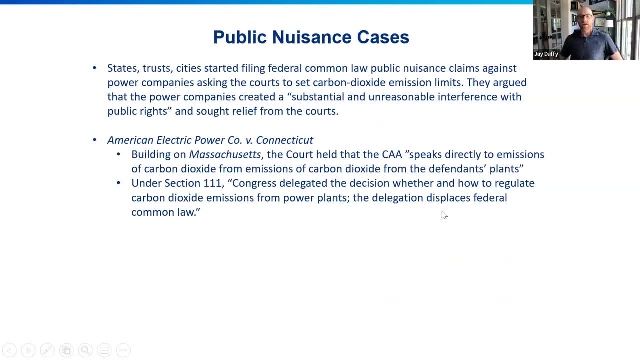 provisions anyway And therefore we can regulate their greenhouse gas emissions under the section. So I'm going to talk briefly about the public nuisance, just because of what it meant for the Clean Air Act. During the same time period, states and trusts and other groups were filing public. 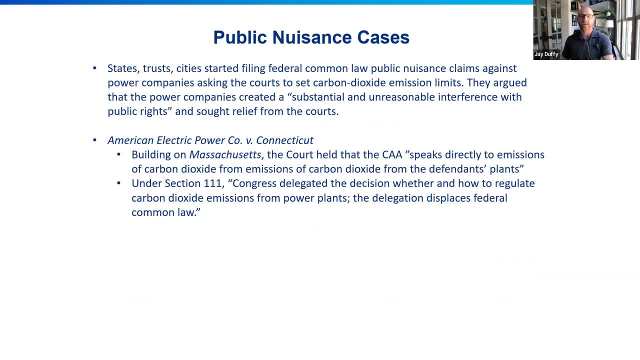 nuisance claims against major climate polluters. They claimed that the polluters, generally power companies, created a substantial and an unreasonable interference with public rights, And they sought relief in the form of emission limits that the court would write One of these cases. 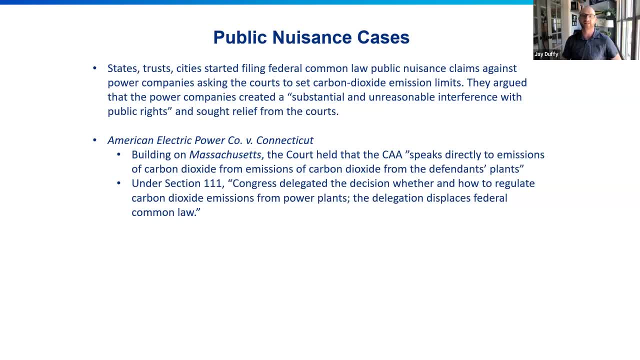 made its way up to the Supreme Court, which said that the Clean Air Act, Section 111, occupied the federal space here and it preempted the public nuisance claims. It wasn't for the courts to set emission limits, That was EPA's job. So, building on Massachusetts, the court held that the Clean 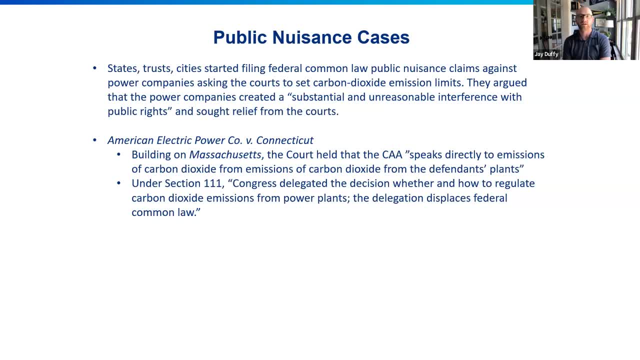 Air Act speaks directly to carbon dioxide emissions from defendants' power plants And under Section 111, Congress delegated that decision of whether and how to regulate carbon dioxide emissions from power plants, And that delegation displaced federal common law. So now we have a clear signal from the court as to 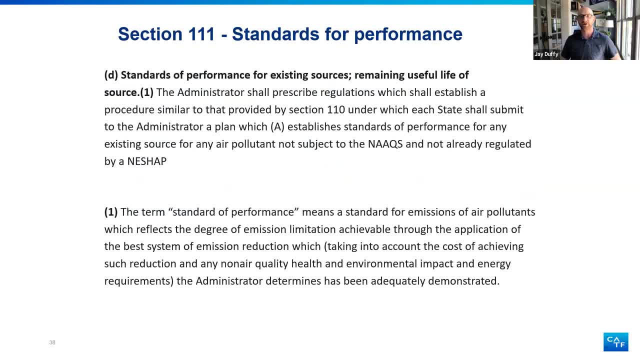 the place within which we should be thinking about how to regulate greenhouse gases. So with that signal, the Obama administration set about setting Section 111 standards. So under Section 111B- and this is a little bit of a refresh, since we've already covered a bit of this- 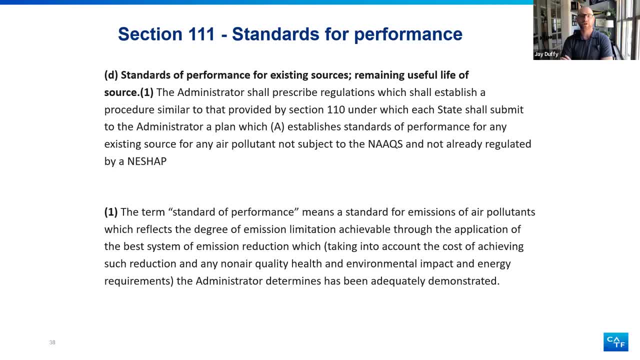 EPA sets performance standards standards directly for new and modified sources Under Section 111D. as in DOG, EPA sets emission guidelines for existing sources based on EPA's standard of performance determination, And then the states apply those emission guidelines directly onto the sources. 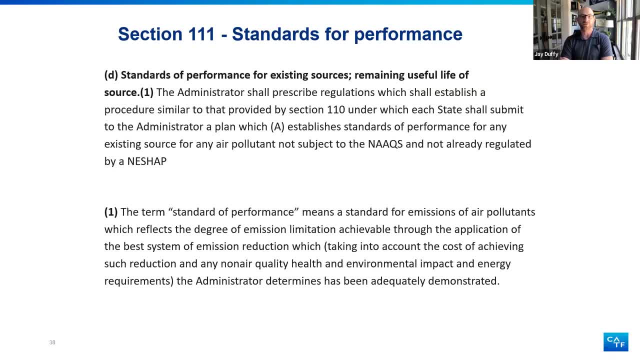 and they can consider the individual plant's remaining use of life and other factors. So Section 111D guidelines can only be set once Section 111B standards are set for new sources in the same category And Section 111D standards can only be set for pollution that isn't covered. 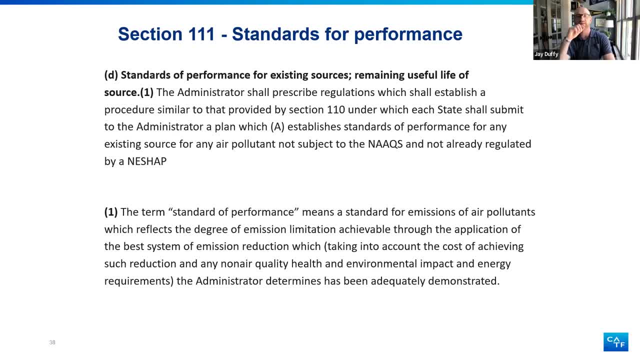 by a NAX and that source so like power plants, so that pollution is not covered under the hazardous air pollutant standards. So here we have power plants and we have CO2. CO2 is not under the NAX and it's not regulated for power plants under the hazardous air pollutant. 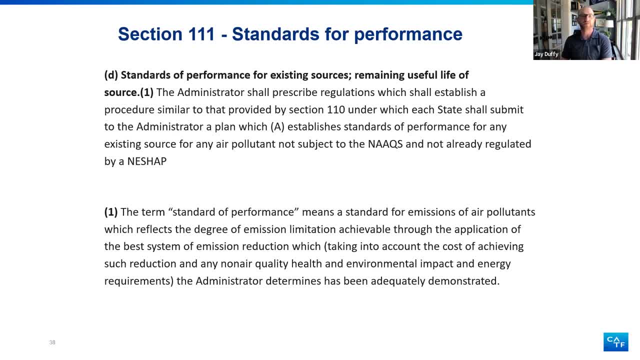 sections of the Clean Air Act. So a standard of performance, as we mentioned, reflects the emission limitation achievable by the best system of emission reduction, taking into account costs and other factors that EPA determines has been adequately demonstrated. There are decades of case law defining what reasonable cost is what adequately demonstrated means. 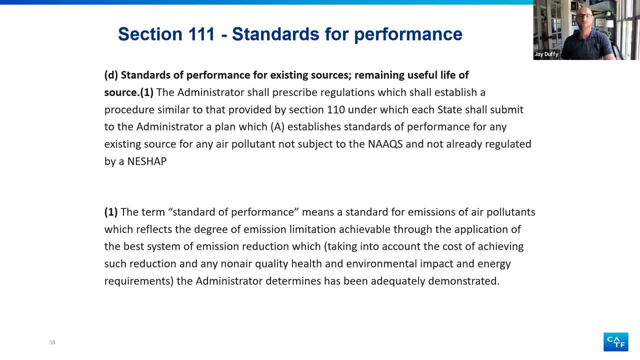 and what not. So this is a standard of performance. as we mentioned, reflects the emission limitation and what it means to be the best system For the existing sources. the Clean Air Act requires EPA to choose the best system of pollution control, set an emission limit. 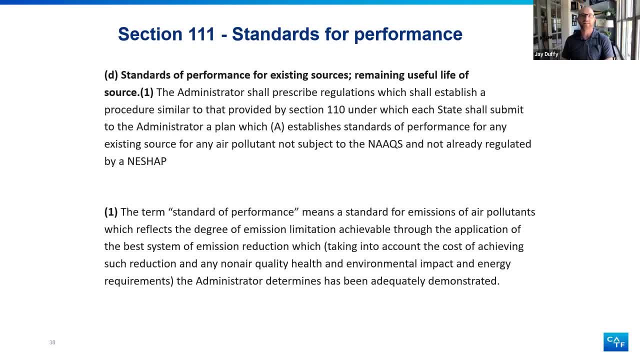 and then the states have the flexibility to design a plan that is equivalent to the emission limit. They can also take into consideration, as I said, the remaining use of life of the plant and other factors in setting these individual emission rates for their plants And they 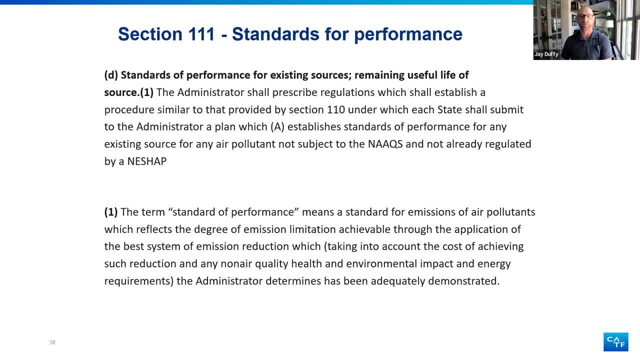 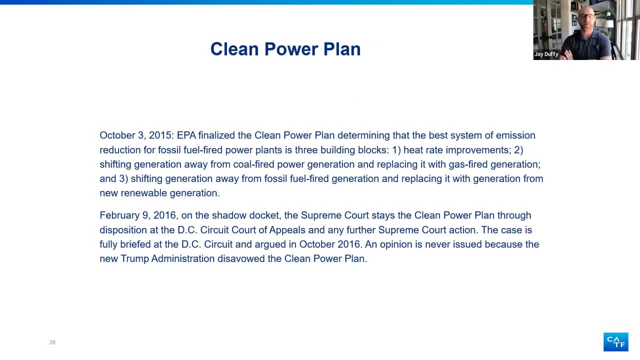 can also decide not to write a plan and EPA will write a plan for them. So let's get into these kind of three attempts at doing. Section 111: standards for the power sector for greenhouse gases. In 2015,, EPA set standards for new gas and coal plants. The standards for 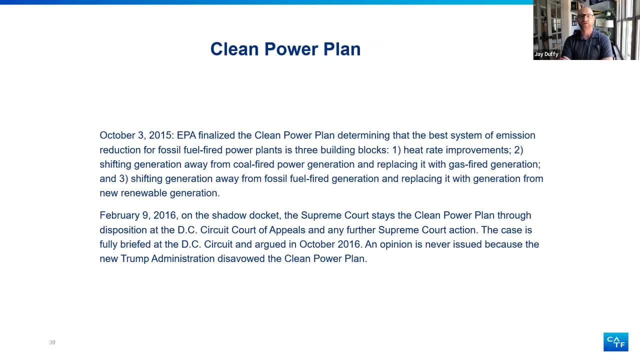 gas plants was based on minimal efficiency measures and the state of the art at the time and the standard for new coal plants, of which none were projected. no one was building any new coal plants at the time, but that was based on partial carbon capture and sequestration. 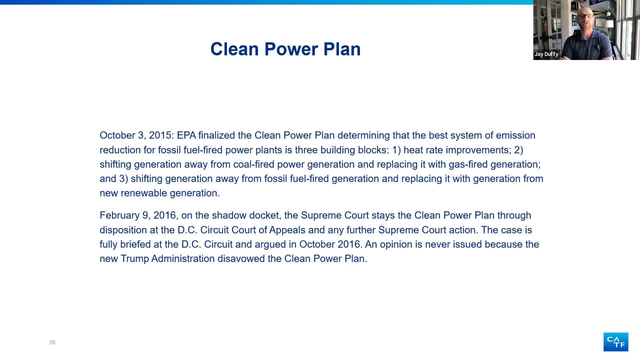 could also be met by co-firing with gas. So these rules for the new power plants were challenged and they were fully briefed at the DC Circuit, but then the Trump administration told the court that it was going to repeal them. It ended up proposing to repeal these standards for new. 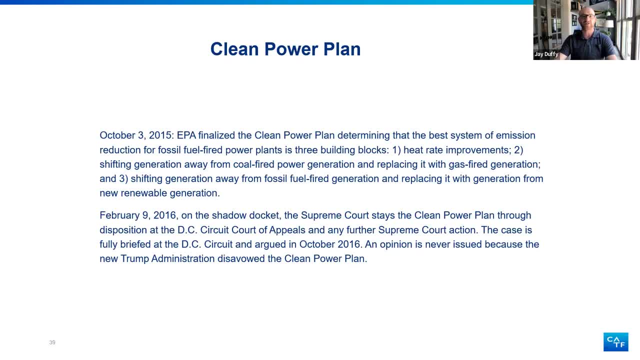 sources but never finalized it, And that challenge is still sitting in abeyance or on pause at the DC Circuit. What got a lot more attention were the emission guidelines for existing gas and coal-fired power plants- That's the Clean Power Plan. So EPA looked at more traditional pollution controls like 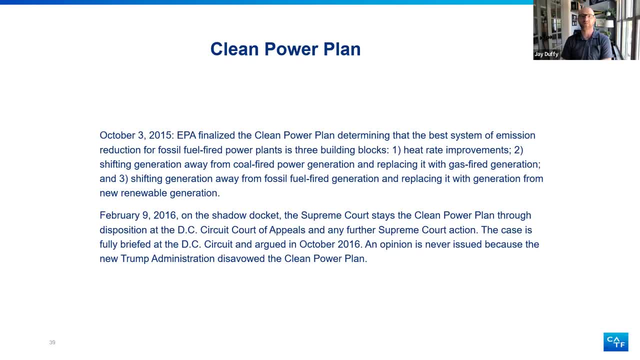 co-firing with natural gas or installing these carbon scrubbers. but it found that even if it set standards based on those pollution controls, the sources would meet that standard by just shifting generation to cleaner sources, and that this is how the industry had been reducing. 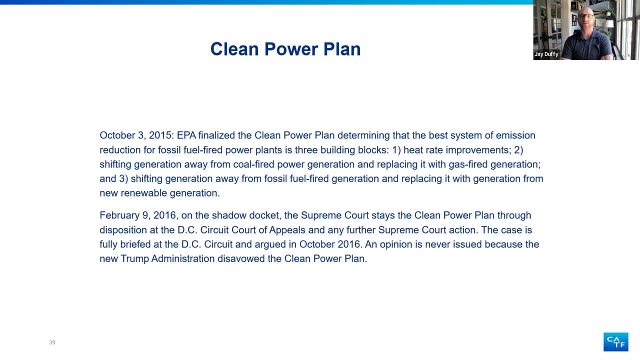 emissions most efficiently and reducing emissions, And that's what we found. So EPA looked at more traditional pollution controls, like coal-firing with natural gas or installing these carbon scrubbers, but it found that even if it set standards based on those pollution controls, the sources would meet that standard by just shifting generation to cleaner sources. And that's what the agency based the 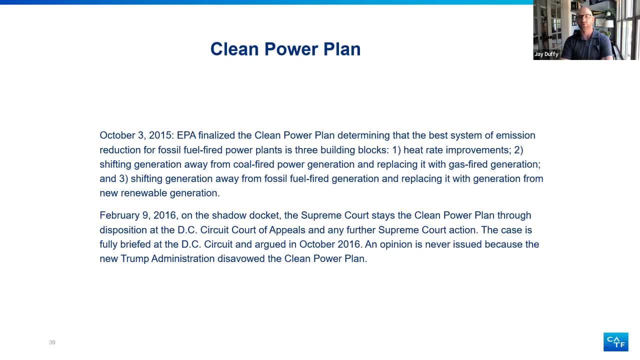 guidelines on. They called them three building blocks. One was efficiency improvements, one was shifting generation away from coal-fired generation to gas-fired generation. And the third building block was shifting generation away from fossil generation toward renewable generation. EPA looked at how much shifting could be done cost-effectively and without impacting reliability, and they set the 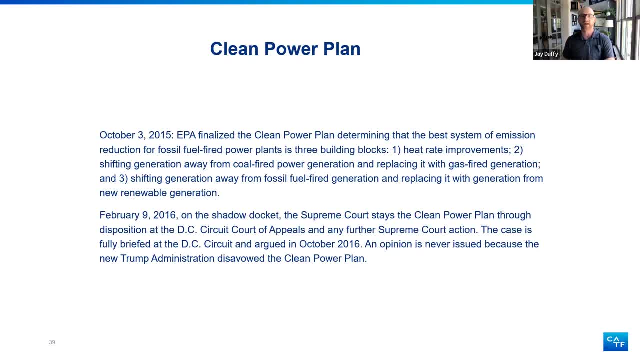 emission limit there And they set the emission limit there. So once the power plant was done, Once that rule was finalized, it was challenged by industry, trade groups, states and coal interests in the DC Circuit. They sought to pause the rule while the litigation ensued. 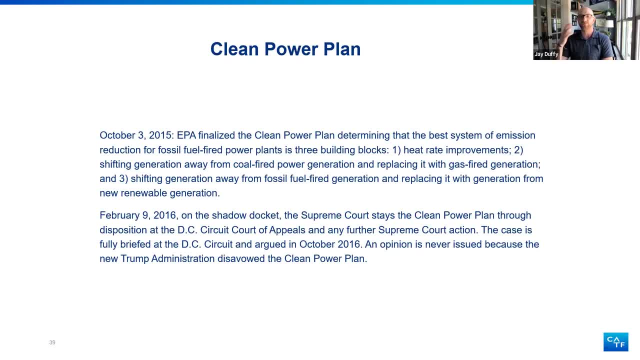 Pam, I'm getting a little bit of feedback. If there's any way you could mute, it's just I'm getting a reverb of myself back at myself, And as much as I like hearing myself twice once is enough. There was, let's see where I was at. 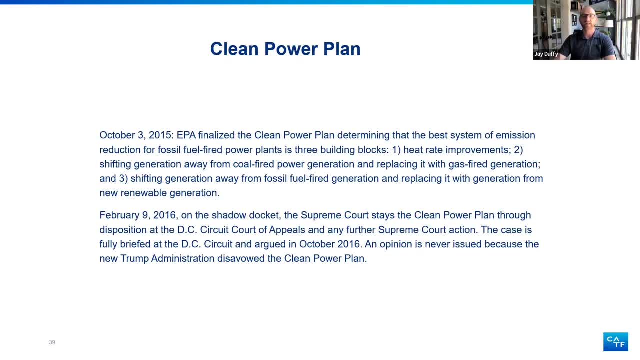 Okay. so once that rule was finalized, it was challenged and the party sought to pause the rule while the litigation ensued, but they were denied by the DC Circuit. They then sought relief from the Supreme Court, which asked them to, and they asked the Supreme Court to stay the rule. 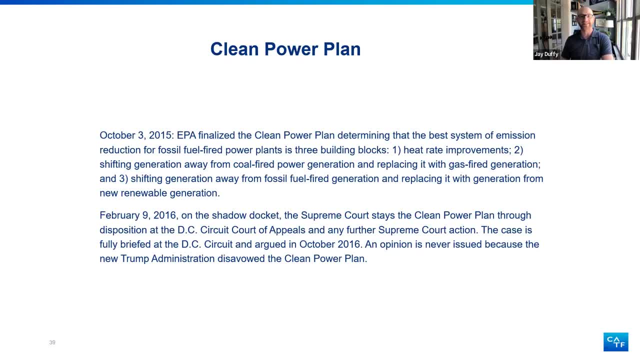 That briefing was done over a matter of days and nights. I can attest to and on the shadow docket, with no explanation. It was actually Justice Scalia's final action before he passed away. They stayed the effectiveness of the clean Power plan for the duration of the court proceedings and it never went into effect and won't. the case then was was fully briefed at the DC. 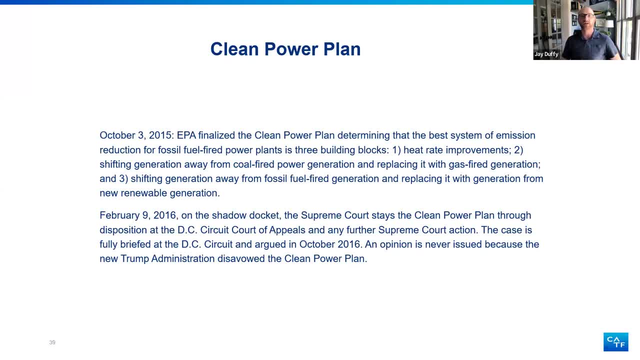 Circuit. Oral argument was held before a full court, including then Judge Cavanaugh, on the DC Circuit. That was in September 2016,. but the court never issued an opinion because the Trump administration disavowed the clean power plan once they came into office. 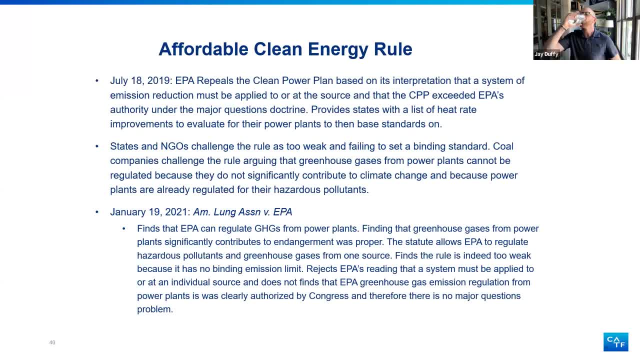 So, then, two years went by Before the Trump administration, EPA repealed the clean power plan, based on its interpretation of the Clean Air Act that only systems that that can be considered for the basis of performance standards are those that can be applied to or at an individual source, and that this kind of generation shifting was not, you know, a kind of bolt on to or at the individual source system. 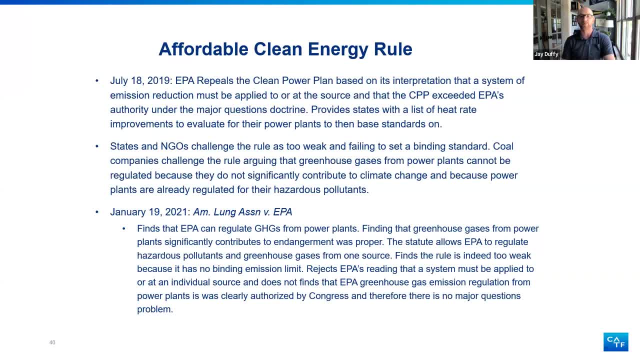 They also, as kind of a backup Argument, said that the clean power plan exceeded EPA's authority under the major questions doctrine, which they understood to preclude, you know, any any costly, really expensive or politically important rule, unless the rule was clearly authorized by the act. 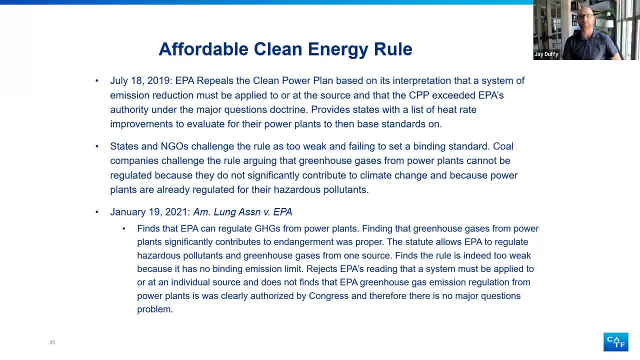 The Act. our, however, has as broad language as we've discussed, kind of applicable to multiple pollutants and to sources, So it doesn't specify or authorize any particular systems to replace the clean power plan. EPA issued The Affordable clean energy rule, or ace, and that provided states with a list of efficiency improvements that states could evaluate to set emission limits for the plants within their states. 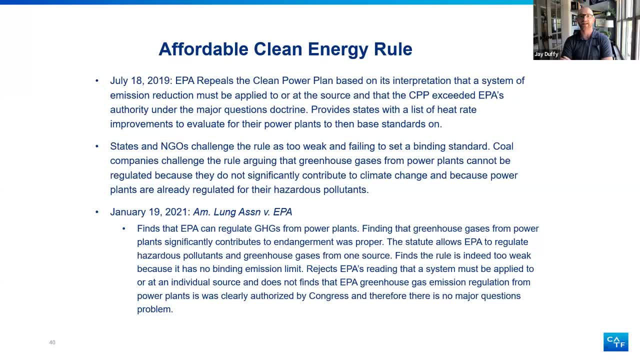 So environmental groups, some power companies and states challenge the role as too weak, noting that by you know, kind of investing in these coal plants and making them more efficient, They would likely run and pollute more and longer, and that there were better systems of pollution control available. 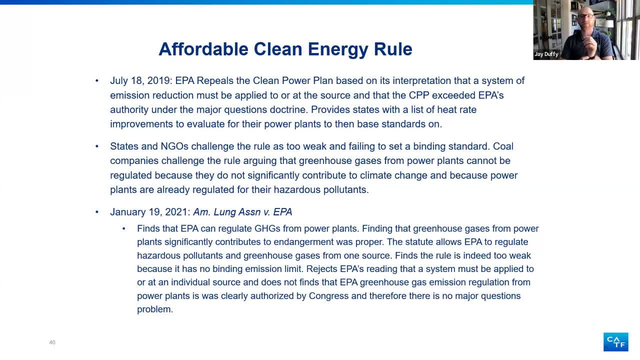 And they also pressed that ace, impermissibly failed to set, you know, kind of a binding emission limit. It just gave, gave states options. Coal interests also challenged the rule and they argued kind of from the other end that greenhouse gases from power plants don't contribute enough pollution to endanger public health and the environment. 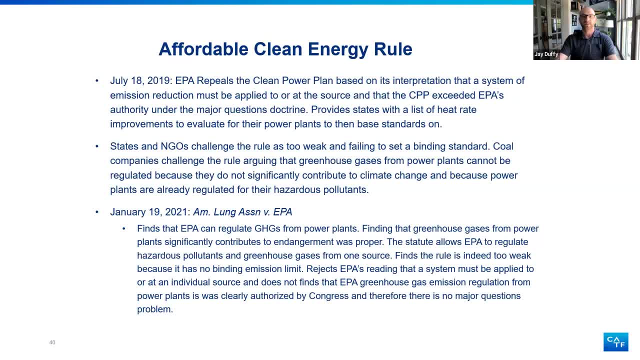 And you can see kind of again: this is our argument, that that the Clean Air Act doesn't cover cover greenhouse gases. And they also argued that Because power plants were already regulated for their hazardous air pollutants, they couldn't be regulated under another provision for their climate pollution. 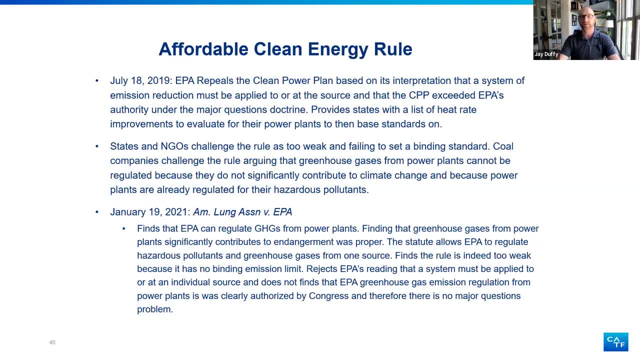 So on the last day of the Trump administration, the Dc Circuit issued an opinion finding that epa can regulate greenhouse gas from power plants. That the determination that greenhouse gases from power plants significantly contributes to endangerment was proper. that the statute does allow epa to regulate both hazardous pollutants. 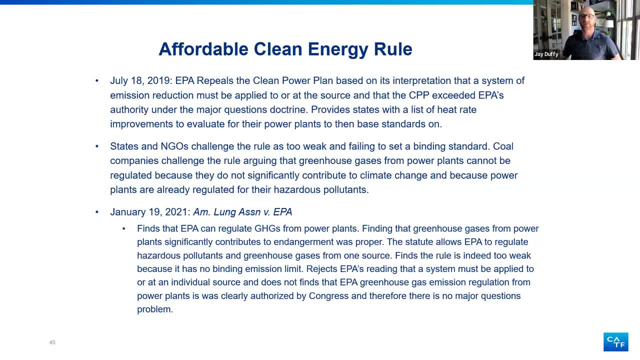 And greenhouse gases from one source under different provisions, and that the finding that the rule was in and they found that the rule was indeed too weak because it didn't have binding emission limits and it rejected epa's reading that the system must be applied to or at an individual source. 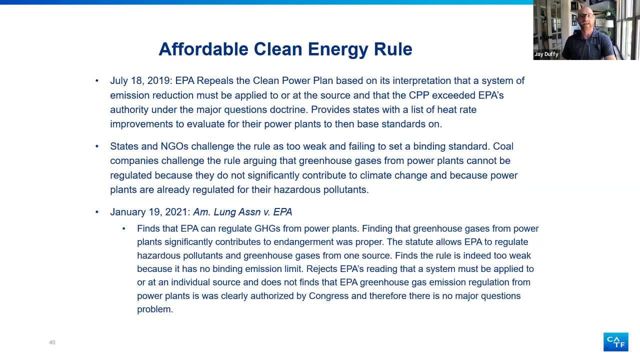 They couldn't find that in the plain language of the act and then, relying on the Aep versus Connecticut, That public nuisance suit, They found that epa's greenhouse gas regulation For For from power plants under section 111 is clearly authorized by Congress and therefore there isn't a major questions problem. 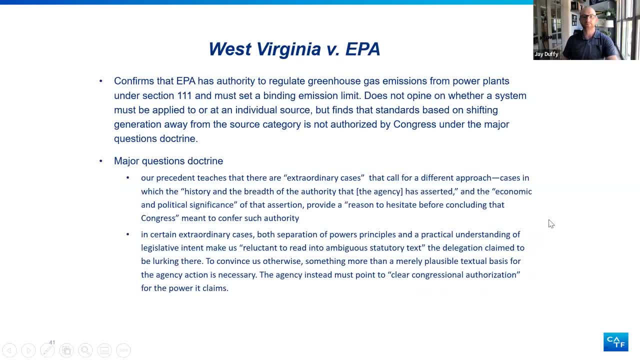 So this was appealed to the Supreme Court and in a decision last June The court confirmed that epa doesn't need to have authority to regulate greenhouse gas emissions from power plants under section 111, and that epa must set a binding mission limit. 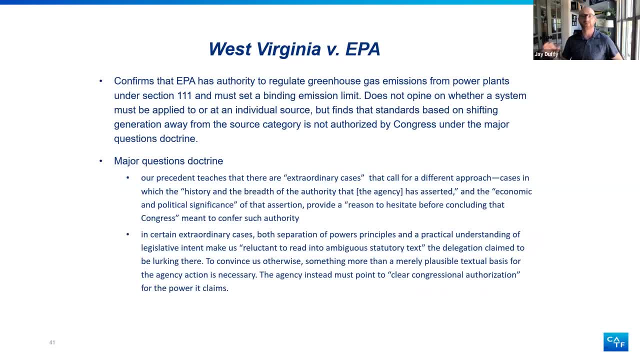 And it didn't opine on whether a system must be applied to Or at an individual source, but it did find that standards based on shifting generation away from the source category isn't authorized by Congress and that that violates the major questions doctrine. 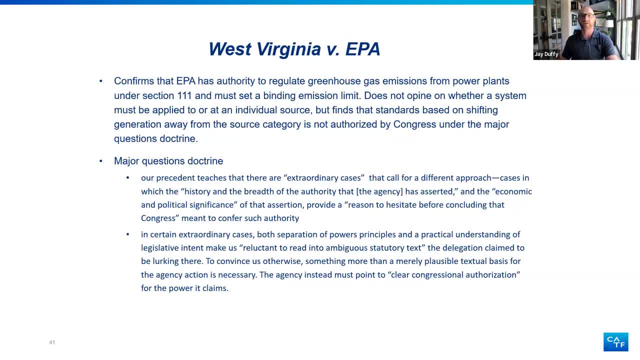 So this was the first time that the court kind of formally announced the major questions doctrine. Since the nineties there's been seeds of it in there and different flavors of it, But this was the first time they, you know, they, they recognize it by name. 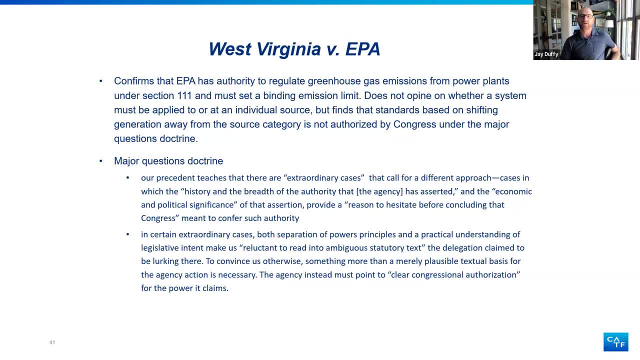 And they said: you know that their precedent taught them that there are extraordinary cases that call for a different approach to statutory interpretation. These are the cases in which you know the history and the breadth of authority that agency has asserted. the economic and political significance of that assertion provide a reason to hesitate before concluding that Congress meant to confer sort of great authority. 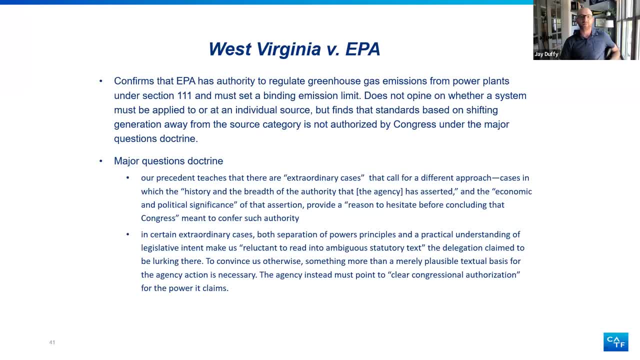 So, in these certain extraordinary cases, Separation of powers, principles, and you know, understanding what, what, what Congress might have meant made them reluctant to read into kind of this broad language that the Clean Air Act has a delegation, a delegation for, for more power, and in order to convince 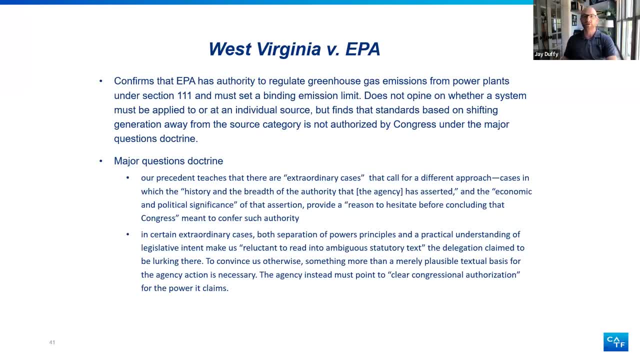 them. otherwise, something more than just broad language needs to be pointed to. There must be a be clear congressional authorization for the power that the agency claims. The court said that it couldn't locate clear authorization to base standards on shifting generation and therefore that the Trump administration properly repealed the clean power plan. 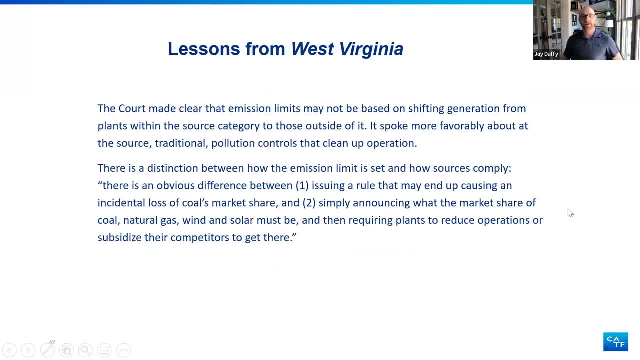 That was last June, and so now we're looking forward. right, so we're in thinking about how to go about regulating power plant climate pollution under section 111. West Virginia provides some guideposts. The The court was clear that standards can't be based on shifting generation from these covered power plants to uncovered sources like renewables or other generation sources. 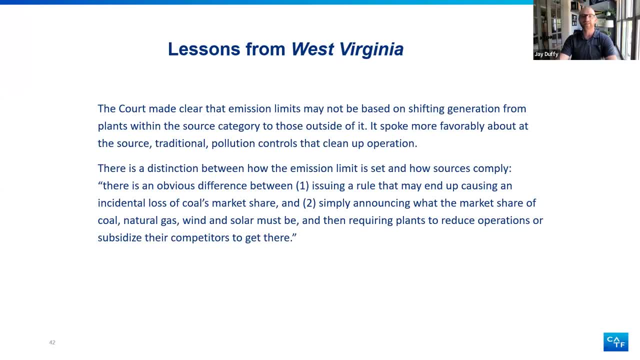 They did. they spoke more favorably of the traditional end of the stack, at the source pollution controls that cause the the covered plants to operate more clear. clearly, a cleanly sorry. They were clear that once an emission limit is set, based on an appropriate system, 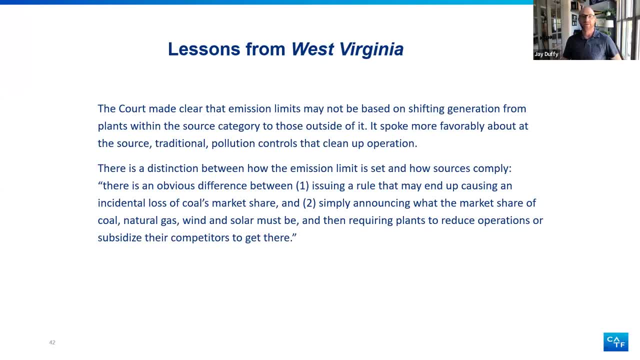 Then the plants can comply in any way they see fit, including by shifting generation. They said there's there's clearly a difference between setting the standard on on generation shifting versus setting a standard based on kind of traditional pollution controls and then the the plant deciding that you know now that it's being forced to internalize its cost of pollution. 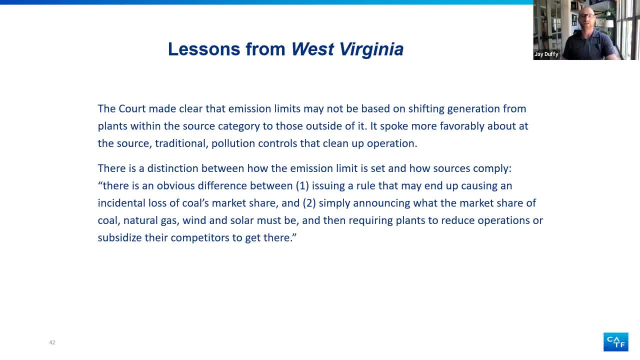 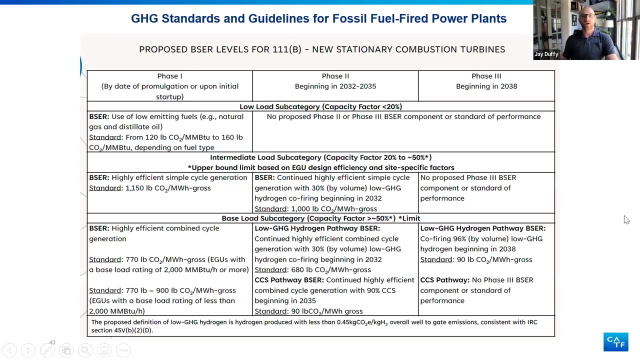 they may decide to shift to toward cleaner generation with lower costs. So that is permissible, but but basing the standard on on that, on the on shifting, is not permissible. So this is. this is a lot and I won't go through all of it. 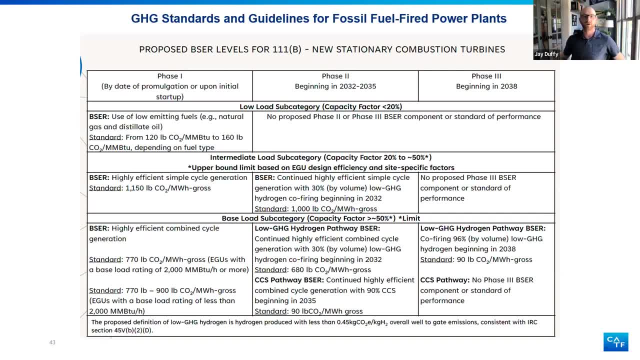 But I wanted to give folks a flavor of where we are now on. on May, the twenty third of this year, EPA proposed a new set of standards for the fossil fleet. They are accepting comments on the proposal until August eighth, about a month away. 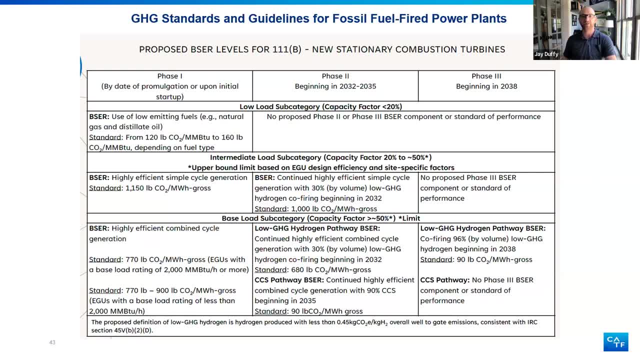 I have been vigorously writing with my colleagues and they're aiming to finalize the rule by the end of April 2,024.. So epa has authority to subcategorize and this is this is across across the the statute. They can subcategorize based on size, class and type of source and they use that authority really extensively in this proposed rulemaking to break the fleet into categories based upon what role the power plants are playing in the power. 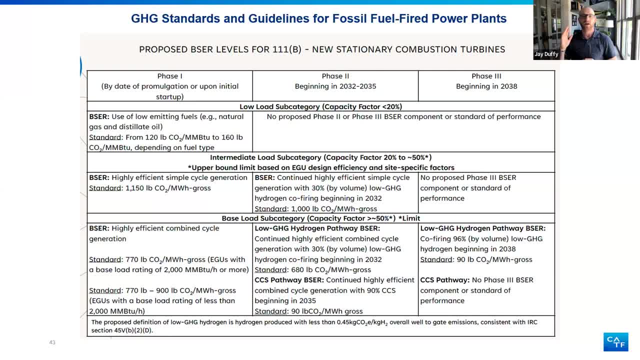 They're also providing very long timelines to allow for planning and permitting and building out infrastructure. So for new coal plants, epa proposes to leave those 2,015 standards in place, Those ones that that have been sitting in the Dc Circuit for for years. They are, but they've been in places for for 8 years now and they're based on on partial capture, partial Ccs. 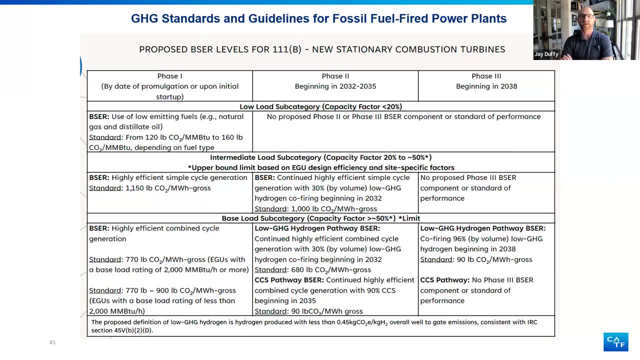 And for new gas plants. epa divides the fleet into 3 categories back based on how much the plants are operating. Are they at low load, intermediate load or base load? How, how often are they running? you know, 20% of the time, 50% of the time, etc. 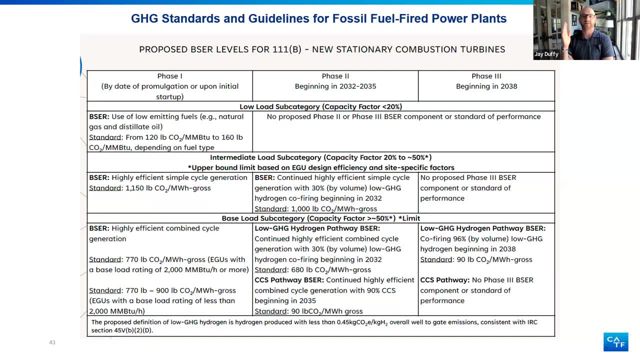 And for some categories they provide time to ramp up to the full best system standards. So those are the phases you see across the top. for those little, those peakers that are only running 20% of the time or less, They must stay before below that threshold and use the lower emitting fuels for the intermediate load. Before 2,032.. They just have an efficiency standard based on simple cycle turbines, But this then in 2,032 the plants will have a tighter standard based on 30% co-firing with low greenhouse gas hydrogen. They are tailoring low ghg hydrogen to tax credits. 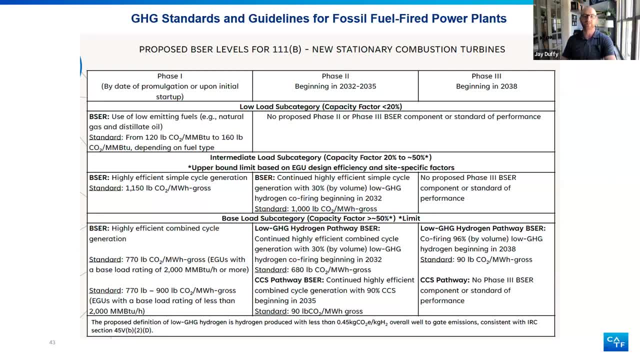 It found in the Inflation Reduction Act that was passed last year, and there's a, a tax credit called 45 V That incentivizes use of cleaner technologies, A cleaner hydrogen. there's several actually tax credits that are relevant here. There's others for that that that provide credits for carbon capture sequestration as well. 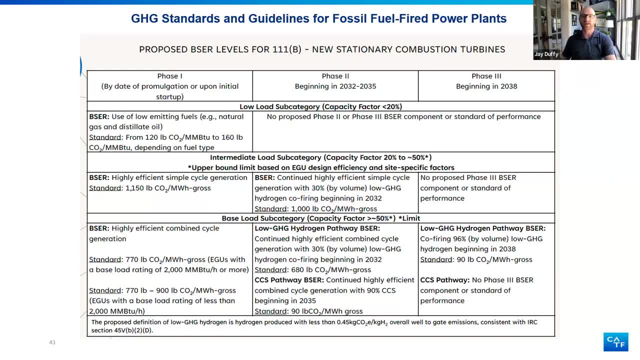 So i'll move on to new base load gas plants. The first phase it will be based on efficiency and after that epa is proposing 2 pathways, one for Ccs and one for hydrogen. for hydrogen, The plant will co-fire with 30% hydrogen, starting in 2,032.. 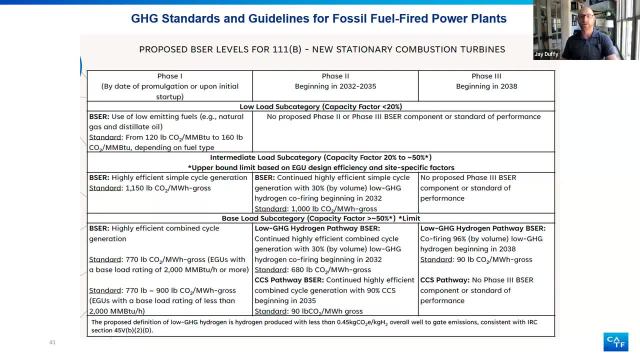 And then ramp up to 96% in 2,038, and for the Ccs pathway The plant would need to meet a standard based on 90% Ccs in 2,035.. So just to give you a flavor of kind of what the what epa is trying to do, which is to kind of tailor- tailor the standards to how these plants are operating and really focus on those traditional at the source stacks and give long lead times. 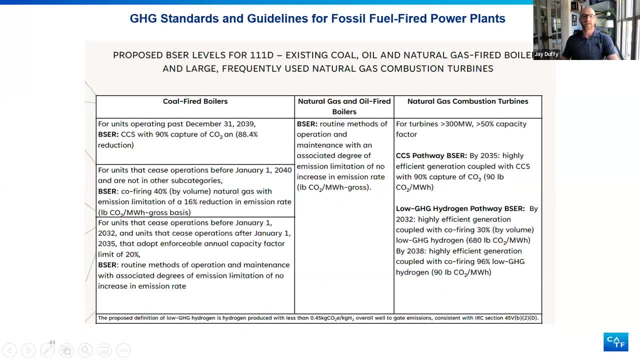 for existing plants. Again, the epa is dividing the fleet. for coal plants. They're dividing the fleet based on when the plant commits to retire, Those that plan to commit to a plan to retire before 2,032. They just have to maintain their rate. a plant that commits to retire by 2,035, and run less than 20%. 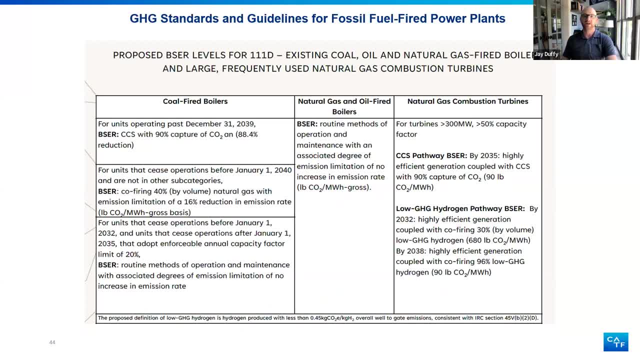 Also can keep its rate emission rate and a plant retiring before 2,040, but not falling into one of these 2 subcategories. Their system of emission reduction, Their standard is based on 40% co-firing Of natural gas and if you're operating past 2,040, the the standard is based on 90% carbon capture. 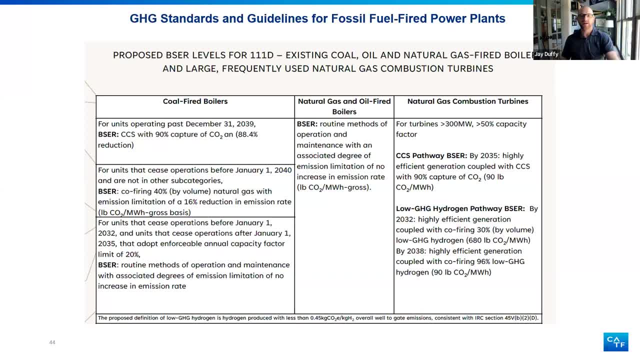 The middle column is a really tiny fleet so i'm gonna skip over that one. and for existing gas, The proposal would cover units that are larger than 300 MW. So they're not- they're not covering the entire existing gas fleet. They're taking kind of a stepwise approach here. 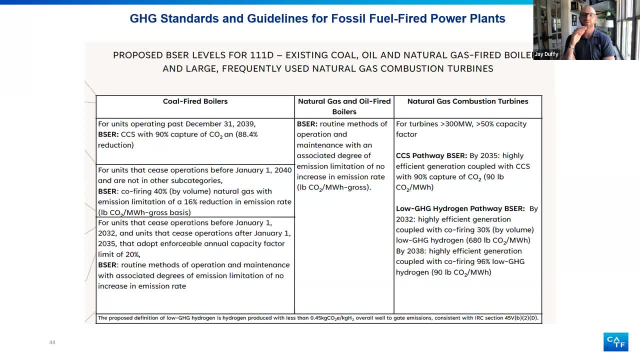 But so they're just covering with a Ccs Based standard Those plants that are larger, those units that are larger than 300 MW and run more than 50% of the time, And they're taking comment on on lower, lower pieces there. 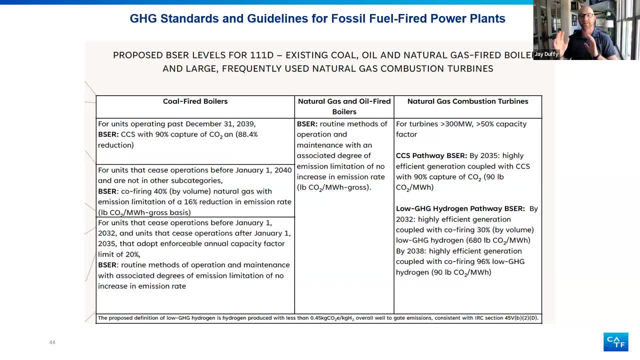 And then if, if, for those plants there is again that that Ccs Or hydrogen pathway, if they're, if they're, covered. so that is all for me. Sorry for the the rapid fire, but I wanted to to cover all this. I can go into some questions or I will. I will throw it back to Pam to to Mcs. 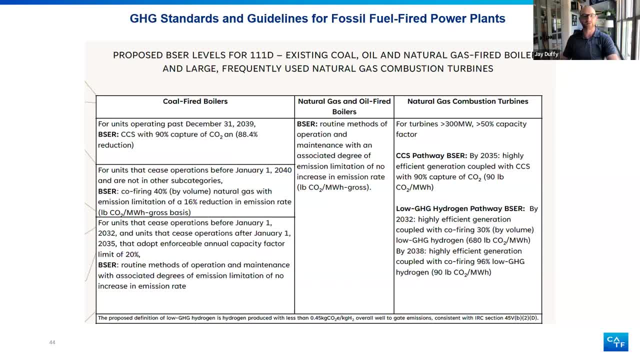 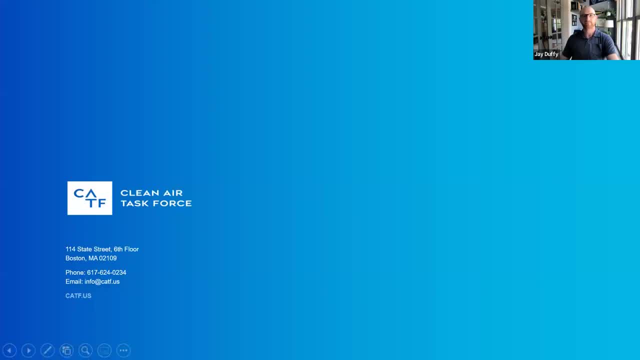 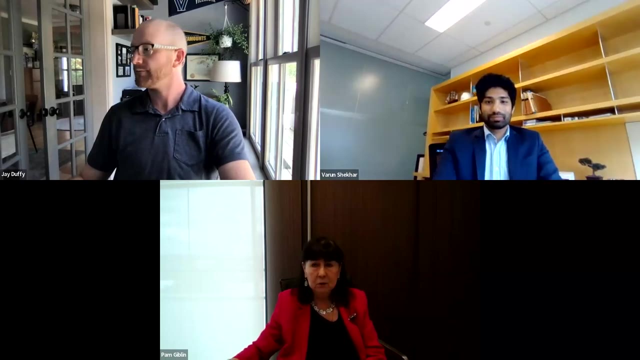 As to how we'd like to spend our our last 10 min. 10 to 12 min here. You're on mute, Pam, And yes, the i'm looking at a question here. The the endangerment finding regarding greenhouse gas emissions from power plants is is definitely viable after, after West Virginia. 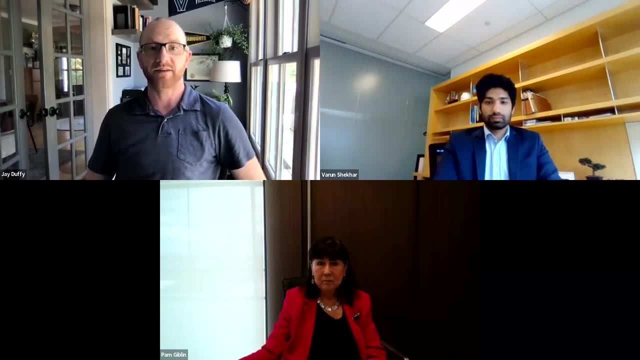 It, it. it says in the in the opinion that the greenhouse gases are covered. They only took issue with how epa was regulating the greenhouse gas emissions, not that they were doing it. Well, what I was saying when I was muted was that you did a superb job, because the prognostication piece is is the toughest. 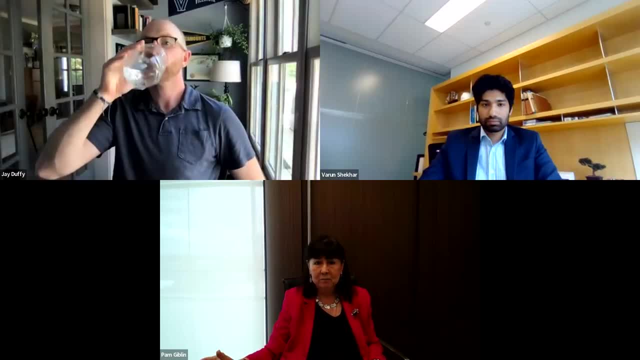 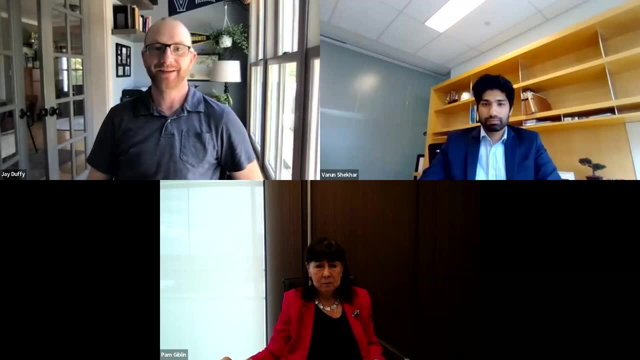 You know, A lot of us have talked about this. I've talked about what the Clean Air Act provided before, and then you gave us one of the best explanations of where we're going in a very tricky area. So thank you. So let's see. 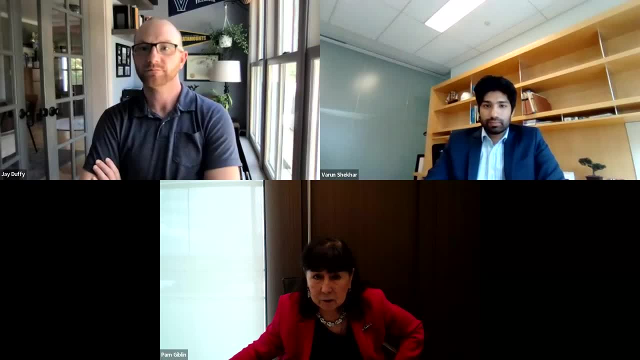 We do have a few questions. Let me see if there's anything specifically related to climate in. there. is captured ghg a hazardous waste? I've been telling myself. Is that? No, it is not. captured. coq is is not defined as a as a hazardous waste. 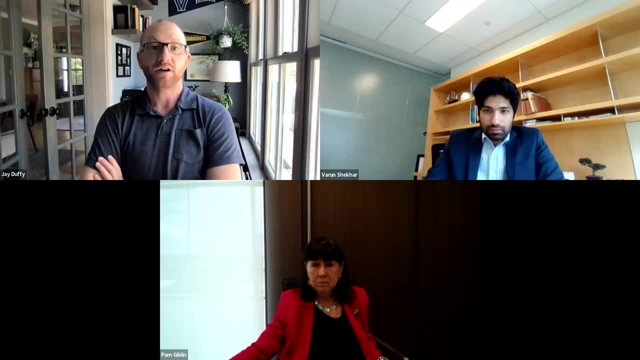 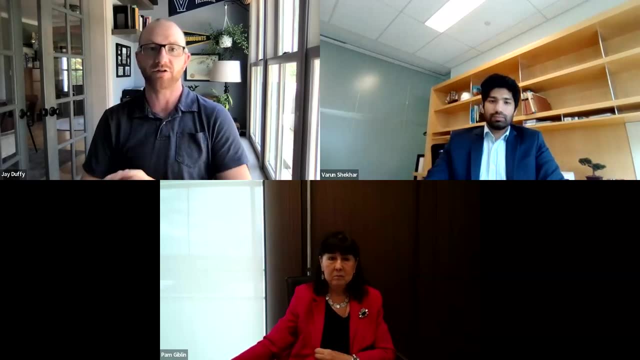 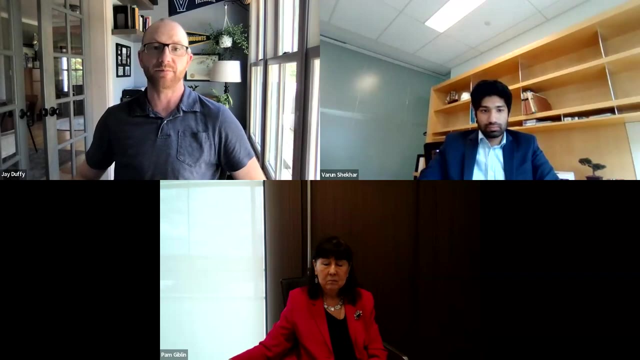 There are a lot of provisions in the under the safe drinking water act that ensure that when, when Co 2 is sequestered underground, that it's done so safely. So there is a lot of there's that, and then there for for any emissions from those wells. 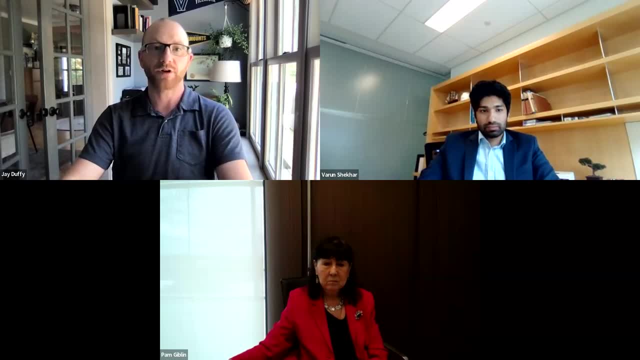 There is a portion of the Clean Air Act, The greenhouse gas reporting rule, that has monitoring and reporting and verification requirements to ensure that that that the Co 2 that's captured is is is not leaking from the sequestration sites. Great, Since, as you well know, Co. 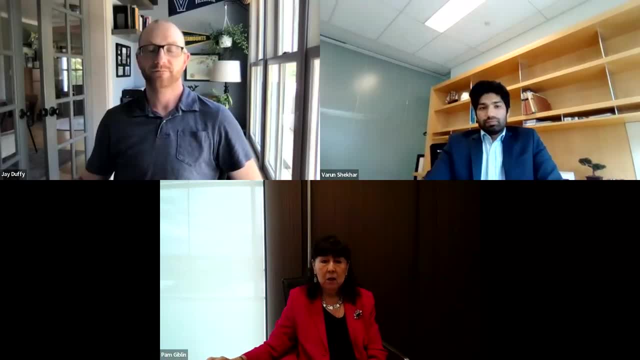 2 is only one of the greenhouse gas gases. Would you comment on what the future is, especially for methane? Everybody recognizes it's vastly more potent than Co 2 in terms of of climate. Yeah, that's some of the other ghgs also, right there's. there's also an effort right now to regulate Hfcs, which are which are very potent as well. 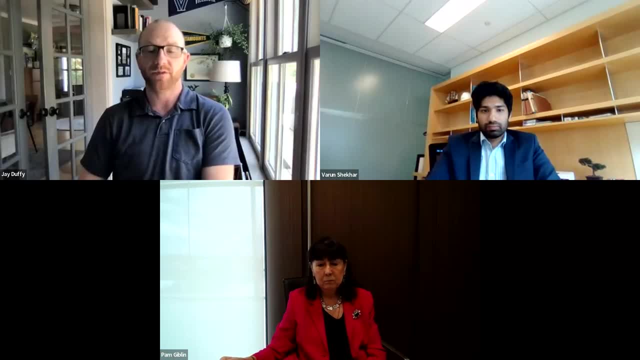 But this EPA is doing a great job of oil and gas methane emissions associated with the fracking and compressors and pipelines And I think in order for For gas to have any sort of- you know- bridge fuel properties in in the power sector, it needs to. 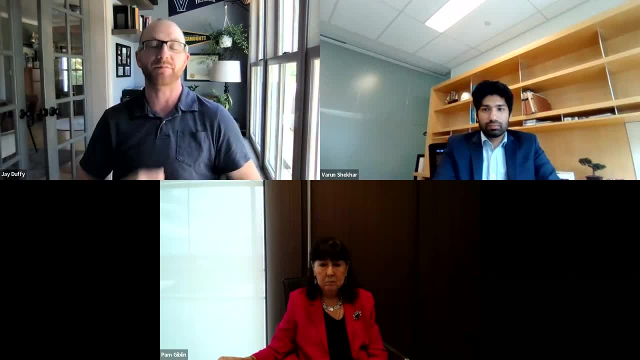 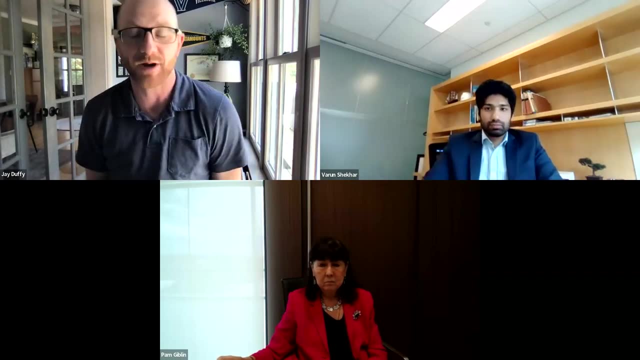 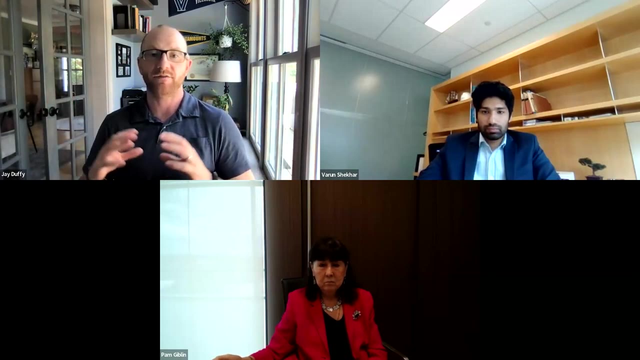 It needs to be upstream. emissions need to be cleaned up, or or it doesn't make much sense to burn it at a power plant If it's just leaking and causing greenhouse gas climate problems elsewhere. So these full the. the one of the issues with the Clean Air Act is it doesn't have a lot of wiggle room for life cycle emissions. 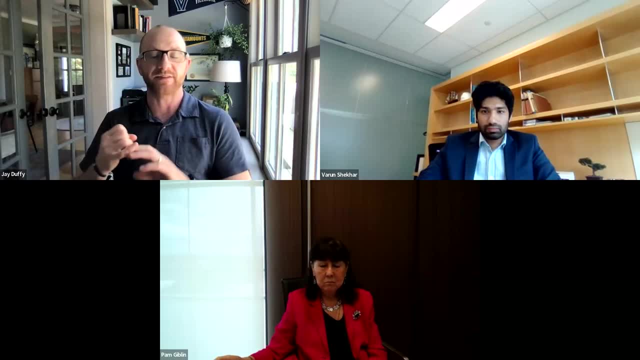 It really regulates, kind of, the emissions at the sources, at the, at the vehicle, at the power plant, at the, at the well, whatever it is, whatever that point source is. And so we have this issue with biomass. you know, biomass increases emissions at the stack. 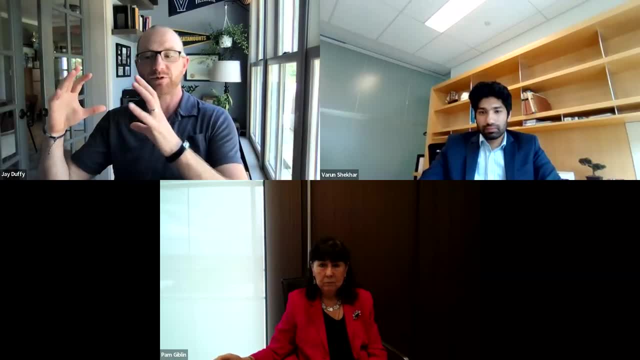 And so that is all that is kind of seen from the from the Clean Air Acts perspective. Hydrogen right: hydrogen reduces emissions at power plant stacks, But there's a lot of emissions associated with generating hydrogen Right. So I do think that they're. you know the Clean Air Act can do a lot, but there are. it was very much focused on how do we clean up the emissions from particular sources. 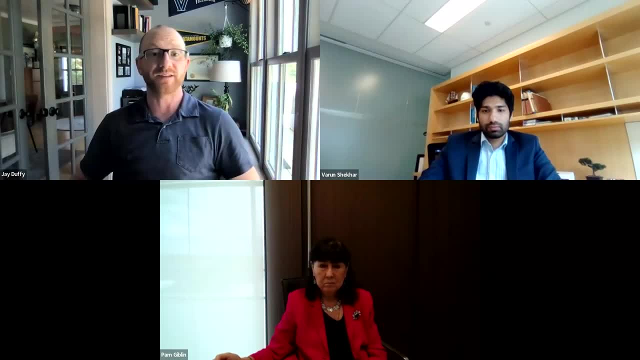 And and now we're looking at a lot of different fuels and things like that. You know, maybe it will be able to to regulate those with with some more creative thinking, But that those life cycle emissions can be tough. Well, I know there hasn't been the stomach to try to amend the Clean Air Act in any significant way. 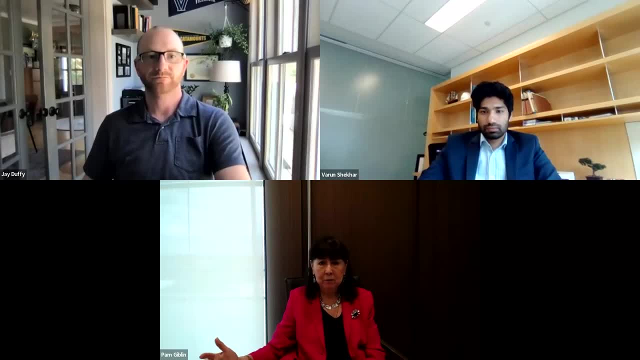 Right, People are sort of afraid of what you asked for, And so I think that it probably will not be amended, But I would like each of you to give me a prognostication. One year from now, what do you think would be the major change or addition to what we're doing to regulate either conventional pollutants or GHGs? 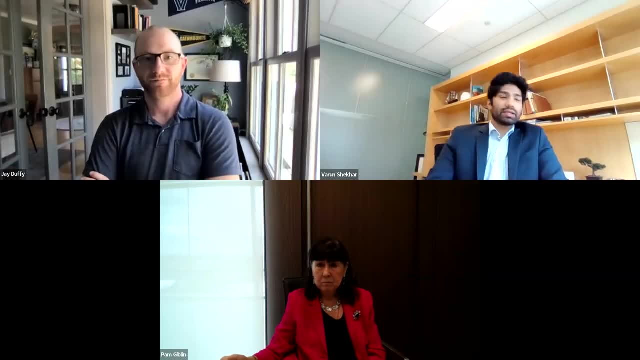 I guess I'll go first. I think the big one is- I think you hit on it, Pam- is revision to the next to include a green greenhouse gases of some sort- Carbon dioxide or something, And I think that's going to be one of the big one. 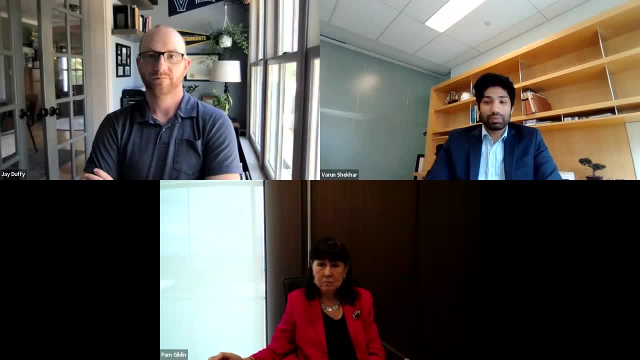 It's going to be a. it's going to have a lot of shock waves associated with it because, as you mentioned, Pam, those, those criteria- pollutants- have been the same since their outset, at the from the outset. So that's going to be something. I think that's I. 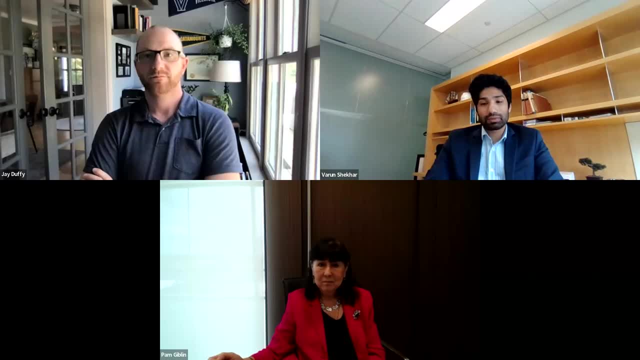 It would not surprise me if- And I think that's where we're going Next with the next big thing in the Clean Air Act- There's there's definitely going to be all kinds of litigation over that, And you know, the thing to note with the Clean Air Act is, as I think some of the issues pointed out by Jay reflect, there's a lot of political whiplash over it, even if the statute itself has not changed. 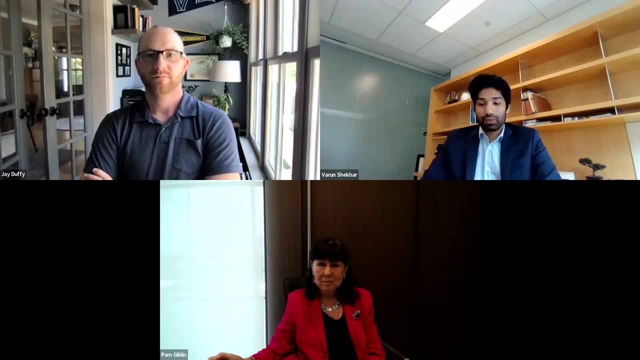 But you know, certainly, from administration to administration, you know, with with power plants and carbon dioxide emissions from them, We had clean power plan, affordable clean energy, The Biden rule. It's just. I think we're going to see something like that for the next five years or 10 years or beyond. 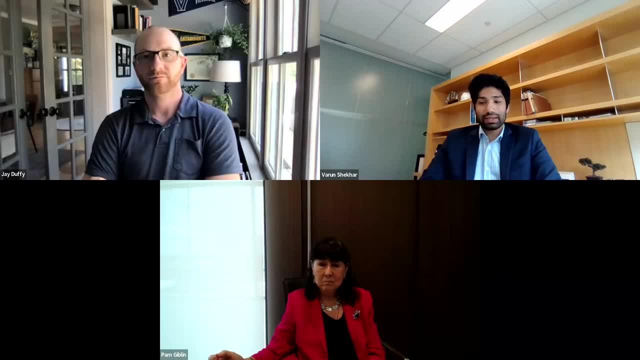 But again, if I had to hazard a guess, I think revision to the next is going to be one that really gets people's attention. How about you, Jay? What do you, what do you predict? Well, I think we're going to watch, Right? 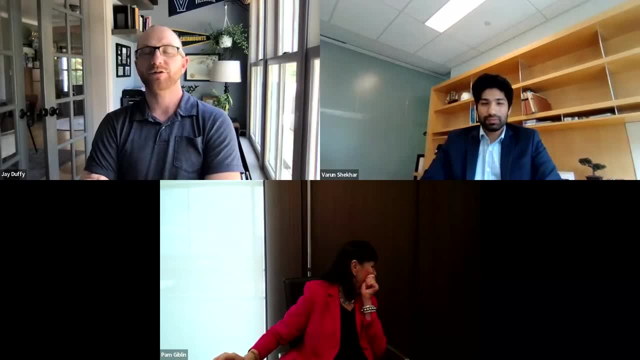 I think one of the most interesting things to me is kind of not what the impacts of the inflation reduction Act are to how we use all of these provisions. You know the Inflation Reduction Act is the biggest investment in clean energy that ever had. 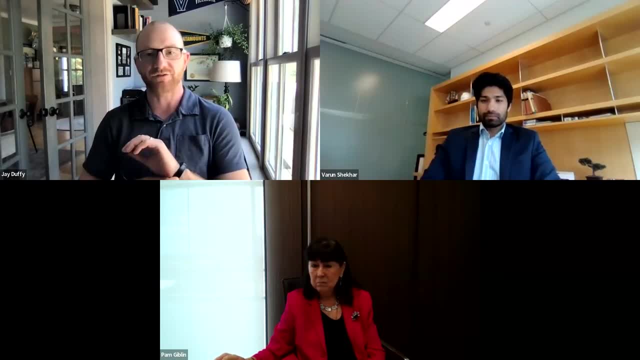 And so now we have a kind of turbo charged build out of hydrogen hubs and pipelines. There's investments for CCS, There's investments in renewable, So there's investments in EVs. So there's a lot is changing very quickly And so by 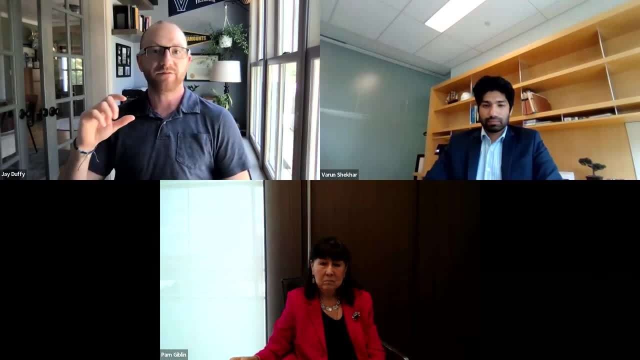 Using the statute we can leverage kind of. the Clean Air Act is is forward looking, It's technology forcing And so when we are having such a quickly advancing clean energy economy and the Clean Air Act is meant to kind of push the envelope and keep things going- 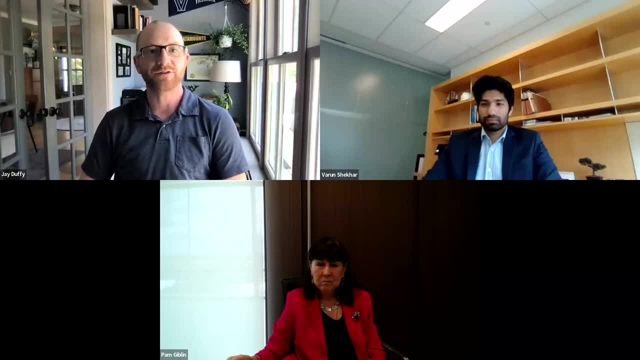 I think we can just have much stronger rules. So I'm interested in kind of how how this big influx of investment pairs with with these investments Instructions that Congress gave EPA to to push push pollution control forward. Well, my prediction of something to watch out for is the the strengthening or tightening of the secondary standards. 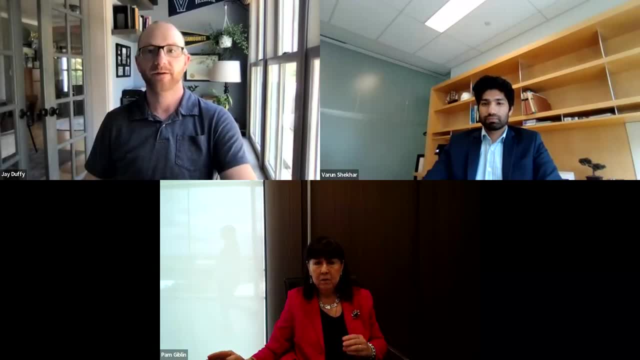 Those really haven't been touched in a long time And, as you know, the the criteria to be used by EPA are are mushier. It's, you know, protection of welfare, And so that's been, that's been Never been taken really seriously. And, as you know, there's there's a push to get EPA to really do something with secondary standards, which would give a lot more tools to EPA because, again, it wouldn't be simply constrained by the science and protection of human health. 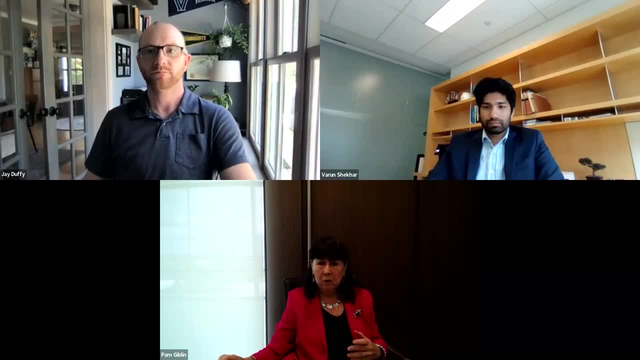 But it would be to protect welfare, with all of the attendant issues that that brings, including obviously EJ and other things. So I just think That is a tool that hasn't been used sufficiently in the past. Could they could open up a lot of you know, a lot of tightening of of operations and certainly a lot of litigation. 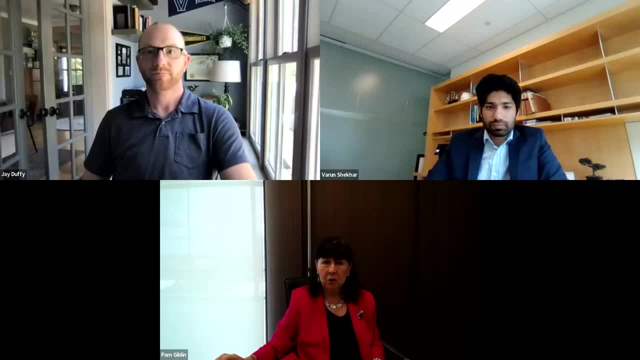 Does anybody else have any questions or any final thoughts? I mean, like I said at the beginning, I think- and I'm biased- The Clean Air Act is one of the most elastic and fabulous statutes. and air, Unlike water or a waste. 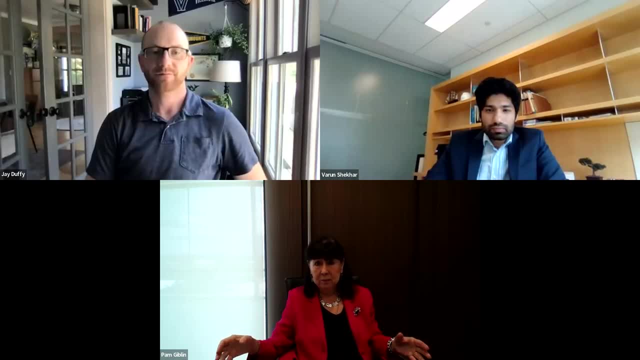 Site doesn't have boundaries in the same way. So so that's what has allowed it to be used so, so expansively. And again, I mean I, just I encourage everybody who's been listening to this webinar to dig into this great statute and to consider working in the airfield, because it's not going to go away. 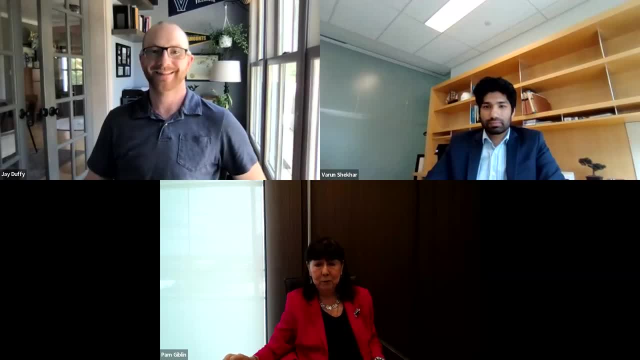 You have job security if you're doing, if you're an air lawyer, So anyway, it's true, I hope I can finally get one of these, One of these rules, across the finish line. Oh, my money's on you, So anyway. so, thanks to both of you and to Eli.